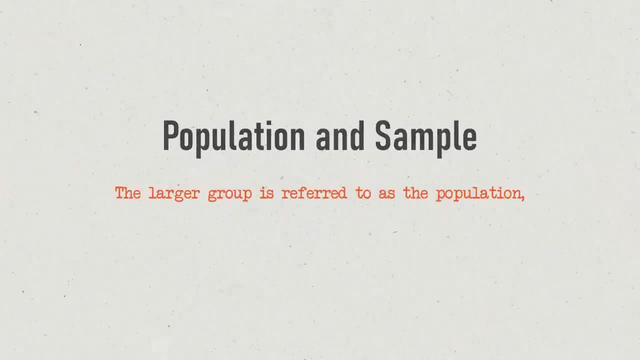 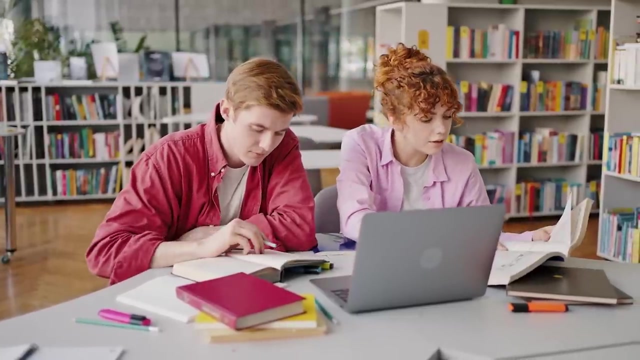 smaller subset of this group. In technical terms, the larger group is referred to as the population, and the subset- the group you will actually engage with- is called the sample. Put another way, you can look at the population as a full cake and the sample as a single slice. 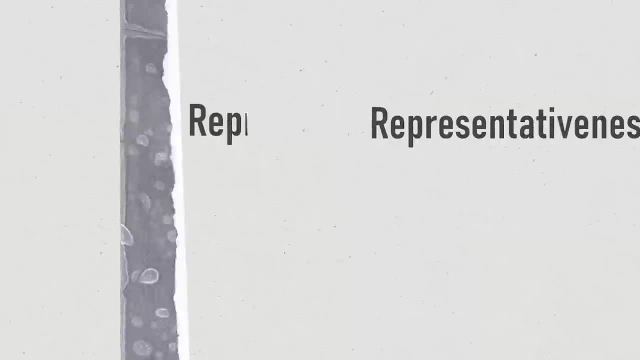 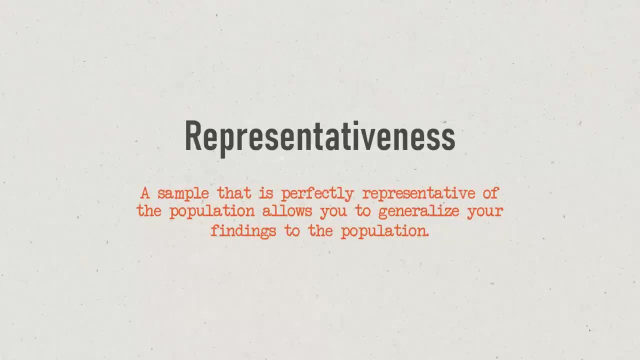 of that cake. Hmm, can you see what my mind is on? Well, in an ideal world, you would want your sample to be perfectly representative of the population, as that would allow you to generalize your sample to a larger group. So let us start with the sample. 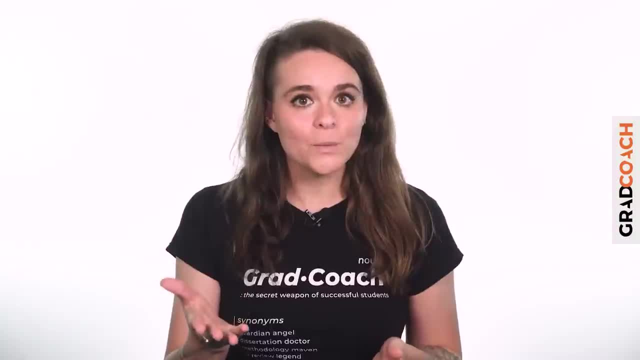 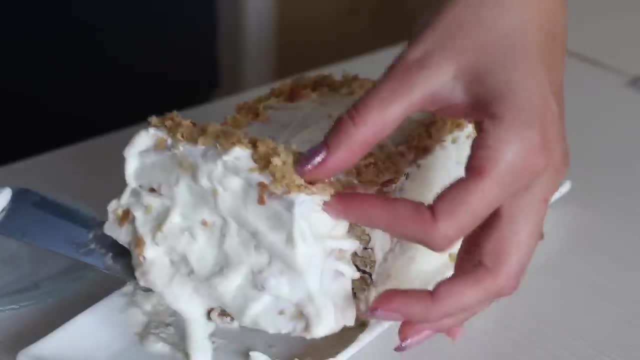 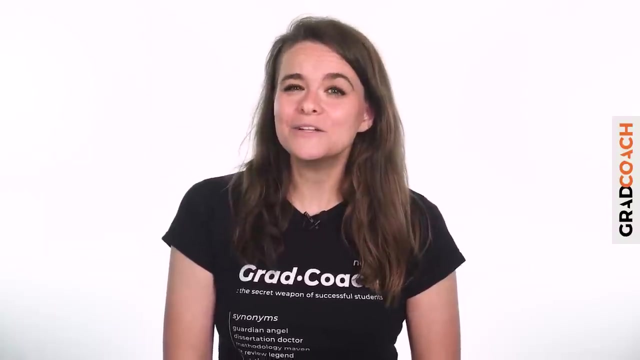 You would want to cut a perfect cross-sectional slice of that cake, such that this slice reflects every layer of the cake in exact proportion. Unfortunately, achieving a truly representative sample is a little trickier than slicing a cake, as there are many practical challenges and obstacles to achieving this in a real-world. 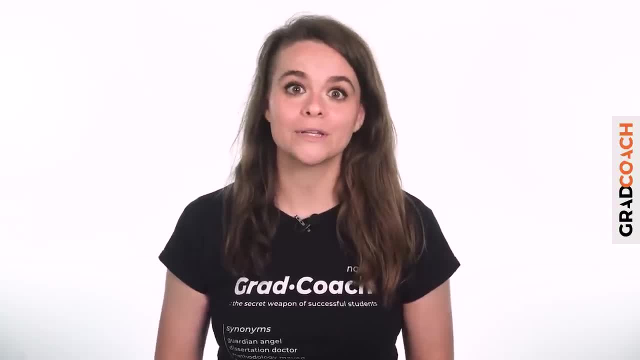 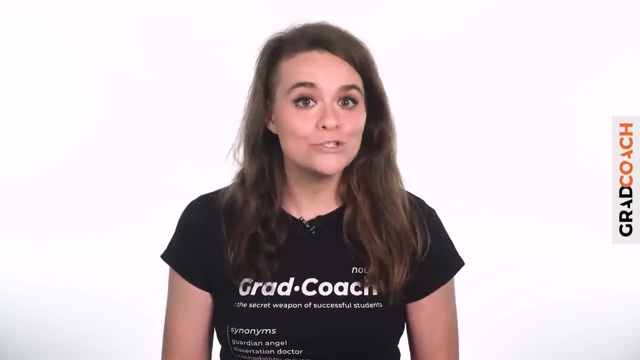 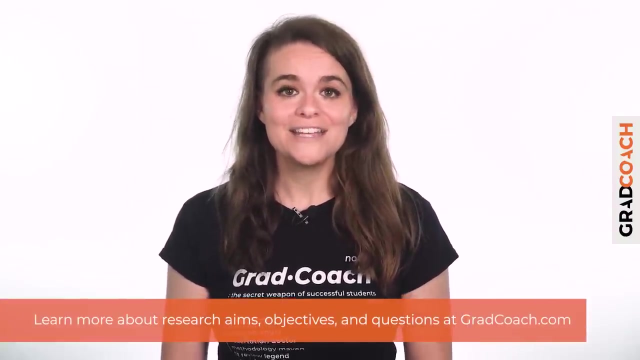 setting. Thankfully, though, you do not always need to have a perfectly representative sample, It largely depends on the specific research aims of each study, so do not stress yourself out about that just yet. By the way, if you want to learn more about research aims, objectives and questions, 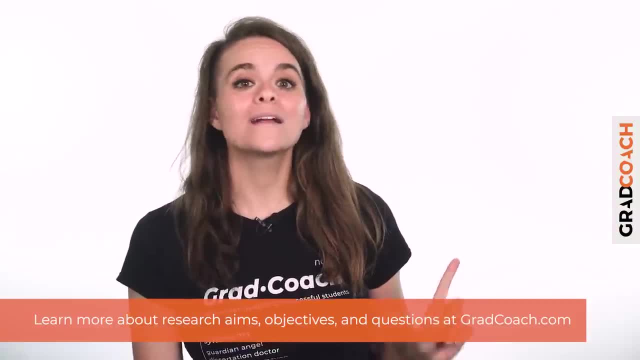 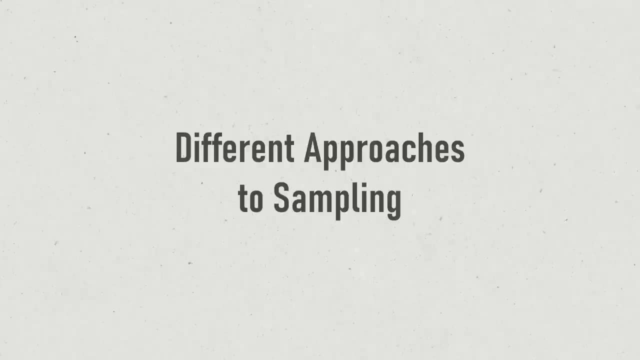 check out our explainer video up here or click on the link in the description. Alright, with the concept of sampling broadly defined, let us look at the different approaches to sampling to get a better understanding of what it all looks like in practice. 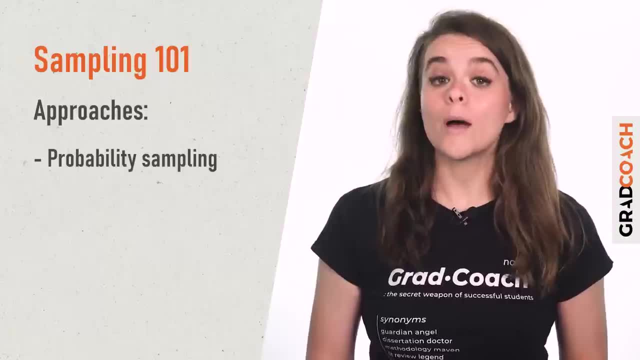 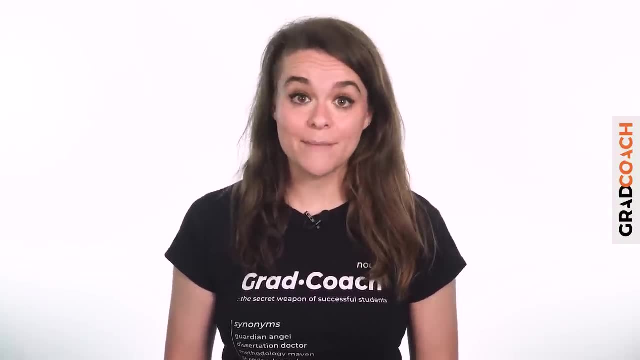 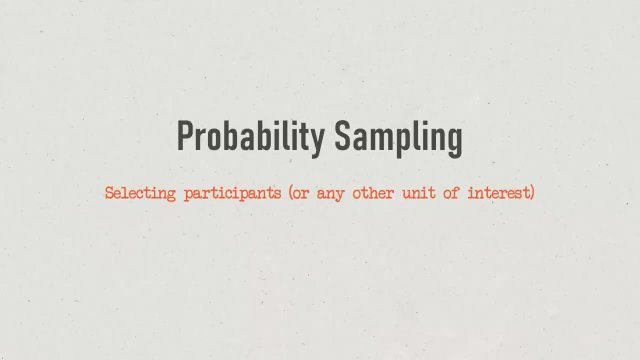 At the highest level. there are two approaches to sampling: probability sampling and non-probability sampling. Within each of these, there are a variety of sampling methods which we will explore a little later. Probability sampling involves selecting participants or any other unit of interest on a statistically random basis, which is why it is also called. 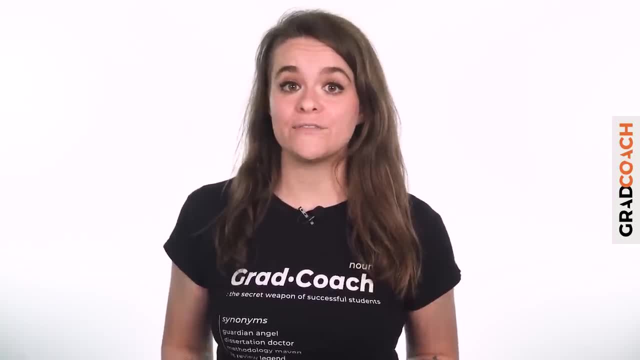 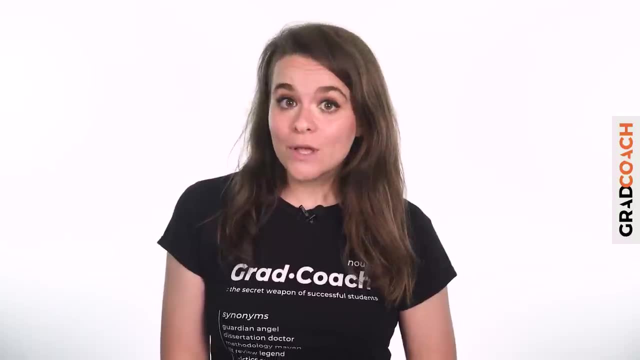 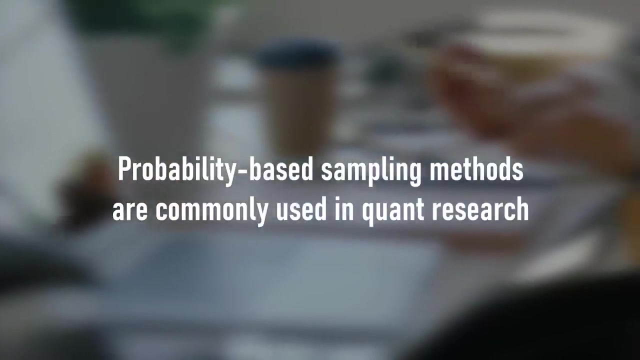 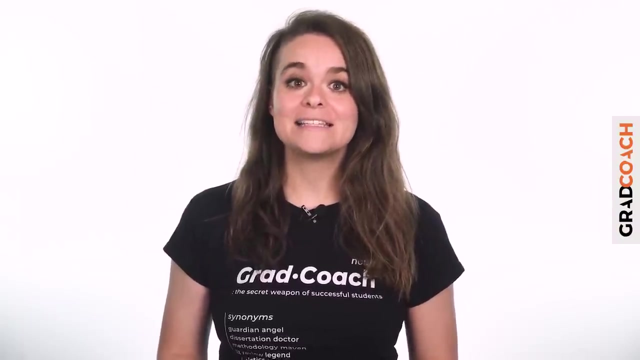 random sampling. In other words, the selection of each individual participant is based on a determined process and not the discretion of the researcher. As a result of this process-driven approach, probability sampling achieves a random sample. Probability-based sampling methods are most commonly used in quantitative research, In other words, numbers and statistics-based 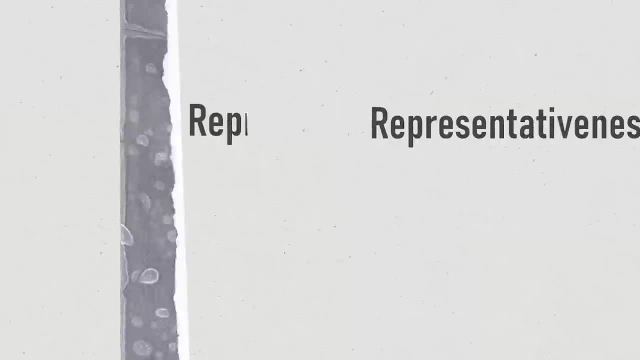 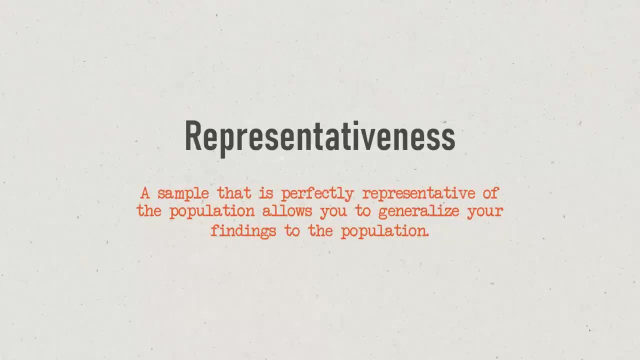 of that cake. Hmm, can you see what my mind is on? Well, in an ideal world, you would want your sample to be perfectly representative of the population, as that would allow you to generalize your sample to a larger group. So let us start with the sample. 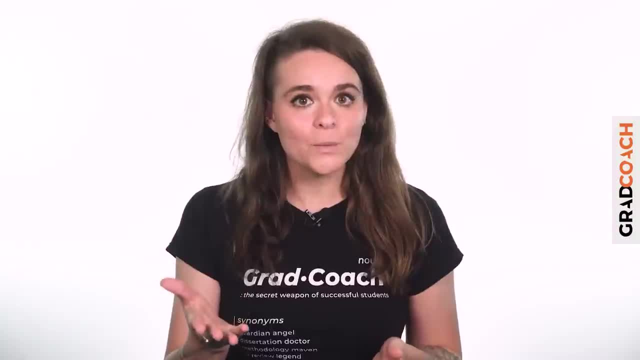 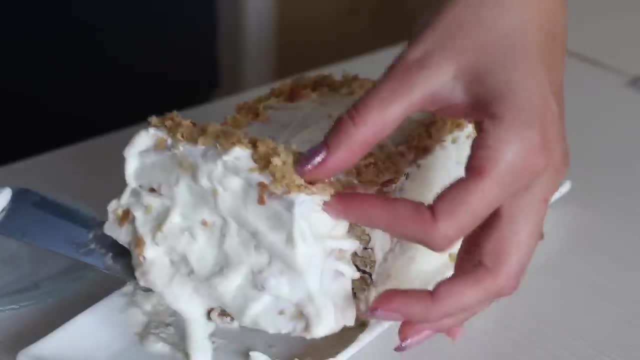 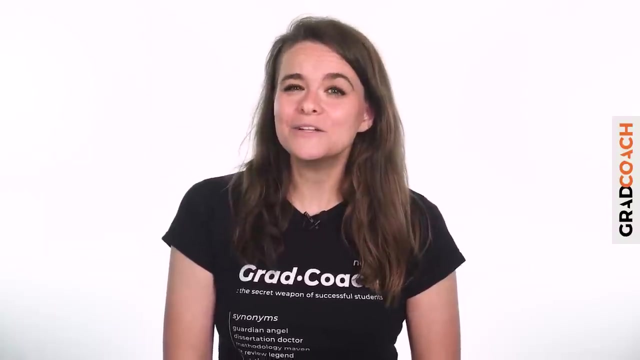 You would want to cut a perfect cross-sectional slice of that cake, such that this slice reflects every layer of the cake in exact proportion. Unfortunately, achieving a truly representative sample is a little trickier than slicing a cake, as there are many practical challenges and obstacles to achieving this in a real-world. 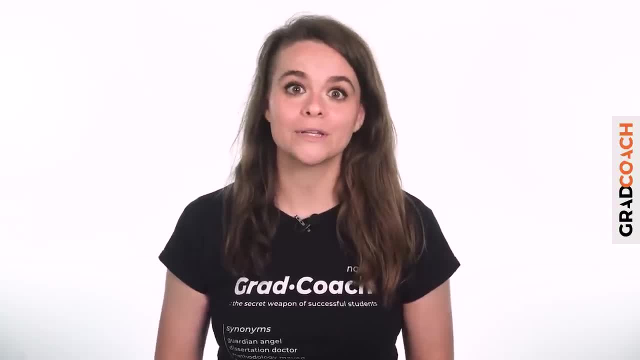 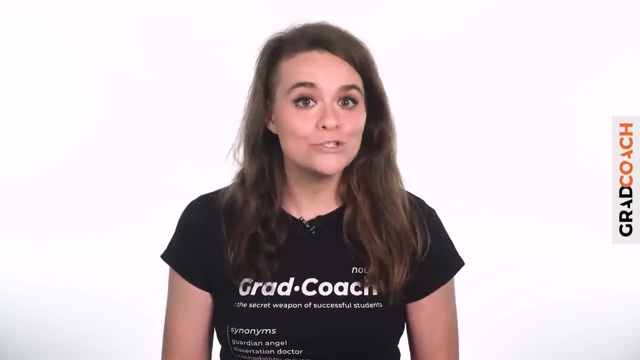 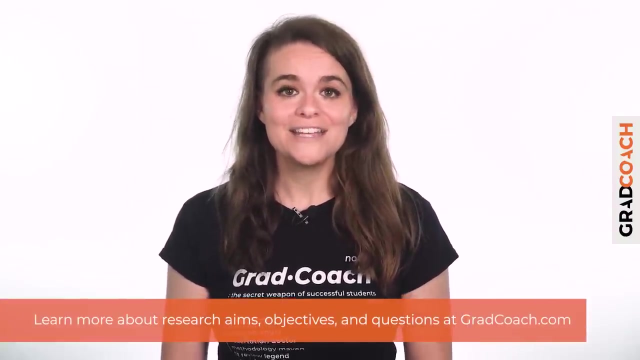 setting. Thankfully, though, you do not always need to have a perfectly representative sample, It largely depends on the specific research aims of each study, so do not stress yourself out about that just yet. By the way, if you want to learn more about research aims, objectives and questions, 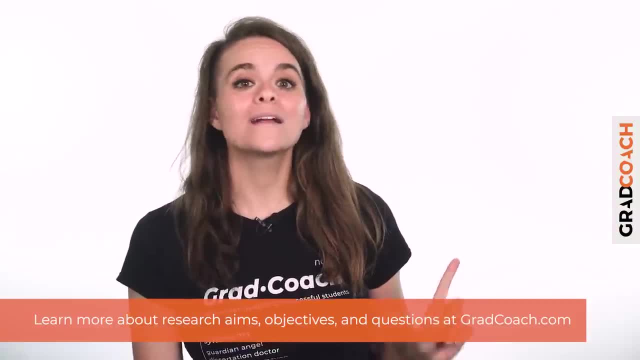 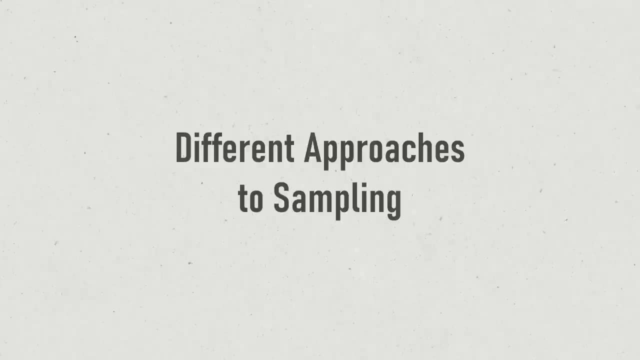 check out our explainer video up here or click on the link in the description. Alright, with the concept of sampling broadly defined, let us look at the different approaches to sampling to get a better understanding of what it all looks like in practice. 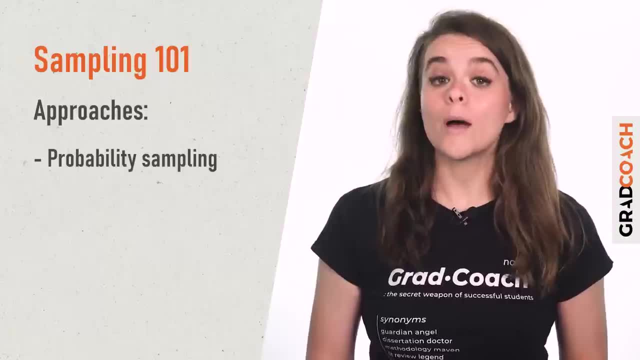 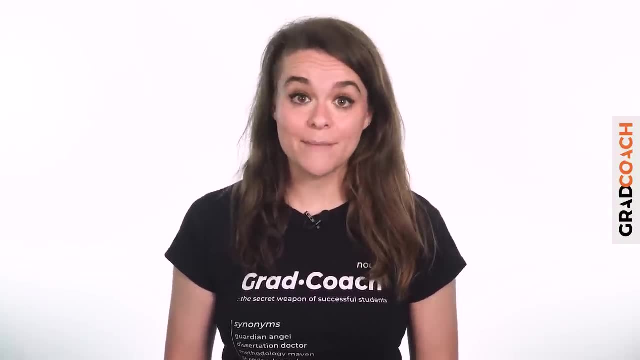 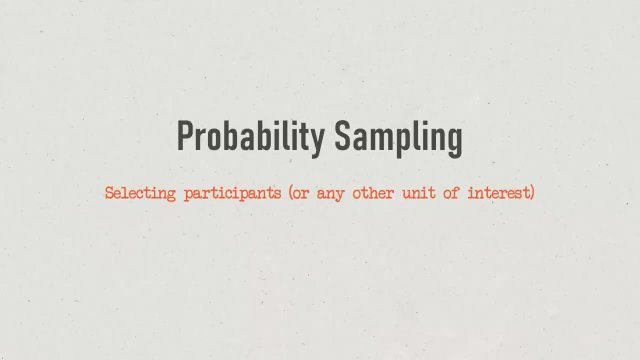 At the highest level. there are two approaches to sampling: probability sampling and non-probability sampling. Within each of these, there are a variety of sampling methods which we will explore a little later. Probability sampling involves selecting participants or any other unit of interest on a statistically random basis, which is why it is also called. 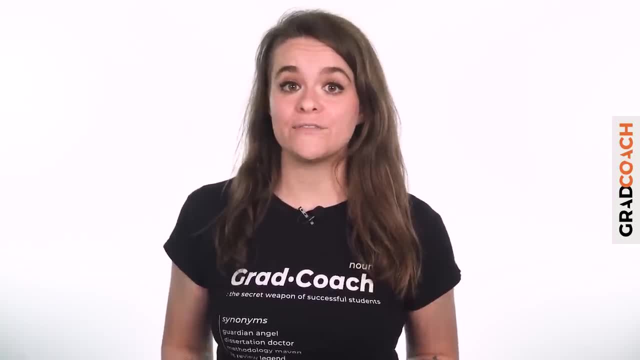 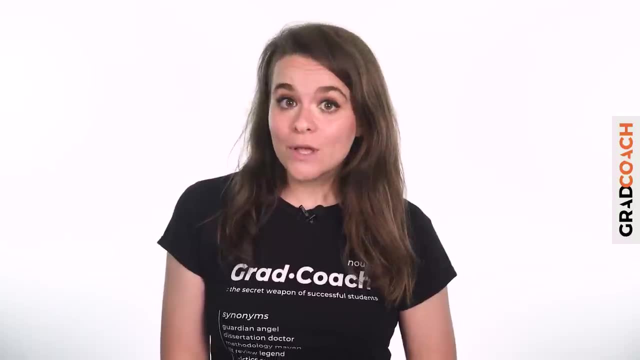 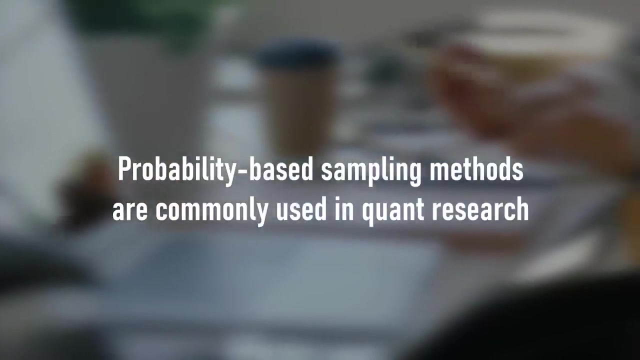 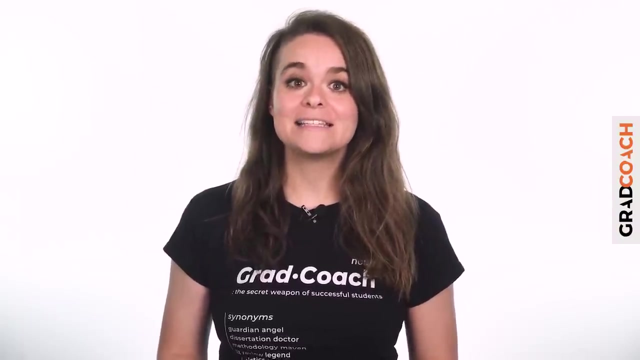 random sampling. In other words, the selection of each individual participant is based on a determined process and not the discretion of the researcher. As a result of this process-driven approach, probability sampling achieves a random sample. Probability-based sampling methods are most commonly used in quantitative research, In other words, numbers and statistics-based 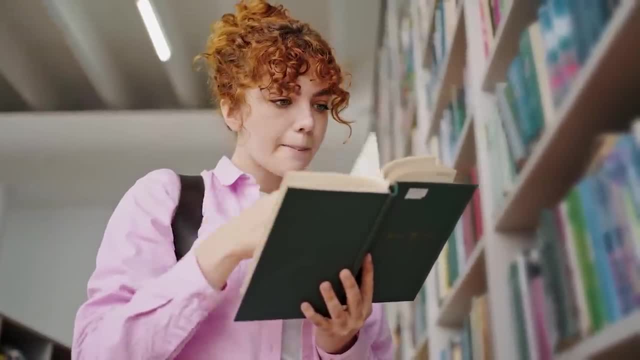 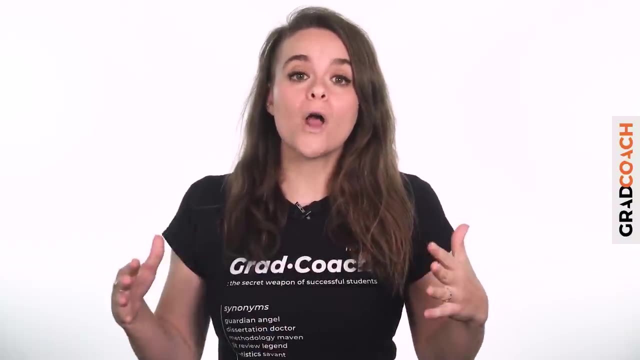 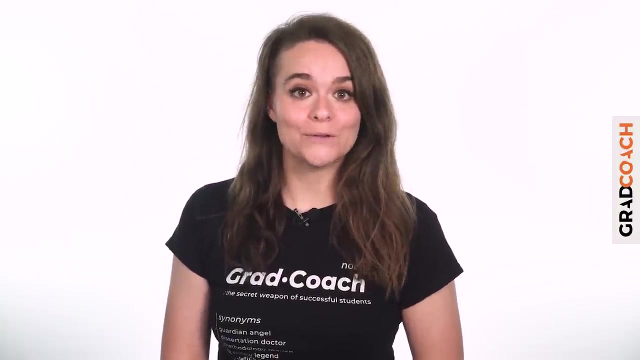 research. This is especially true for studies where the aim is to produce generalizable findings, In other words, to produce findings that allow you to draw conclusions about broader population of interest, not just the sample itself. Right now let us look at the second approach: non-probability sampling. 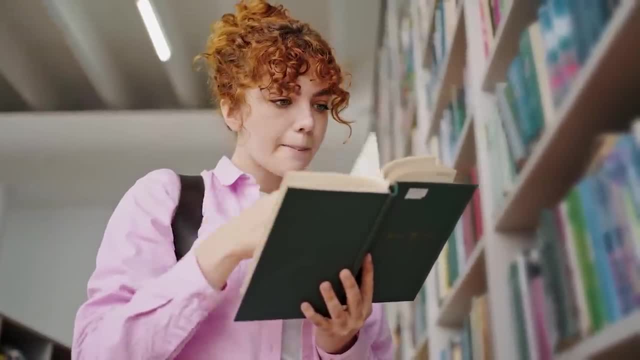 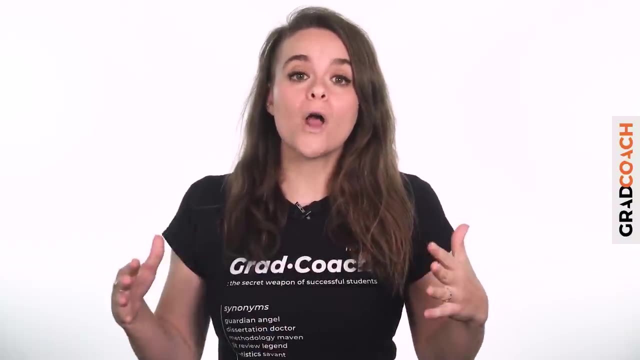 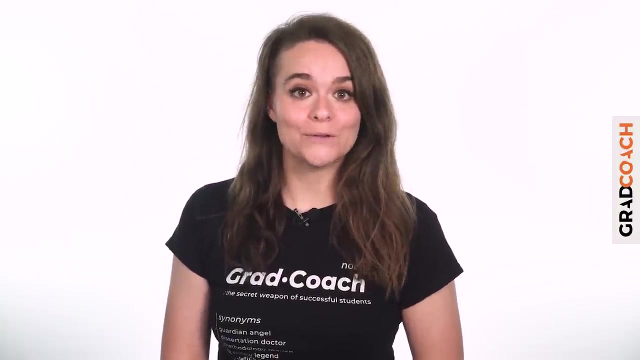 research. This is especially true for studies where the aim is to produce generalizable findings, In other words, to produce findings that allow you to draw conclusions about broader population of interest, not just the sample itself. Right now let us look at the second approach: non-probability sampling. 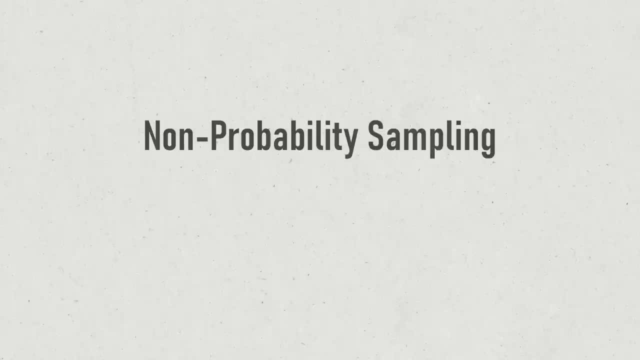 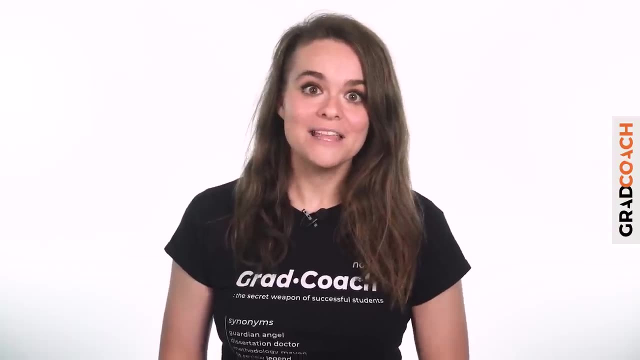 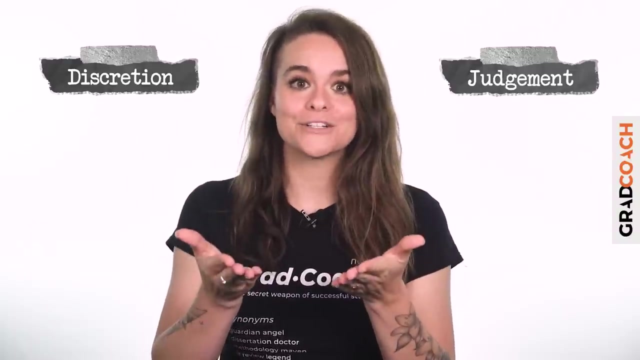 Non-probability sampling, as the name suggests, consists of sampling methods in which participant selection is not statistically random. In other words, the selection of individual participants is based on the discretion and judgment of the researcher rather than on a predetermined process. 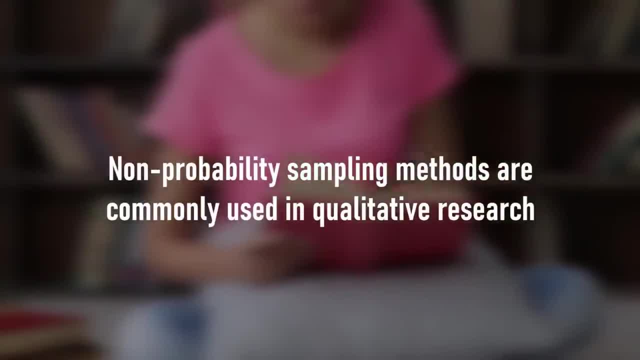 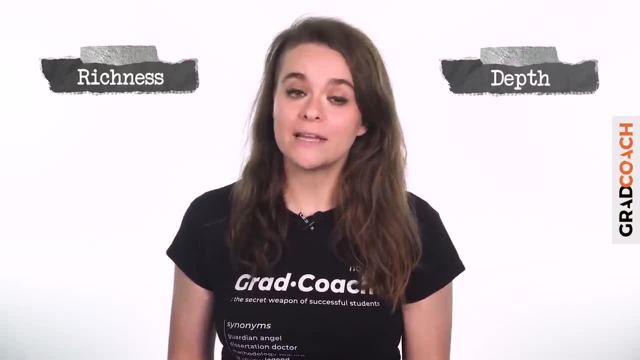 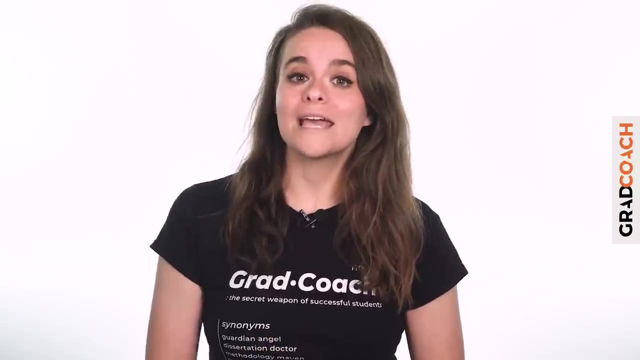 Non-probability sampling methods are commonly used in qualitative research where the richness and depth of the data are more important than the generalizability of the findings. If that all sounds a little too conceptual and fluffy, do not worry. Next we will take a look at some actual sampling methods to make it a little more tangible. 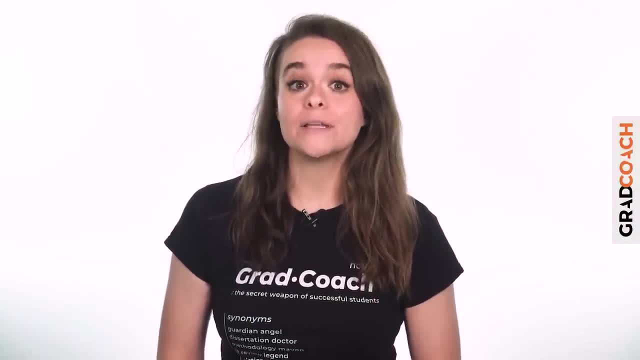 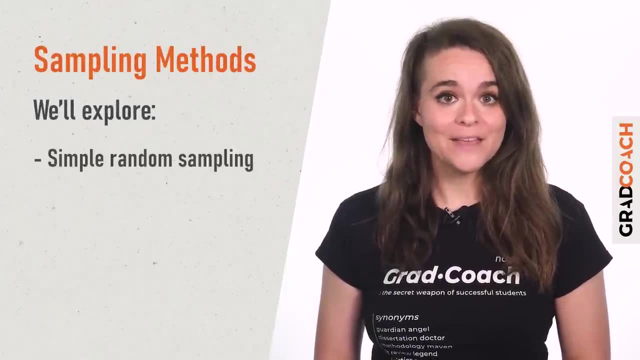 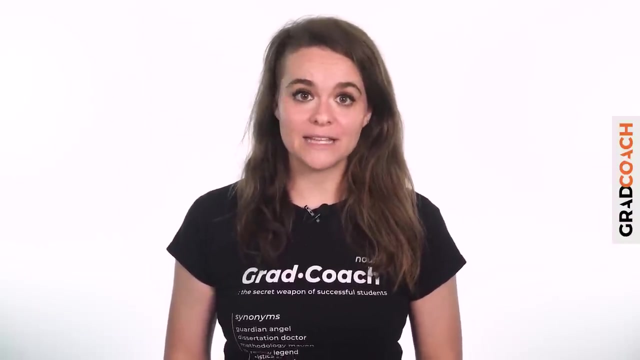 To kick things off, we will look at three popular probability-based random sampling methods. Specifically, we will explore simple random sampling, stratified random sampling and cluster sampling. Importantly, this is not a comprehensive list of all possible probability sampling methods. 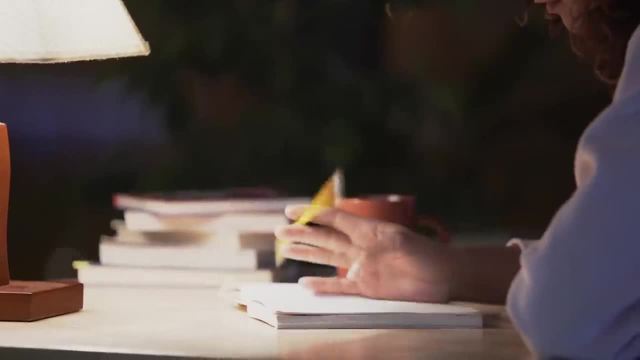 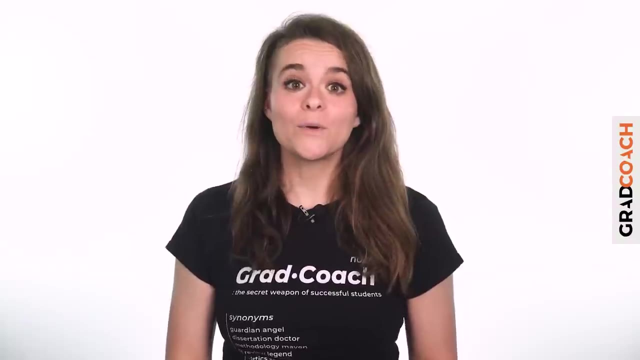 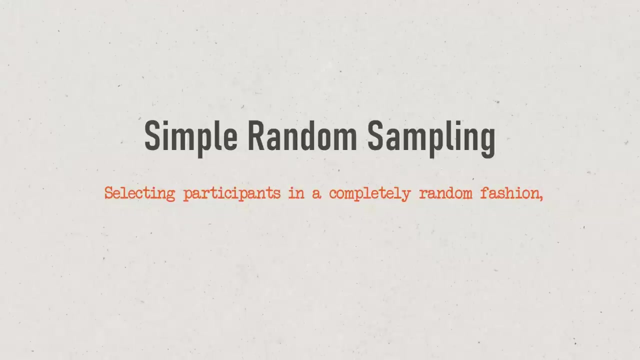 These are just the three most common ones, So if you are interested in adopting a probability-based sampling approach, be sure to explore all of the options. First up, we have simple random sampling. Simple random sampling involves selecting participants in a completely random fashion. 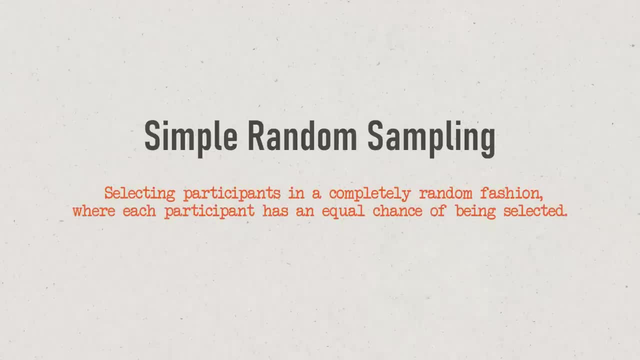 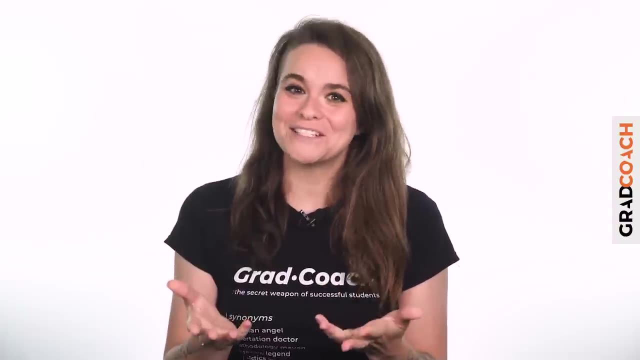 where each participant has an equal chance of being selected. Basically, this sampling method is the equivalent of pulling names out of a hat, except that you can do it digitally. For example, if you had a list of 500 people, you could use a random number. 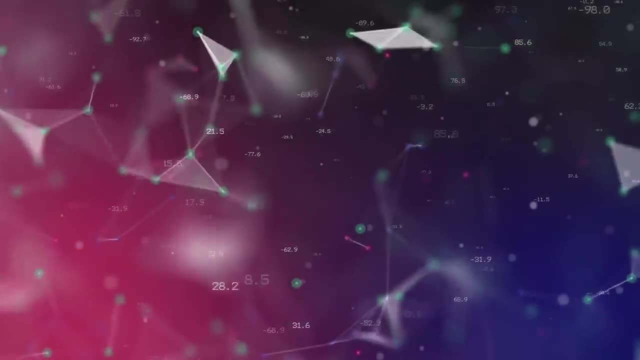 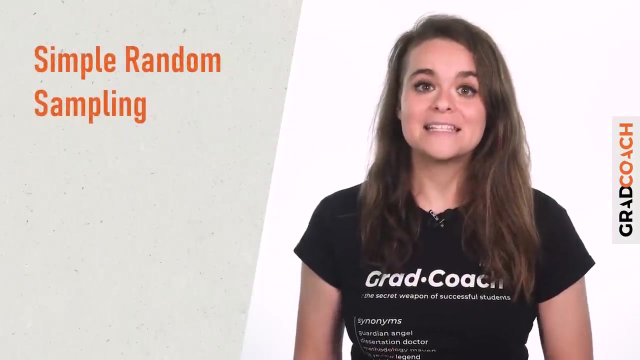 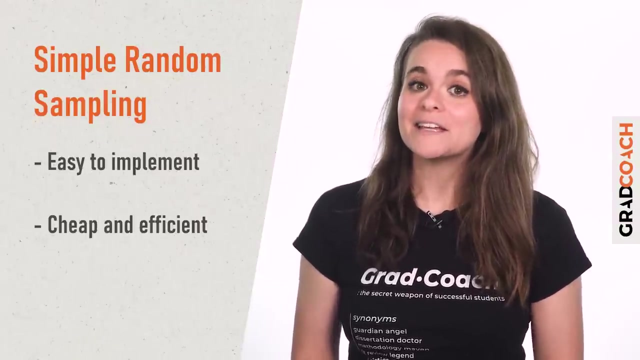 generator to draw a list of 50 numbers, each number reflecting a participant, and then use that dataset as your sample. Thanks to its simplicity, simple random sampling is easy to implement and, as a consequence, is typically quite cheap and efficient. Because the selection process is completely random, you can generalize your results fairly. 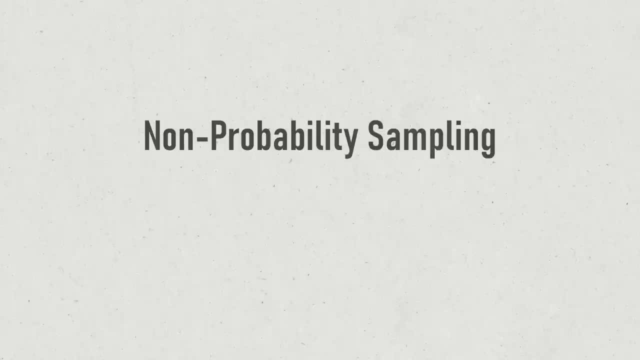 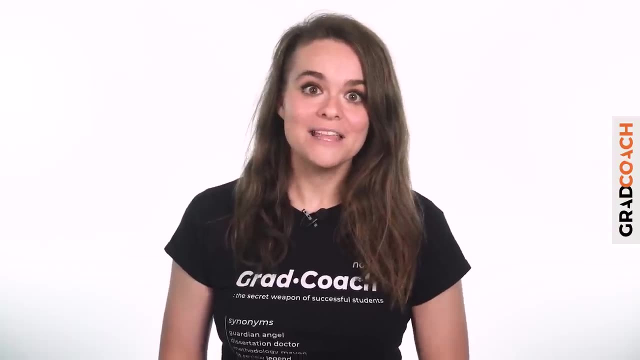 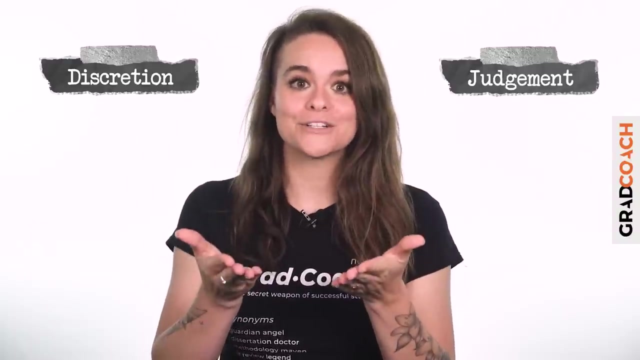 Non-probability sampling, as the name suggests, consists of sampling methods in which participant selection is not statistically random. In other words, the selection of individual participants is based on the discretion and judgment of the researcher rather than on a predetermined process. 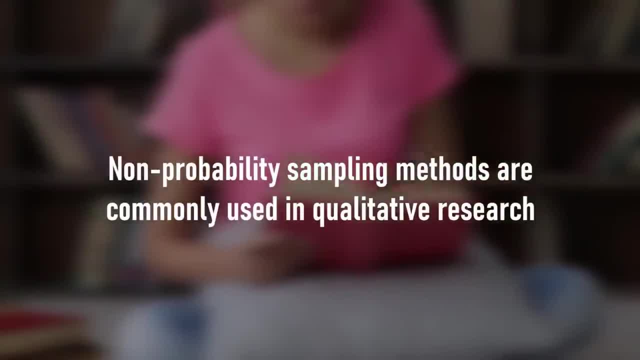 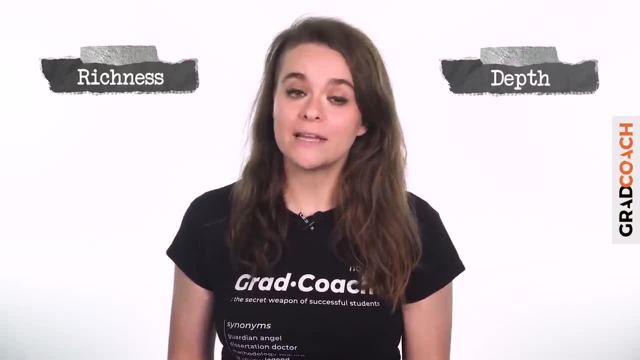 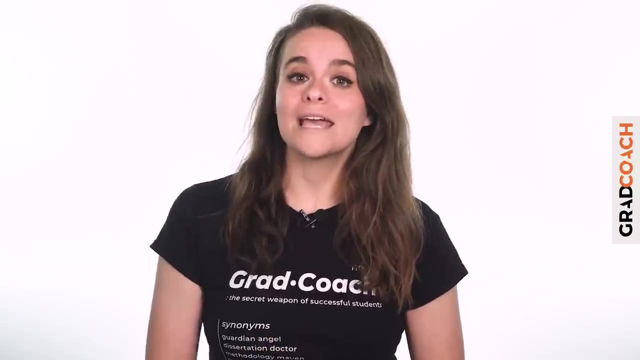 Non-probability sampling methods are commonly used in qualitative research where the richness and depth of the data are more important than the generalizability of the findings. If that all sounds a little too conceptual and fluffy, do not worry. Next we will take a look at some actual sampling methods to make it a little more tangible. 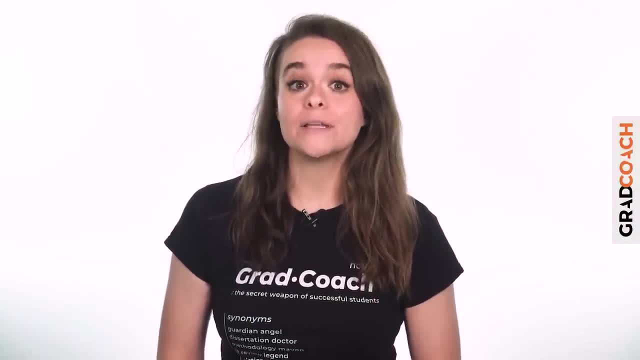 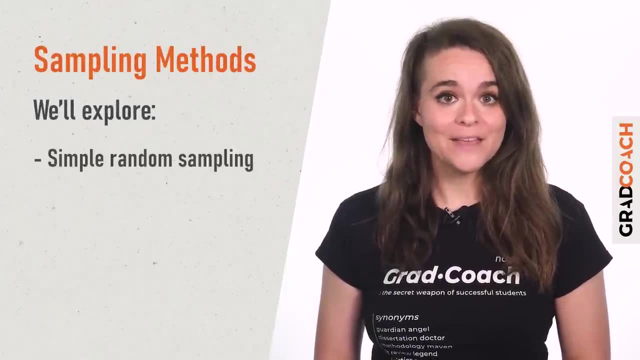 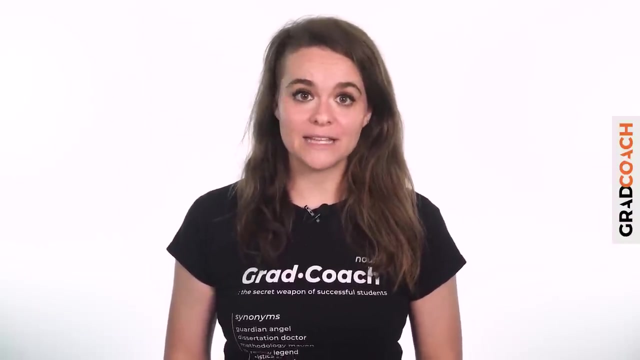 To kick things off, we will look at three popular probability-based random sampling methods. Specifically, we will explore simple random sampling, stratified random sampling and cluster sampling. Importantly, this is not a comprehensive list of all possible probability sampling methods. 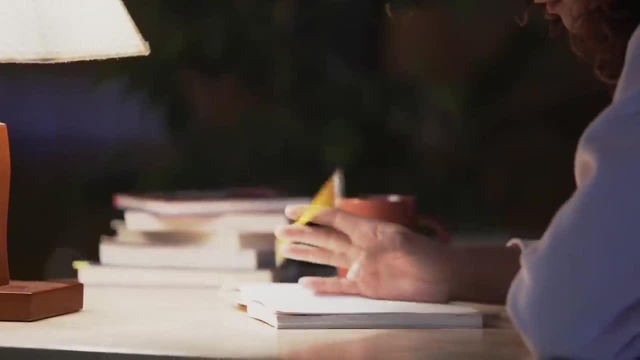 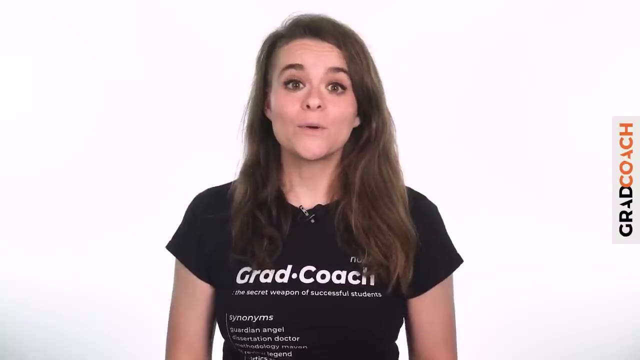 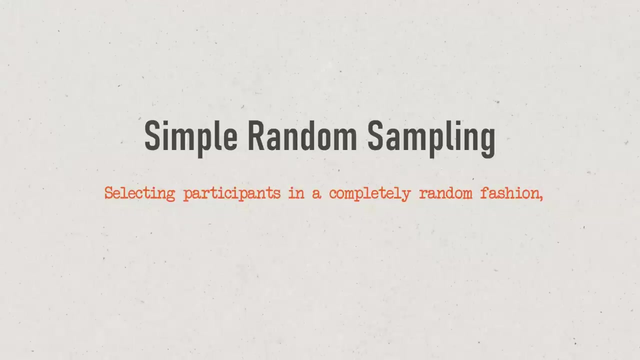 These are just the three most common ones, So if you are interested in adopting a probability-based sampling approach, be sure to explore all of the options. First up, we have simple random sampling. Simple random sampling involves selecting participants in a completely random. 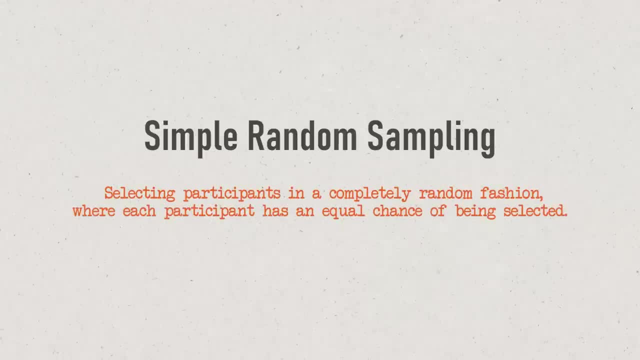 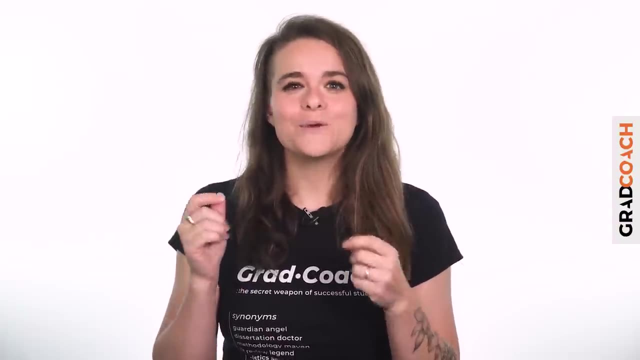 fashion where each participant has an equal chance of being selected. Basically, this sampling method is the equivalent of pulling names out of a hat, except that you can do it digitally. For example, if you had a list of 500 people, you could use a random number. 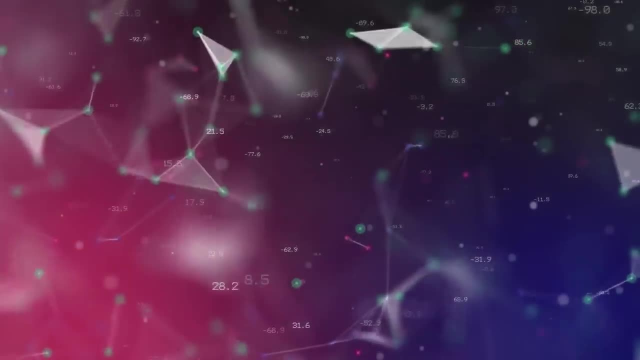 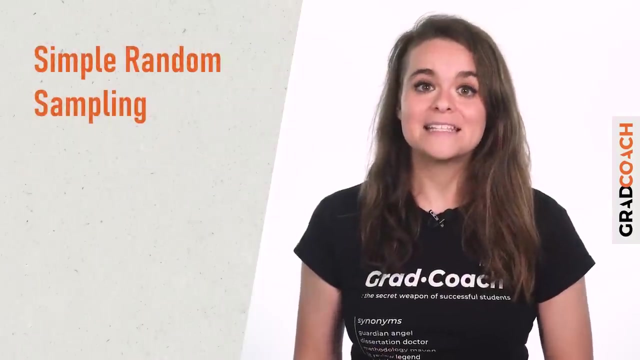 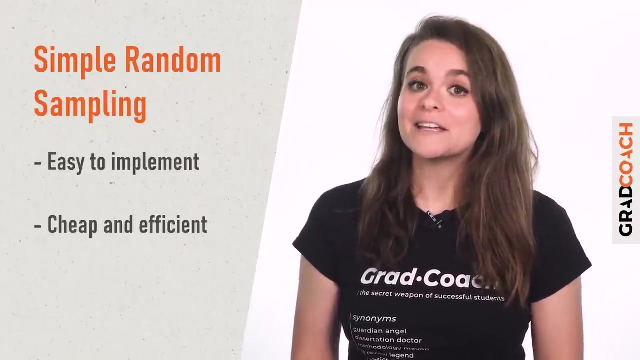 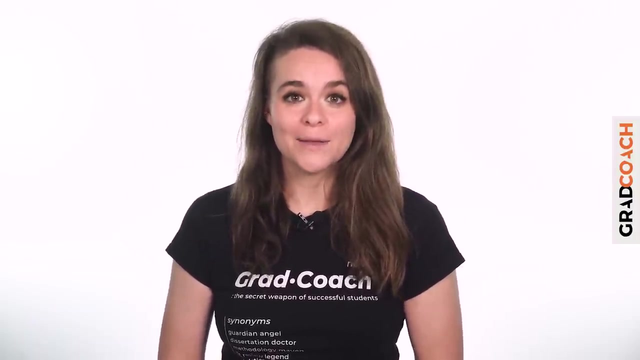 generator to draw a list of 50 numbers, each number reflecting a participant, and then use that data set as your sample. thanks to its simplicity, simple random sampling is easy to implement and, as a consequence, is typically quite cheap and efficient. because the selection process is completely random, you can generalize your results fairly reliably. however, this also 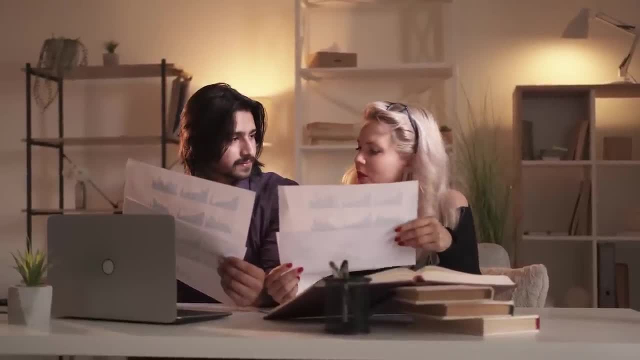 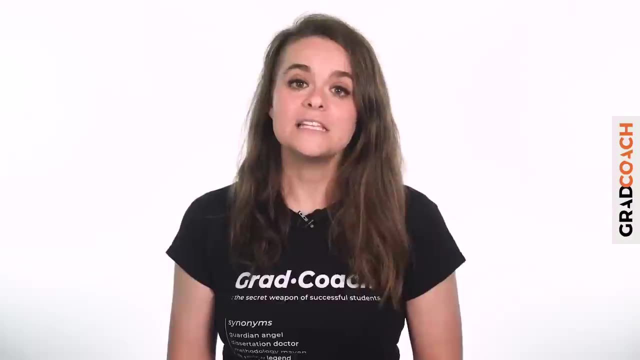 means it can hide the impact of large subgroups within the data, which can result in minority subgroups having little representation in the results, if any at all. this may or may not be an issue, depending on what you are trying to achieve, so it is important to always consider. 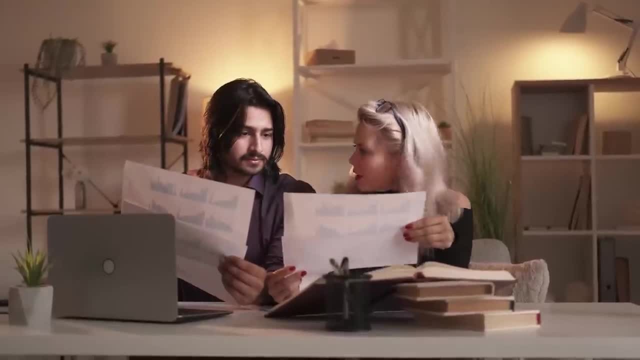 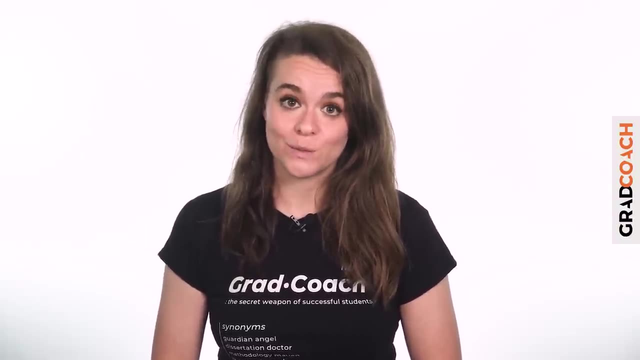 reliably. However, this also means it can hide the impact of large subgroups within the data, which can result in minority subgroups having little representation in the results, if any at all. This may or may not be an issue, depending on what you are trying to achieve. 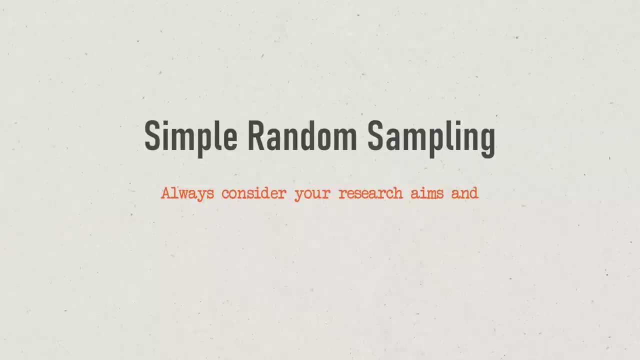 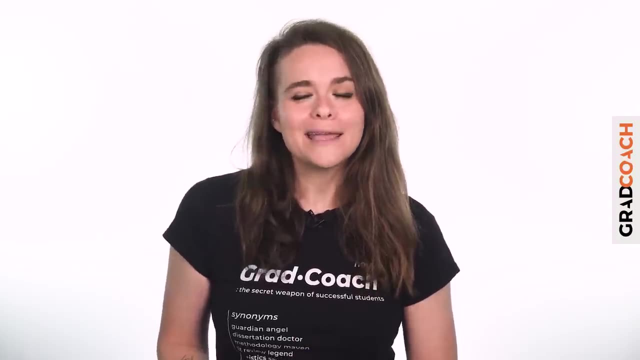 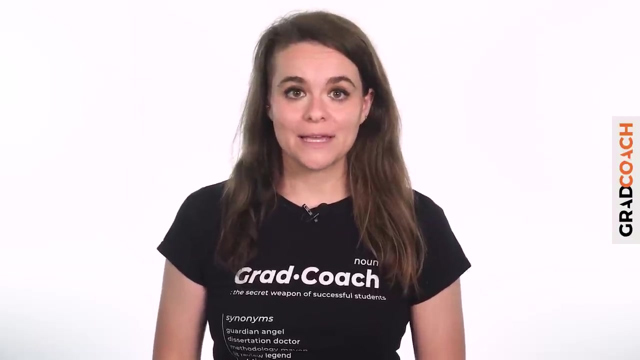 so it is important to always consider your research aims and research questions when you are deciding which sampling method to use. We will explore that a little later in more detail. Next in line, we have stratified random sampling. Stratified random sampling is similar to the previous method. 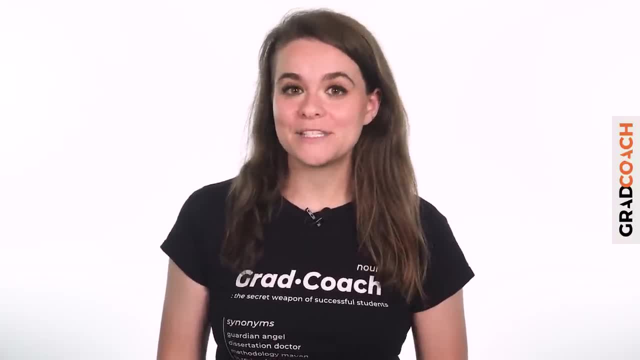 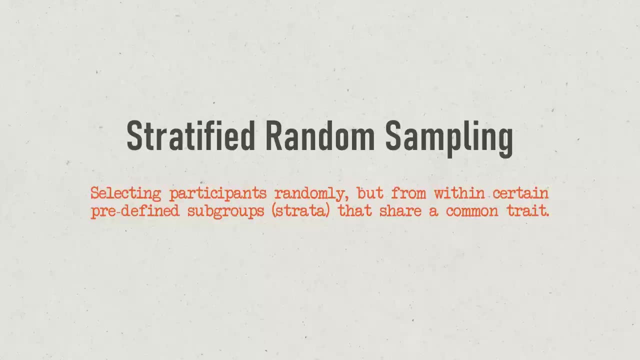 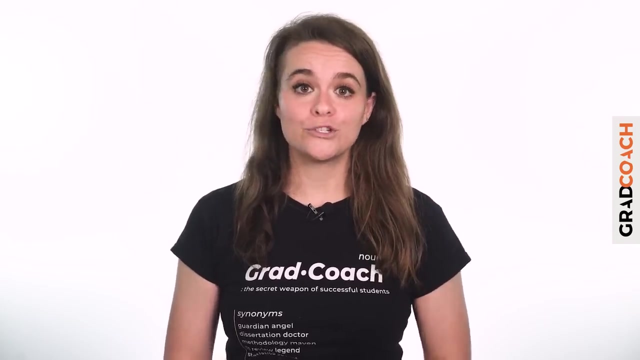 but it kicks things up a notch. As the name suggests, stratified sampling involves selecting participants randomly, but from within certain predefined subgroups that share a common trait. These are called strata. For example, you could stratify a given population based on gender, ethnicity or level of education. 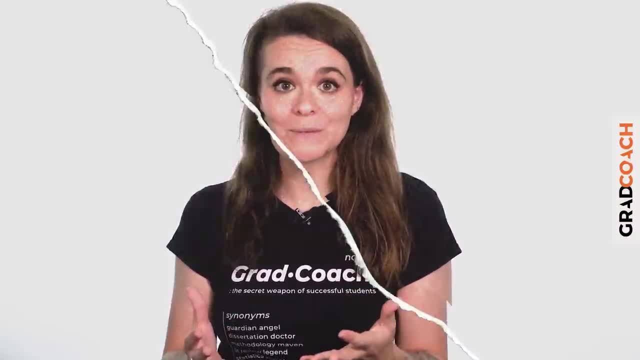 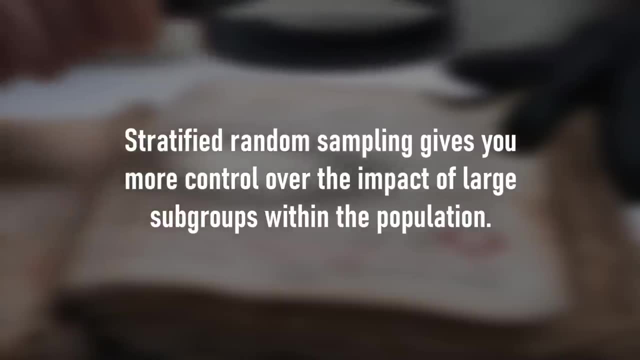 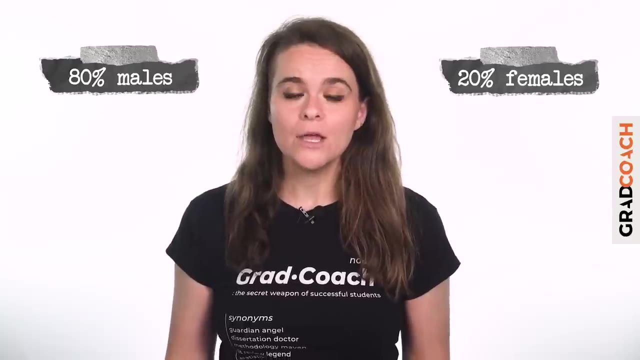 and then select participants randomly from each group. The benefit of this sampling method is that it gives you more control over the impact of large subgroups, large strata within the population. For example, if a population comprises 80% males and 20% females. 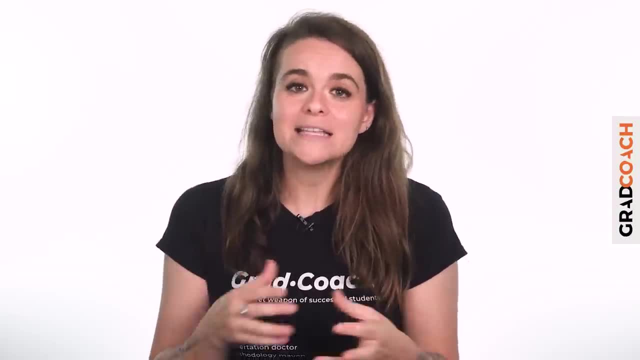 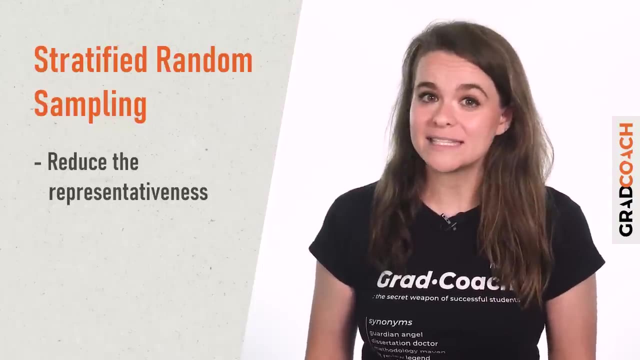 you may want to balance this skew out by selecting an equal number of male and female participants. This would, of course, reduce the representativeness of the sample, but it would allow you to identify differences between subgroups. So, once again, you need to. 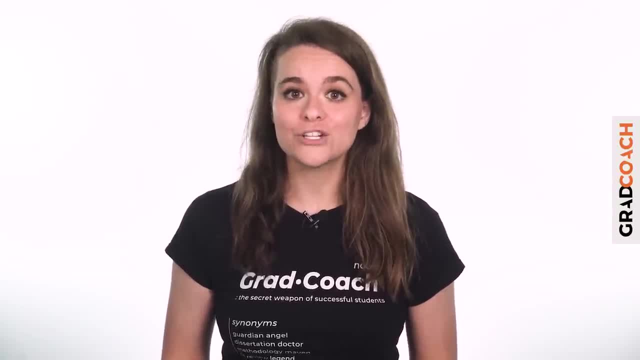 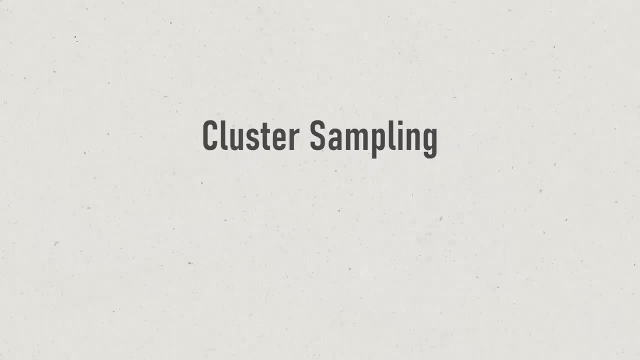 think about your research aims, as well as the nature of the population that you are interested in, so that you can make the right sampling choice. Next up, let us look at cluster sampling. As the name suggests, this sampling method involves sampling from naturally occurring 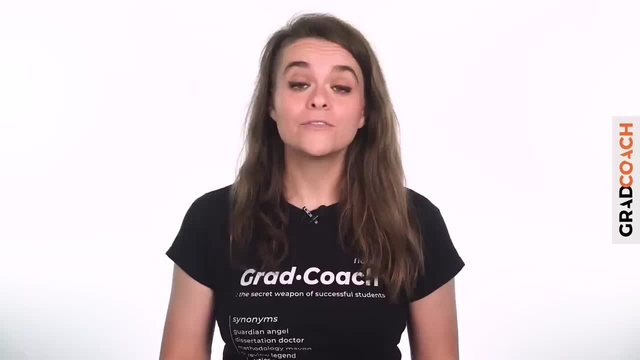 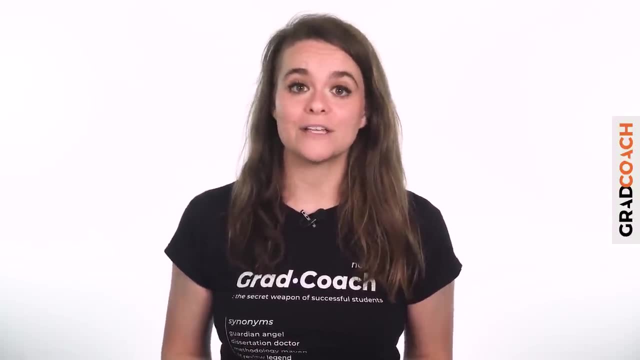 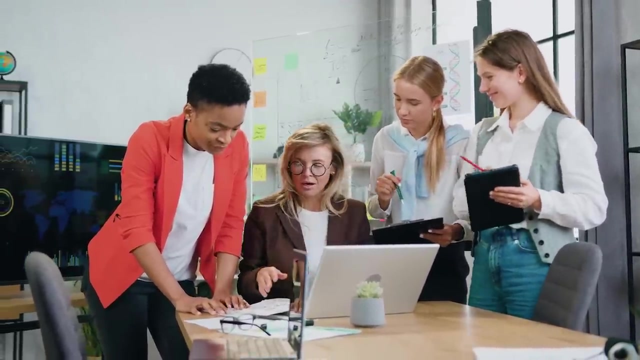 mutually exclusive clusters within a population, For example, area codes within a city or cities within a country. Once the clusters are defined, a set of clusters are randomly selected and then a set of participants are randomly selected from each cluster. Now your purpose of sampling the answers is to see if your sample is in the right order within the population. 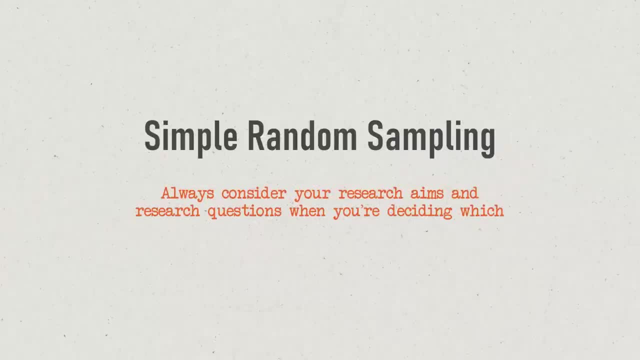 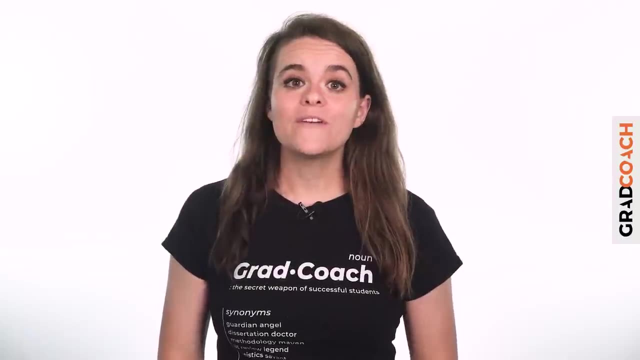 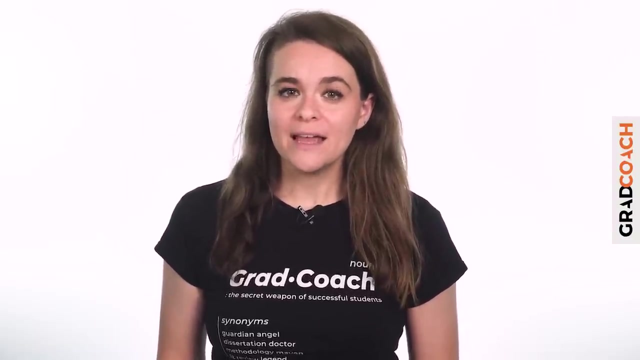 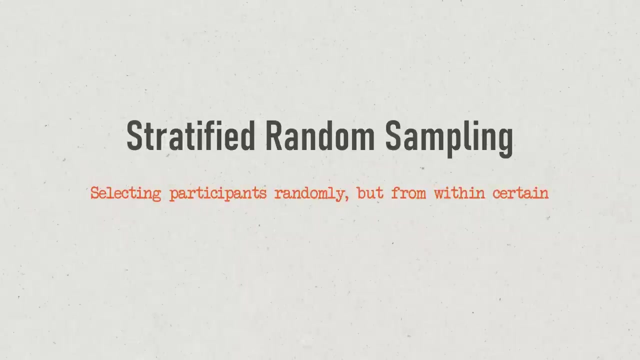 your research aims and research questions when you are deciding which sampling method to use. we will explore that a little later in more detail. next in line we have got stratified random sampling. stratified random sampling is similar to the previous method, but it kicks things up a notch. as the name suggests, stratified sampling involves selecting participants. 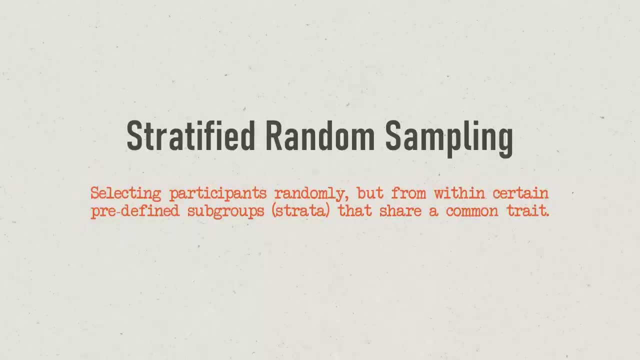 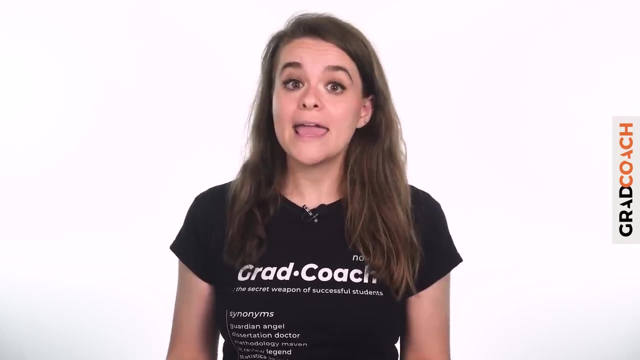 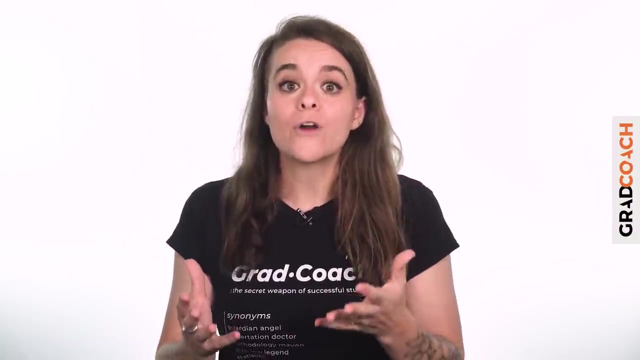 randomly, but from within certain predefined subgroups that share a common trait. these are called strata. for example, you could stratify a given population based on gender, ethnicity or level of education and then select participants randomly from each group. the benefit of this sampling method is that it gives you more control over the impact of random sampling. 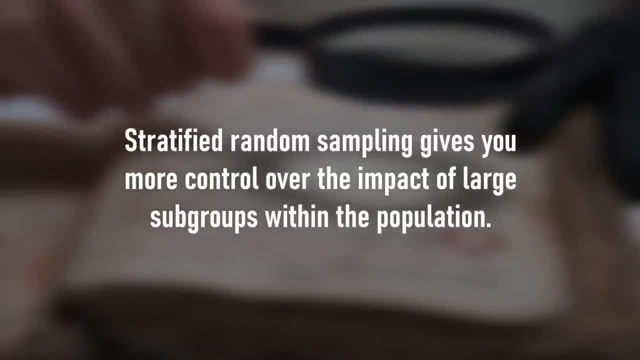 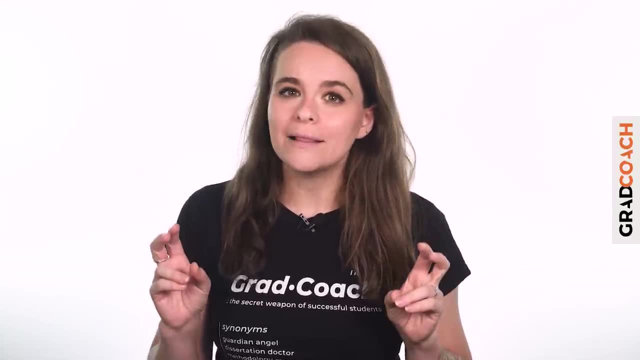 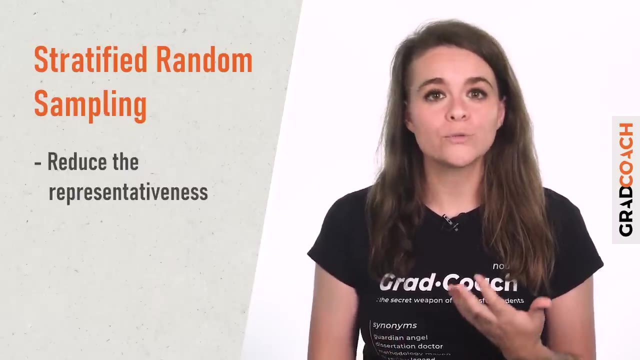 of large subgroups, large strata within the population. for example, if a population comprises 80 males and 20 females, you may want to balance this skew out by selecting an equal number of male and female participants. this would, of course, reduce the representativeness of the sample, but it would allow you to identify differences between subgroups. 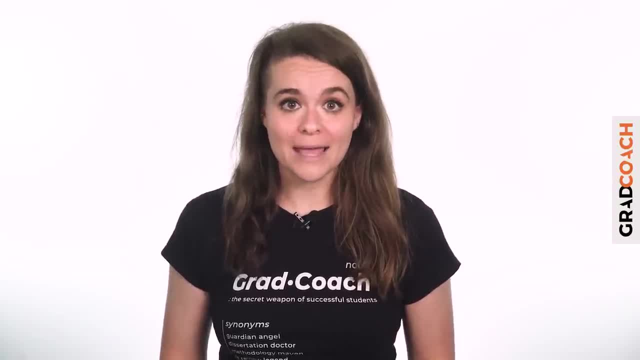 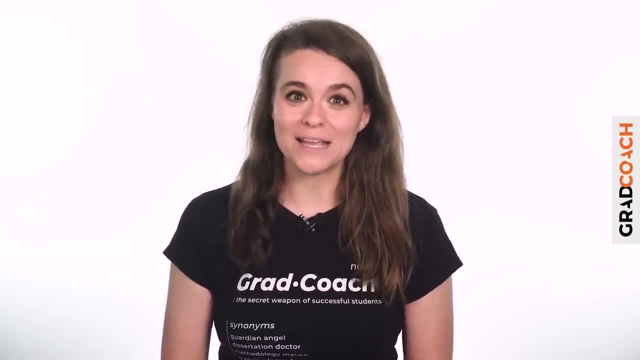 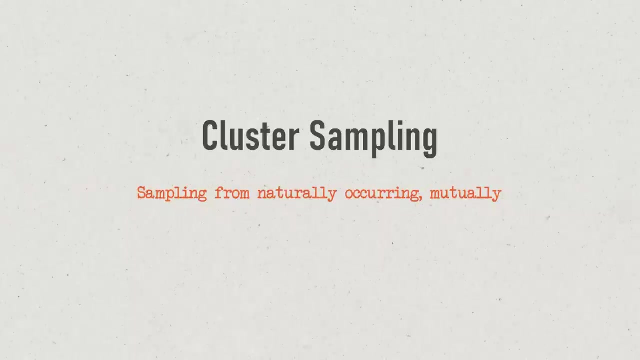 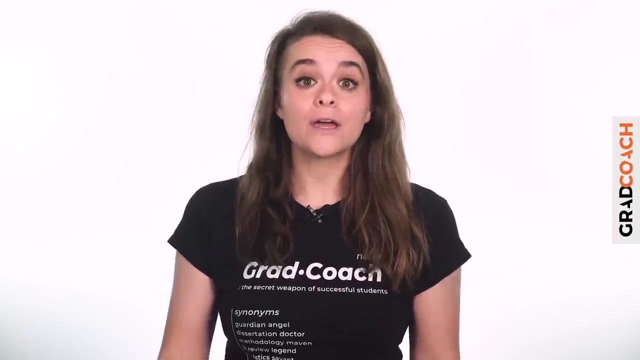 so, once again, you need to think about your research aims, as well as the nature of the population that you are interested in, so that you can make the right sampling choice. next up, let us look at cluster sampling. as the name suggests, this sampling method involves sampling from naturally occurring mutually exclusive clusters within a population, for example, area. 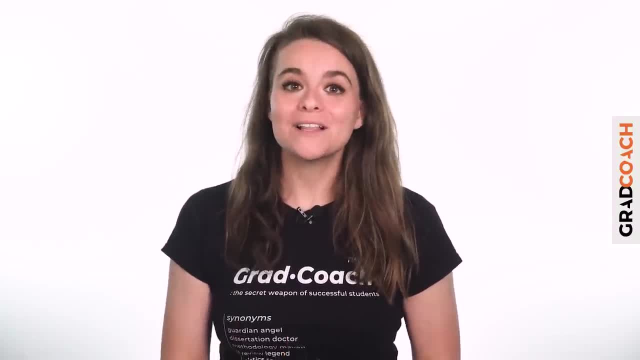 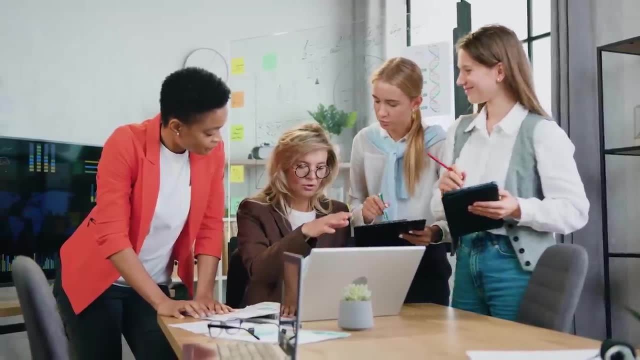 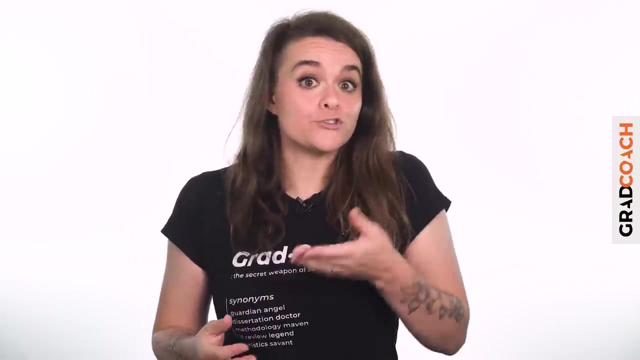 codes within a city or cities within a country. once the clusters are defined, a set of clusters are randomly selected and then a set of participants are randomly selected from each cluster. now you are probably wondering: how is cluster sampling different from stratified random sampling? well, let us look at the previous example, where each cluster reflects an area code. 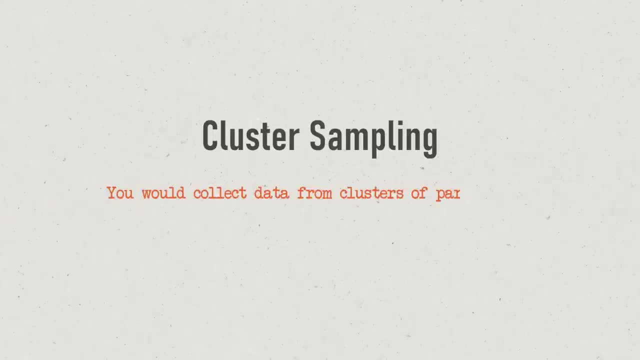 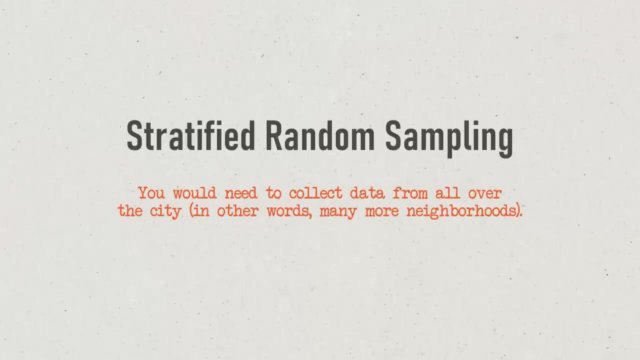 in a given city. with cluster sampling, you would collect data from clusters of participants in a handful of area codes, let us say five neighborhoods. conversely, with stratified random sampling, you would need to collect data from all over the city, in other words, many more neighborhoods. either way, you would still achieve the same sample size. let us say 200. 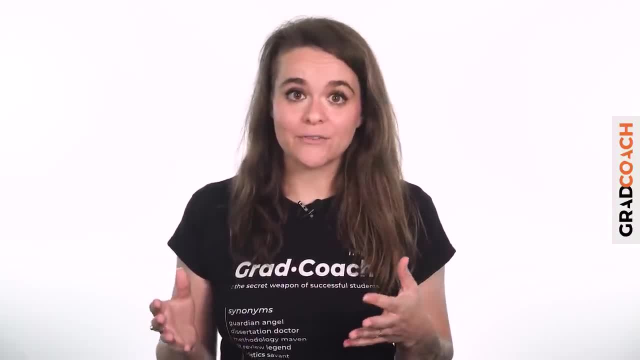 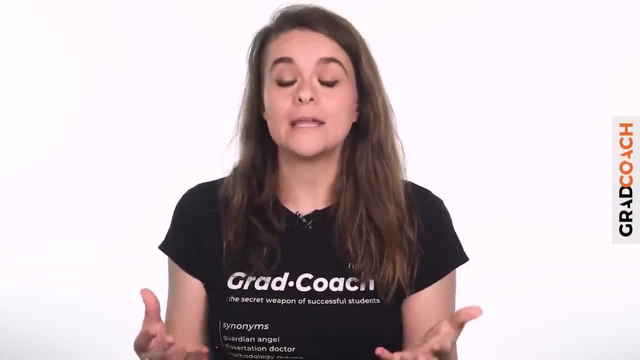 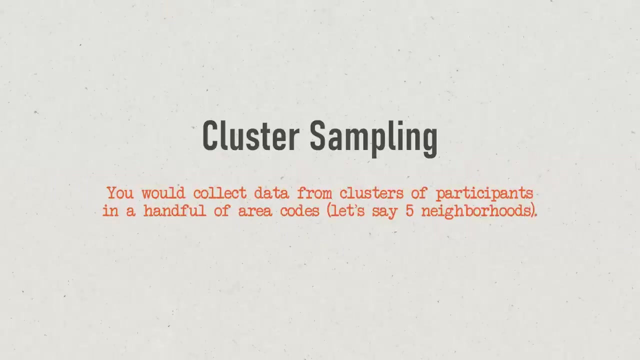 probably wondering: how is cluster sampling different from stratified random sampling? Well, let us look at the previous example, where each cluster reflects an area code in a given city. With cluster sampling, you would collect data from clusters of participants in a handful of area codes, let us say 5 neighborhoods. Conversely with stratified random sampling, you would need to collect data from all over the city, in other words, many more neighborhoods. Either way, you would still achieve the same sample size, let us say 200 people, for example- But with stratified sampling you would need to do a lot more running around as participants. 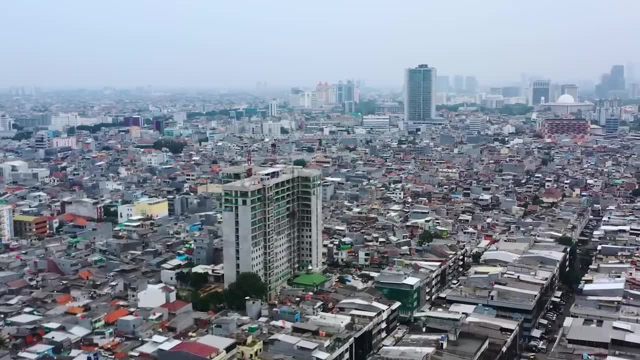 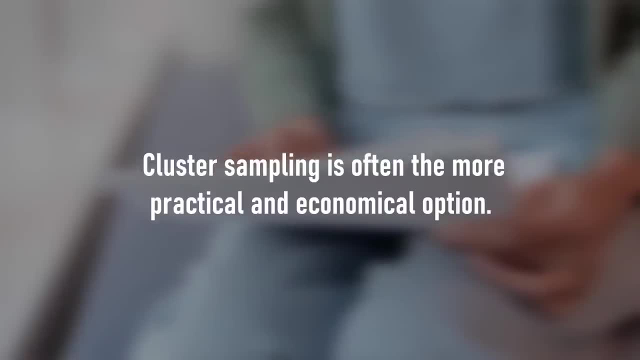 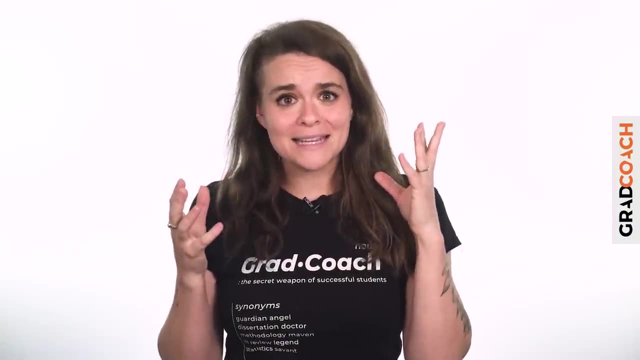 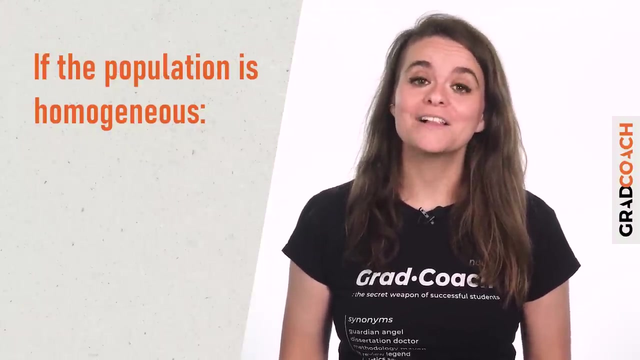 would be scattered across a more vast geographic area. As a result, cluster sampling is often the more practical and economical option, especially when the population spans a large geographic area. If that all sounds a little mind-bending, you can use the following general rule of thumb: If a population is relatively homogenous, cluster sampling will. 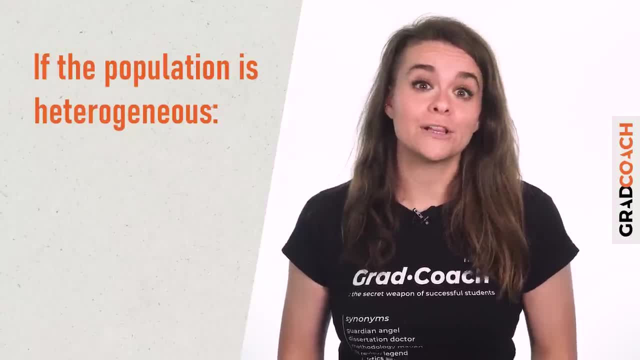 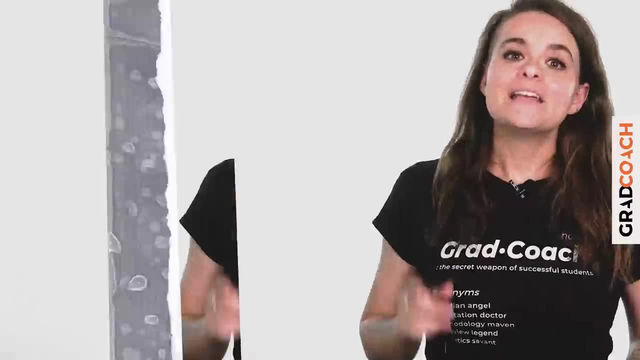 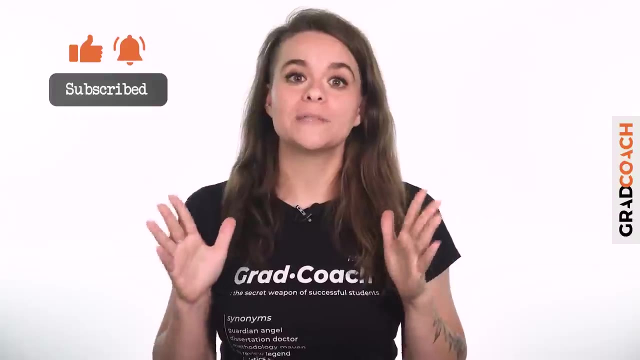 often do the trick. Conversely, if a population is generally quite heterogeneous, in other words, diverse, stratified sampling will often be more appropriate. If you are enjoying this video so far, please help us out by hitting that like button. You can also subscribe for loads of plain language, actionable advice. 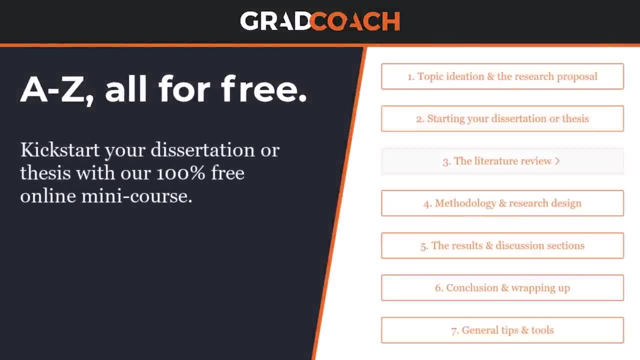 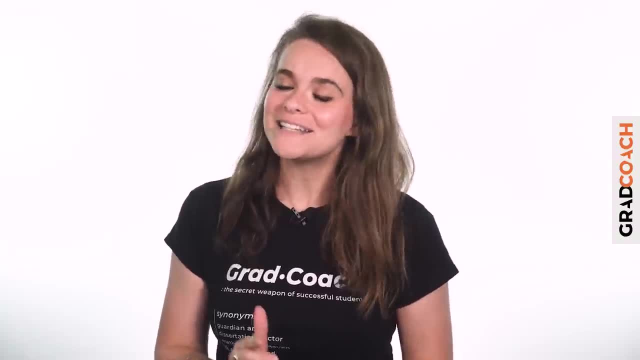 If you are new to research, check out our free dissertation writing course, which covers everything that you need to get started on your research project. As always, links are down in the description. Right now that we have looked at a few probability-based sampling methods, 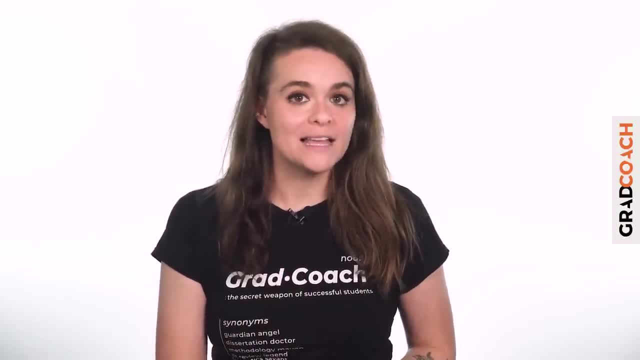 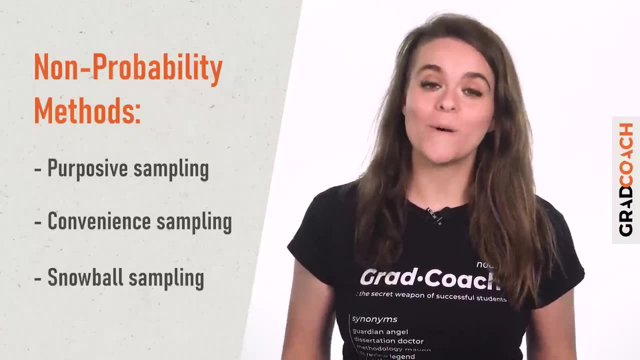 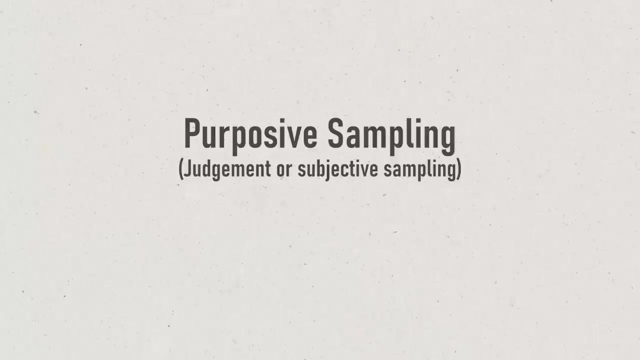 it is time to explore some non-probability methods. The three that we will be looking at are purposive sampling, convenience sampling and snowball sampling. First up, we have purposive sampling, also known as judgment or subjective sampling. The names here provide some clues, as this sampling method involves the researcher. 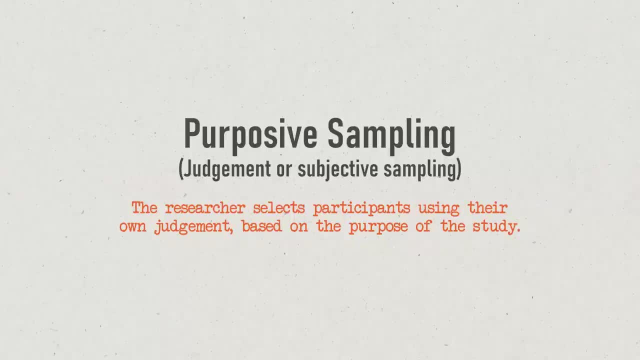 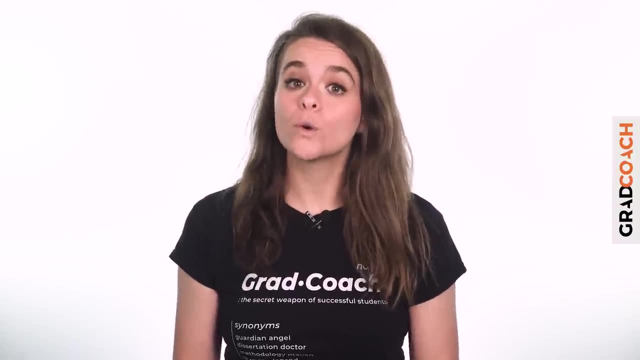 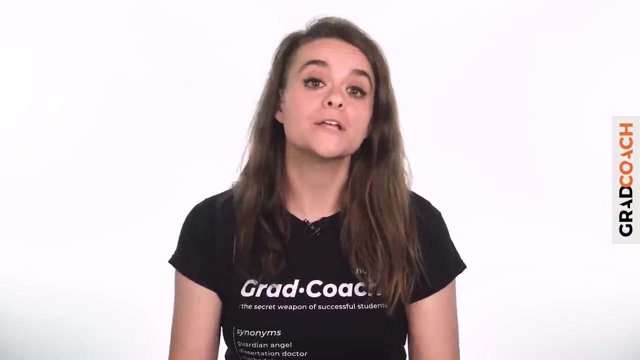 selecting participants using their own judgment, based on the purpose of the study, that is to say the research aims. For example, suppose your research aims were to understand the perceptions of hyper-loyal customers of a particular retail store. In that case, you could use your judgment. 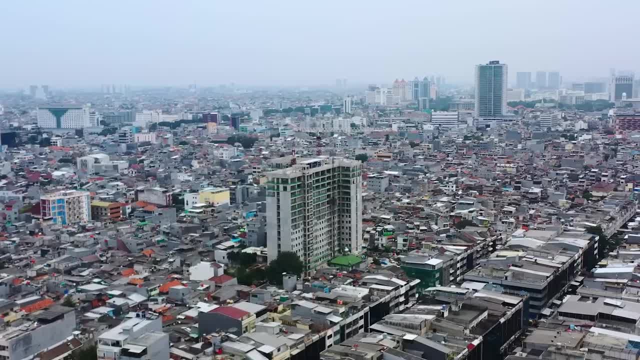 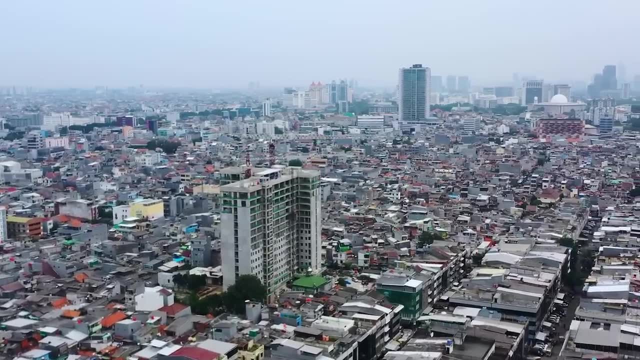 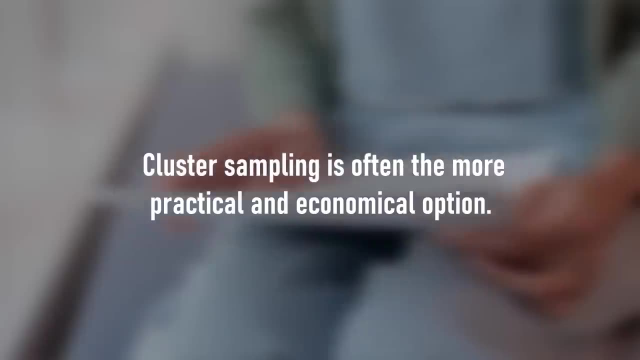 people, for example. but with stratified sampling you would need to do a lot more running around, as participants would be scattered across a more vast geographic area as a result. cluster sampling is often the more practical and economical option, especially when the population spans a large geographic area. if that all sounds a little mind-bending, you can. 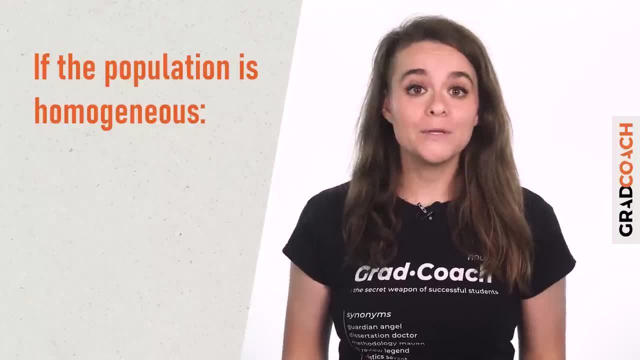 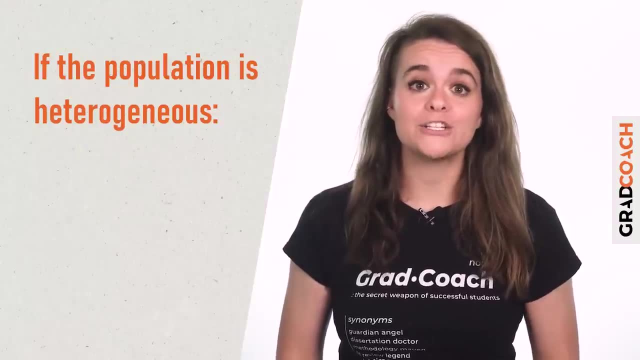 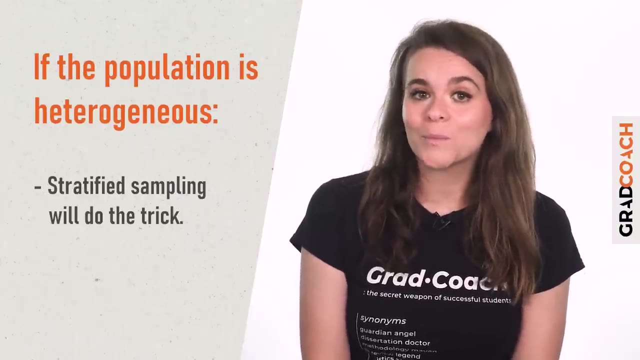 use the following general rule of thumb: if a population is relatively homogeneous, cluster sampling will often do the trick. conversely, if a population is generally quite heterogeneous- in other words, diverse, stratified sampling will often be more appropriate. if you are enjoying this video so far, please help us out by hitting that like button. you can also. 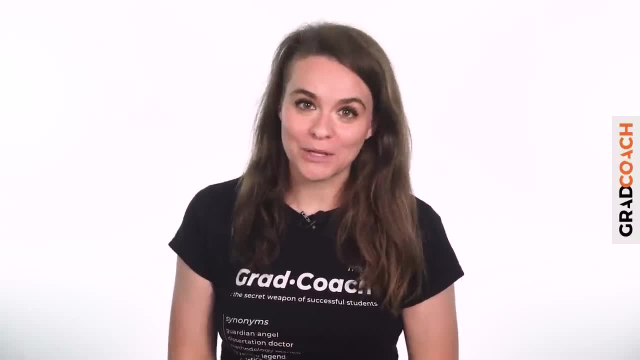 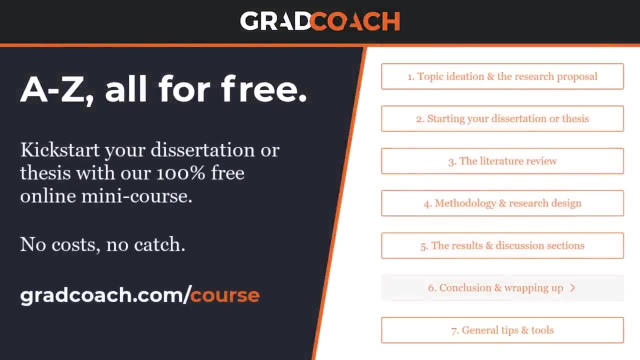 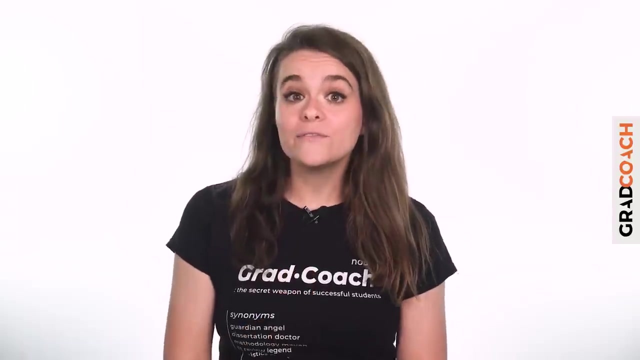 subscribe for loads of plain language. actionable advice. if you are new to research, check out our free dissertation writing course, which covers everything that you need to get started on your research project. as always, links are down in the description. right now that we have looked at a few, 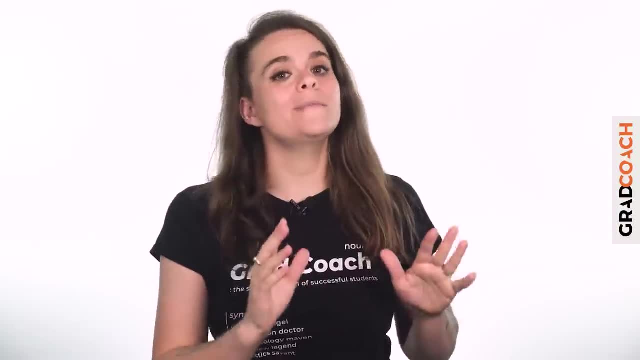 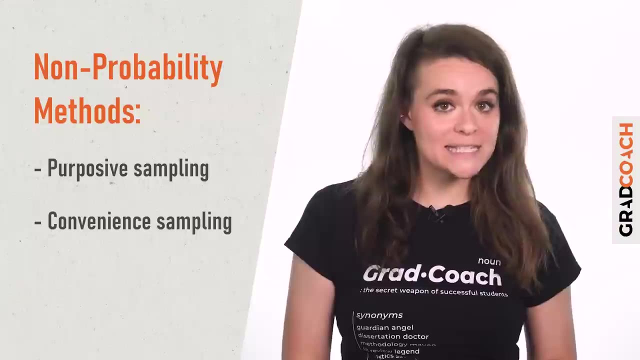 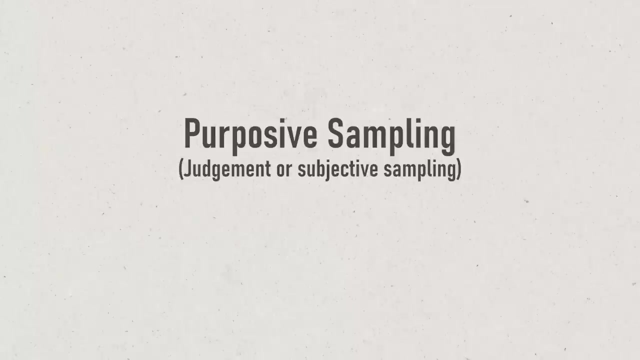 probability based sampling methods. it is time to explore some non-probability methods. the three that we will be looking at are purposive sampling, convenient sampling and snowball sampling. first up, we have purposive sampling, also known as judgmental or subjective sampling. The names here provides some clues. 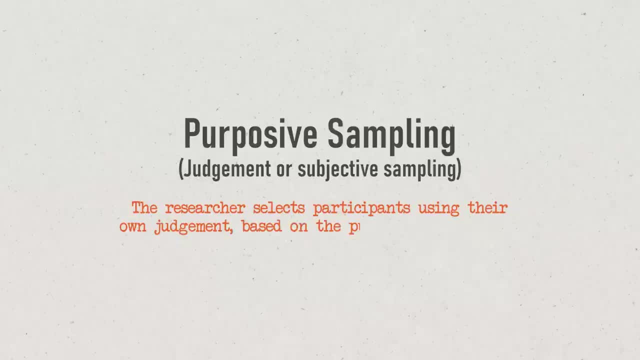 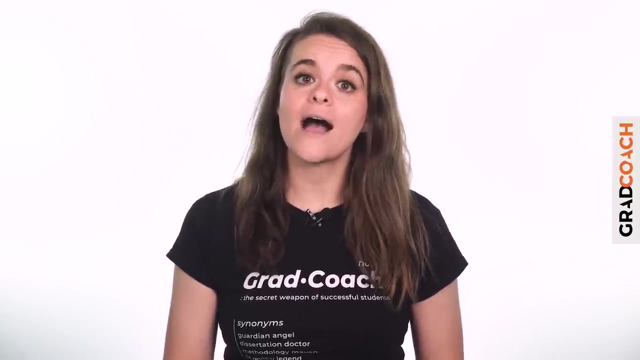 as the sampling method involves the researcher selecting participants using their own judgment, based on the purpose of the study, that is to say the research aims. For example, suppose your research aims were to understand the perceptions of hyper-loyal customers of a particular retail store. 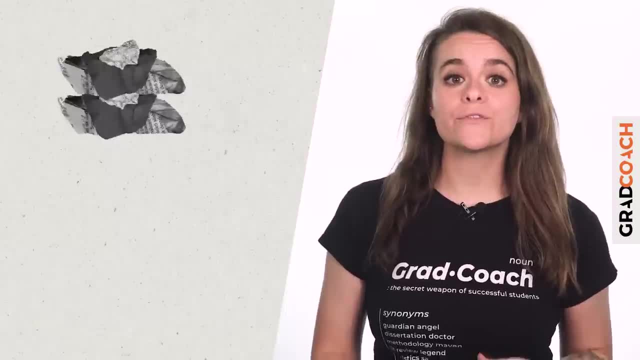 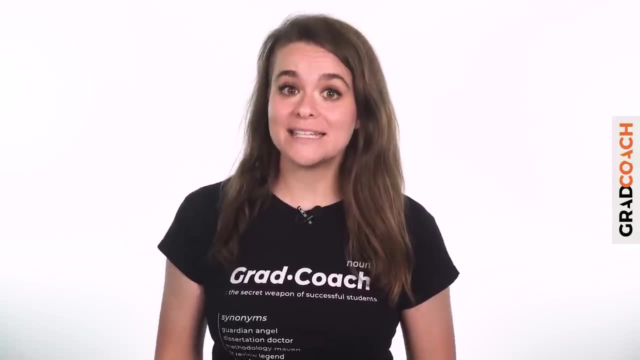 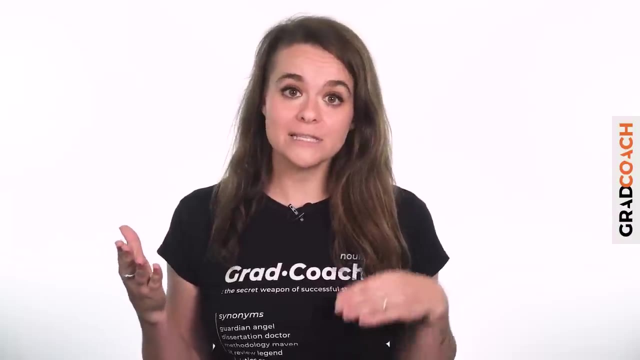 In that case, you could use your judgment to engage with frequent shoppers as well as rare or occasional shoppers and then analyze the resultant data to understand what perceptions and attitudes drive the two behavioral extremes frequent versus rare shopping. Purpose of sampling is often used in studies. 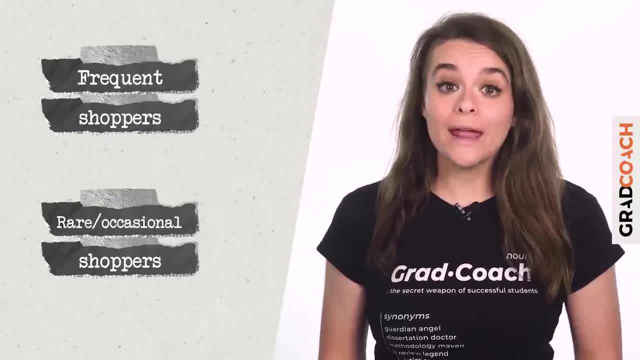 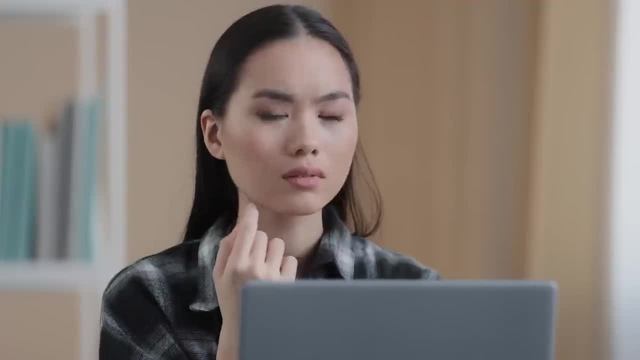 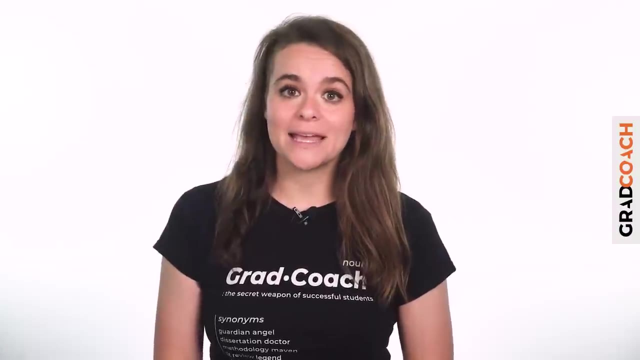 to engage with frequent shoppers, as well as to understand the perception of hyper-loyal customers, Then analyze the resultant data to understand what perceptions and attitudes drive the two behavioral extremes- frequent versus rare shopping. Purposive sampling is often used in studies where the aim is to gather information. 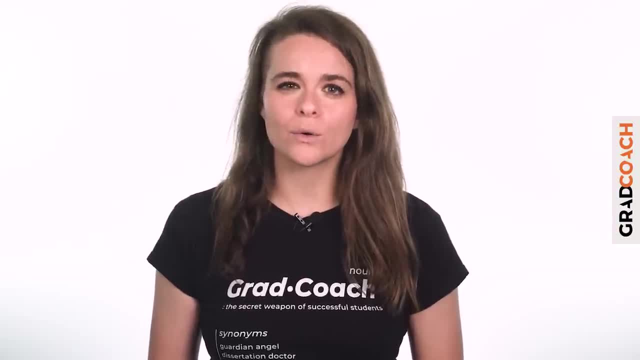 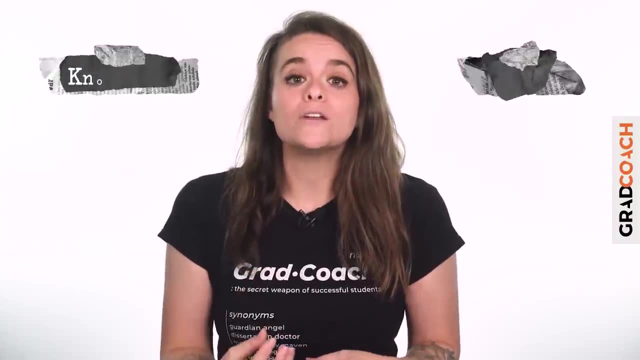 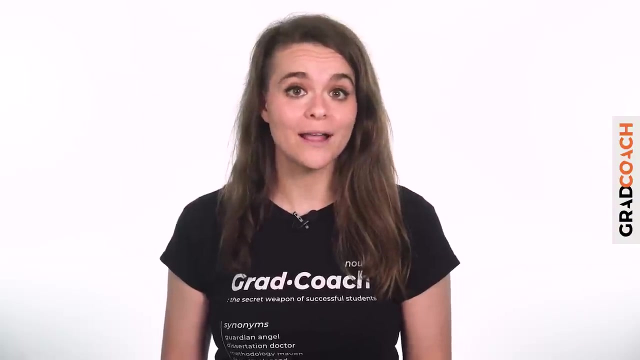 from a small population, especially rare or hard-to-find populations, as it allows the researcher to target specific individuals who have unique knowledge or experience. Naturally, this sampling method is quite prone to research bias and judgment error, and it is unlikely to produce generalizable results, so it is best suited to studies where 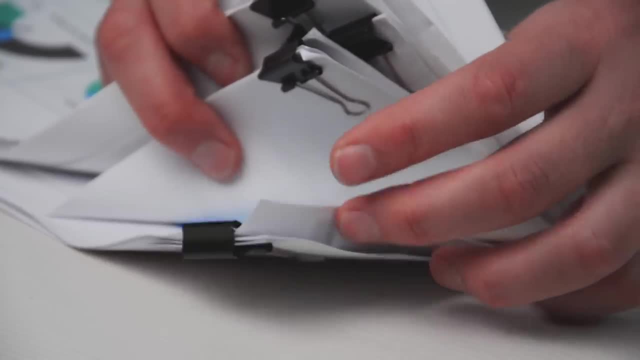 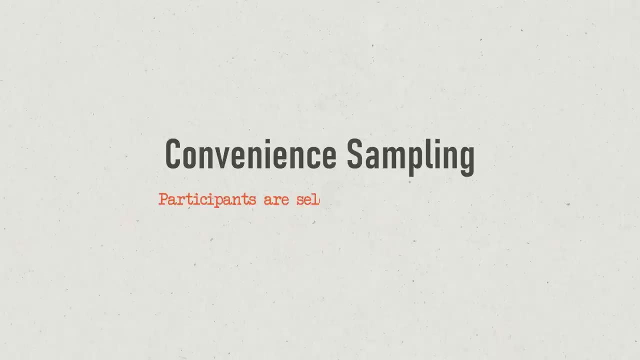 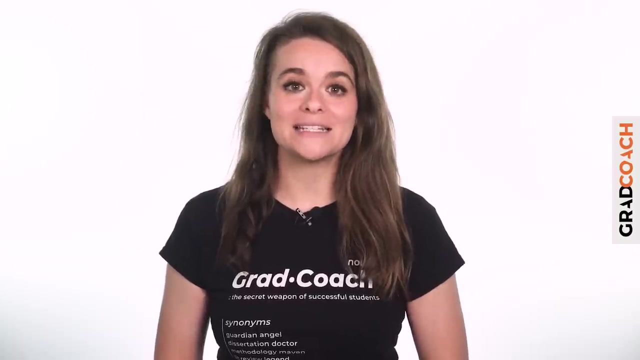 the aim is to go narrow and deep rather than broad. Next up, let us look at convenience sampling. As the name suggests, with this method, participants are selected based on their availability or accessibility. In other words, the sample is selected based on their availability or accessibility. 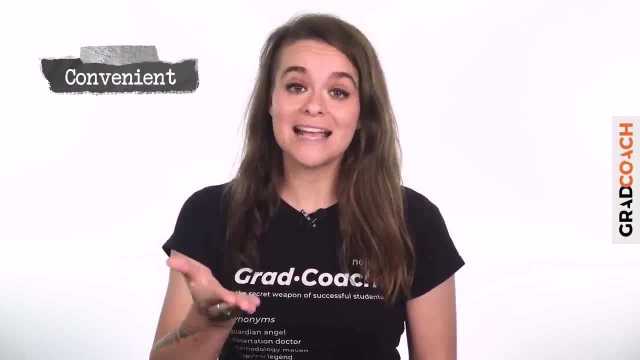 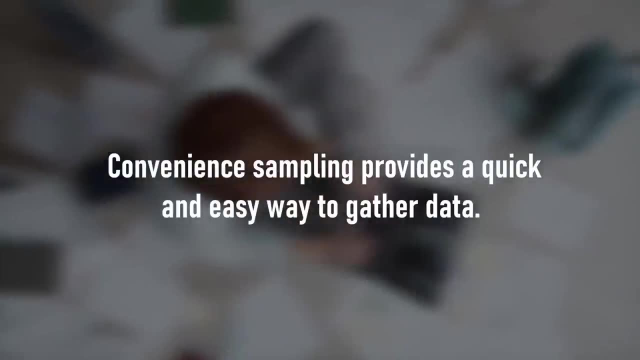 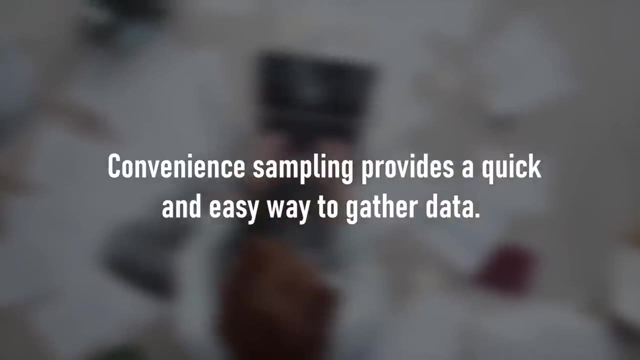 The sample is selected based on how convenient it is for the researcher to access it, as opposed to using a predefined or objective or consistent process. Naturally, convenience sampling provides a quick and easy way to gather data, as the sample is selected based on the individuals who are readily available and willing. 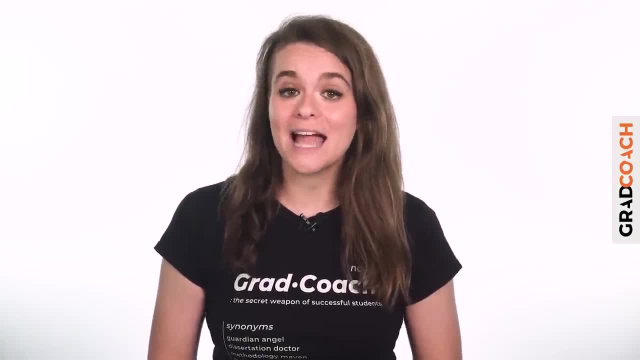 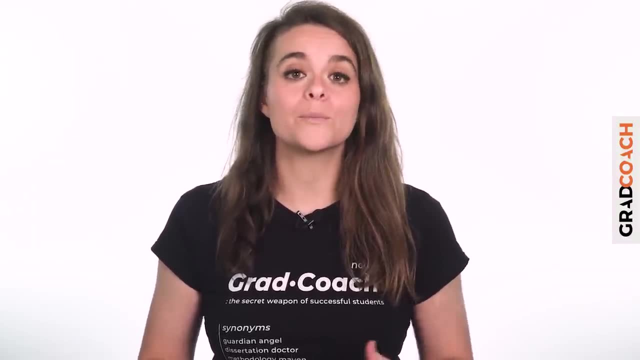 This makes it an attractive option if you are particularly tight on resources or time. But, as you would expect, this sampling method is unlikely to produce good results. This makes it an attractive option if you are particularly tight on resources or time, is unlikely to produce a representative sample. 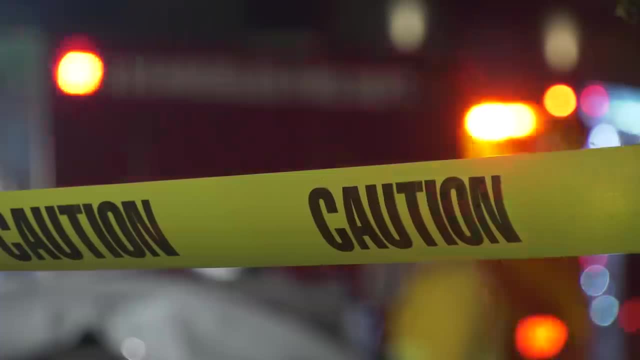 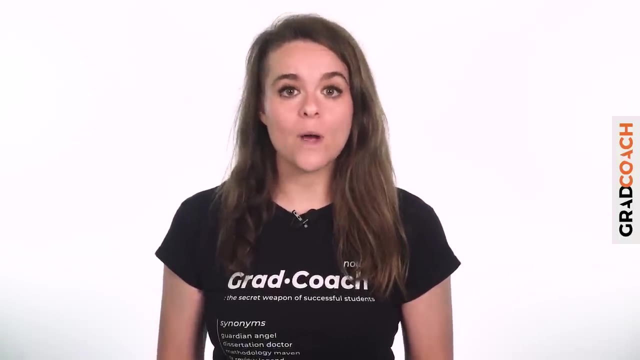 and will, of course, be vulnerable to research bias, So it is important to approach it with caution. By the way, if you want to learn more about research bias, check out our video about that up here, or you can hit the link in the description. 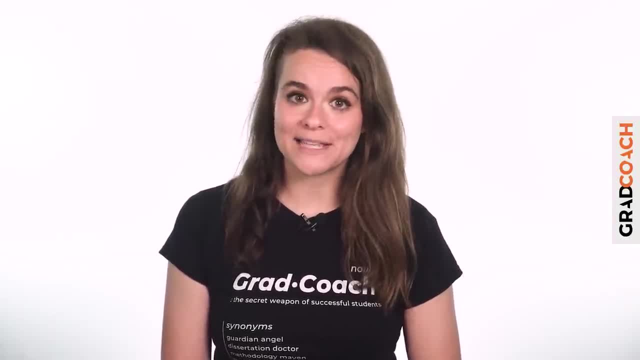 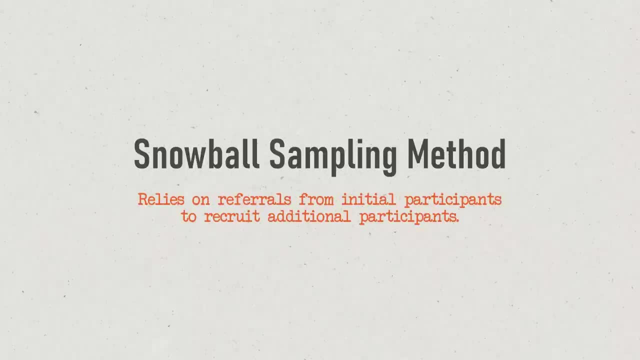 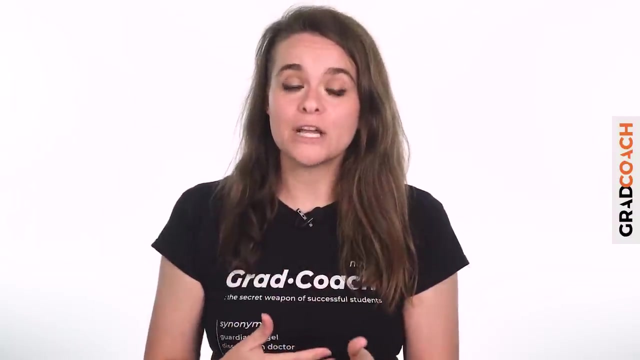 Last but certainly not least, we have the snowball sampling method. This method relies on referrals from initial participants to recruit additional participants. In other words, the initial subjects from the first small snowball and each additional subject recruited through a referral is added to the snowball. 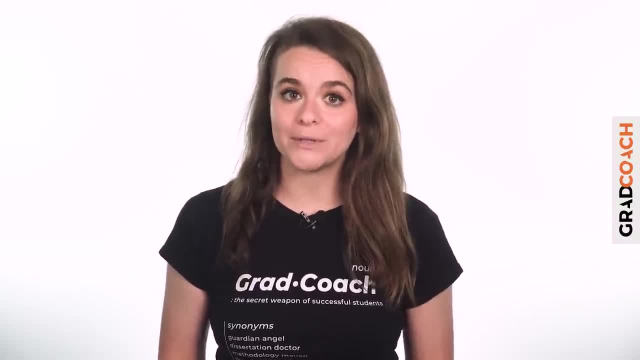 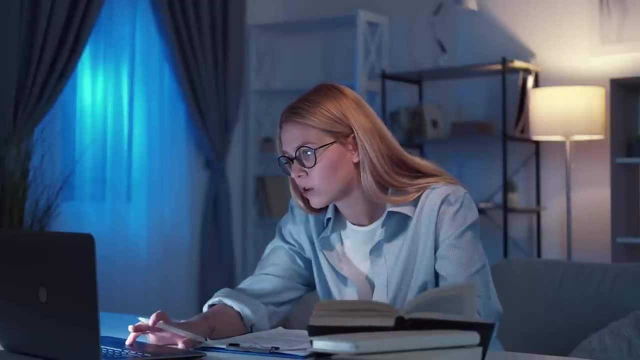 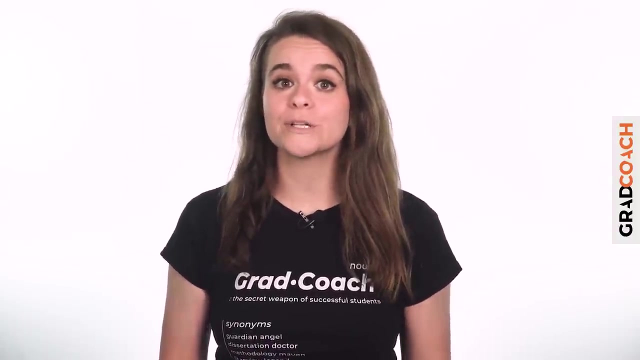 where the aim is to gather information from a small population, especially rare or hard to find populations, as it allows the researcher to target specific information: individuals who have unique knowledge or experience. Naturally, this sampling method is quite prone to research bias and judgment error. 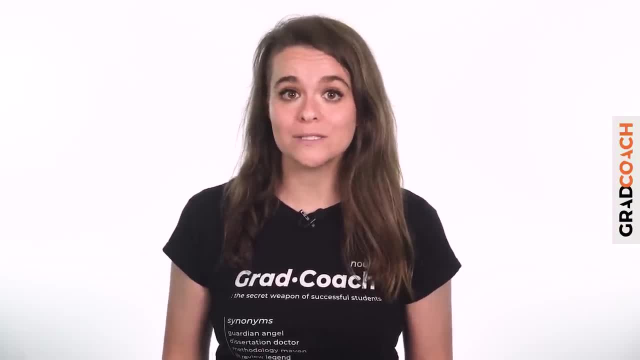 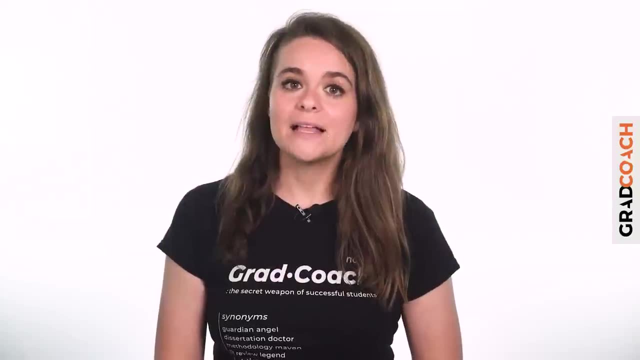 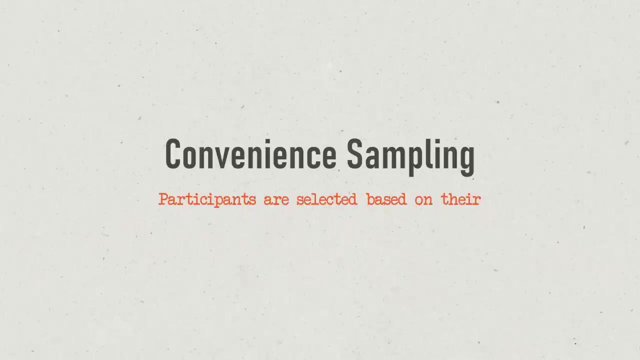 and it is unlikely to produce generalizable results, so it is best suited to studies where the aim is to go narrow and deep rather than broad. Next up, let us look at convenient sampling, As the name suggests, with this method, participants are selected based on their availability. 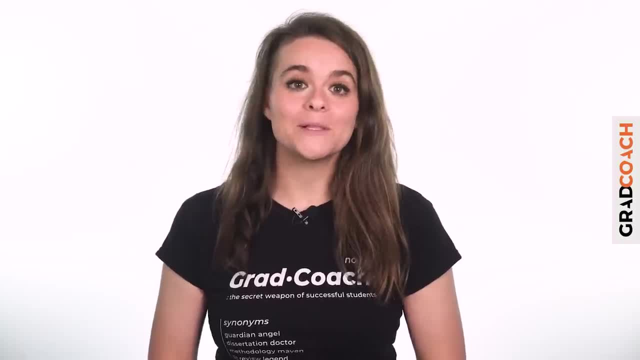 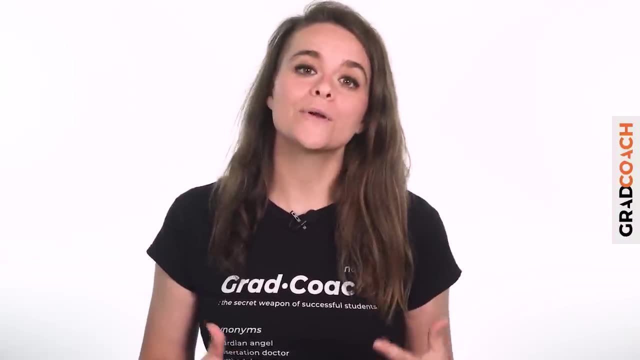 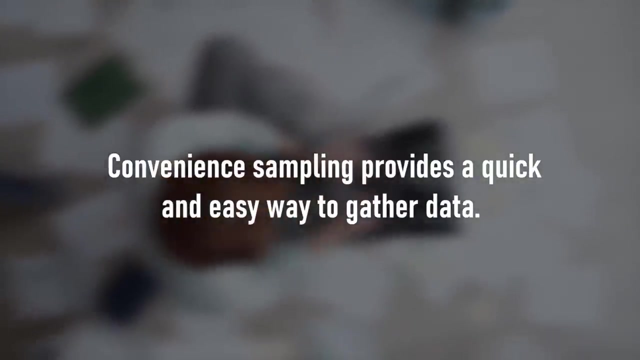 or accessibility. In other words, the sample is selected based on how convenient it is for the researcher to access it, as opposed to using a predefined or objective or consistent process. Naturally, convenient sampling provides a quick and easy way to gather data, as the sample is selected based on the individuals. 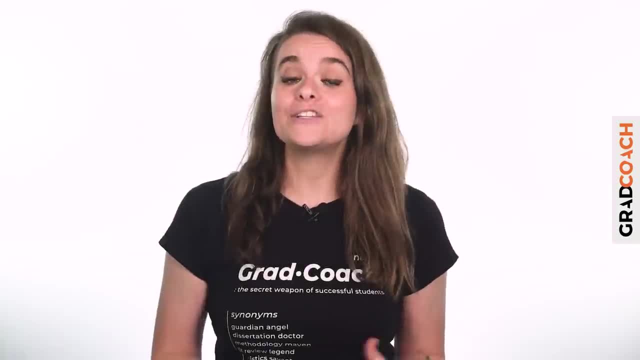 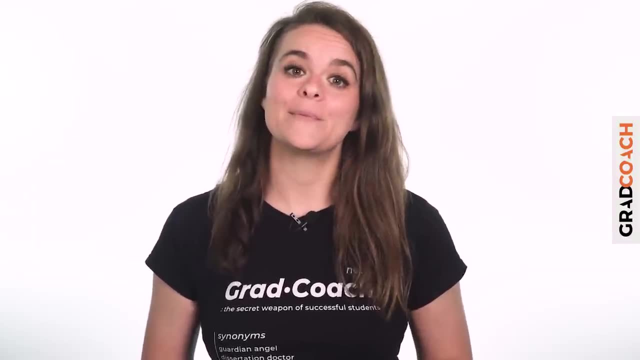 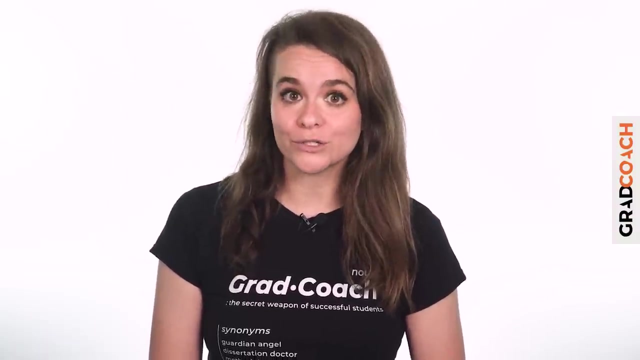 who are readily available and willing. This makes it an attractive option if you are particularly tight on resources or time, but as you wish, you would expect, this sampling method is unlikely to produce a representative sample and will, of course, be vulnerable to research bias. 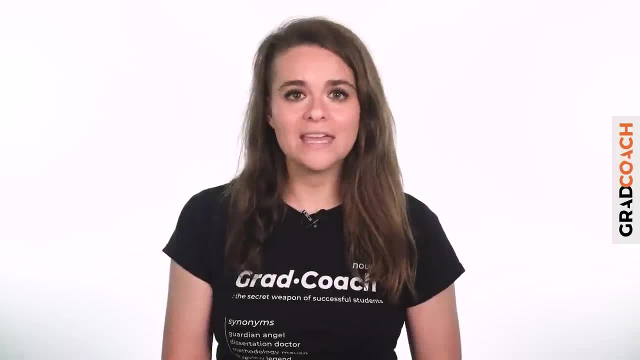 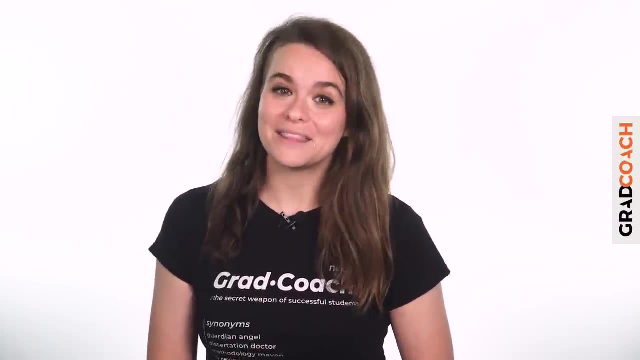 so it is important to approach it with caution. By the way, if you want to learn more about research bias, check out our video about that up here, or you can hit the link in the description. Last but certainly not least, we have the snowball sampling method. 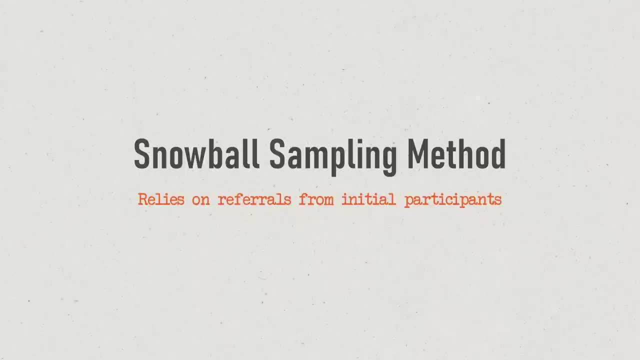 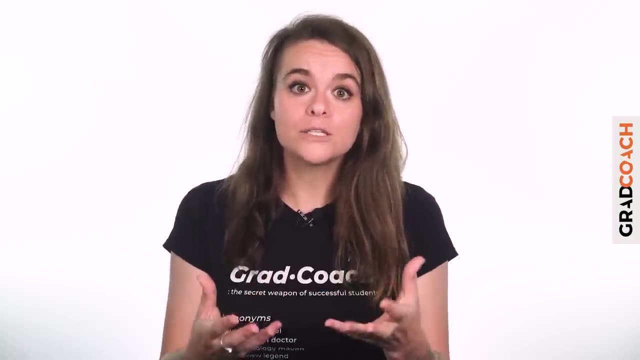 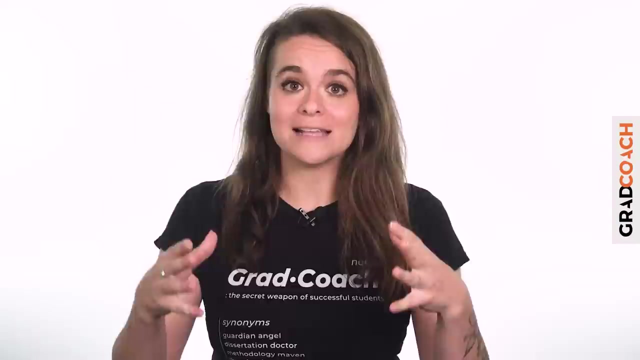 This method relies on referrals from initial participants to recruit additional participants. In other words, the initial subjects from the first small snowball and each additional subject recruited through referral is added to the snowball, making it larger as it rolls along. Snowball sampling is often used in situations 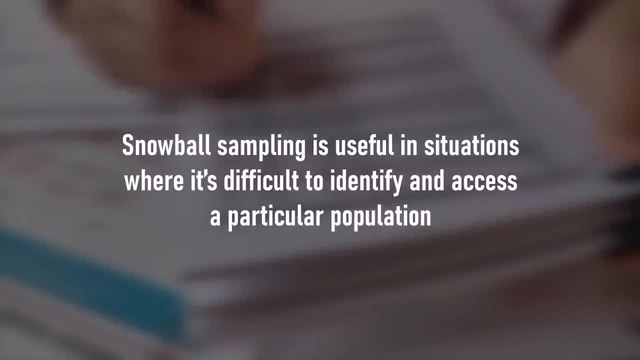 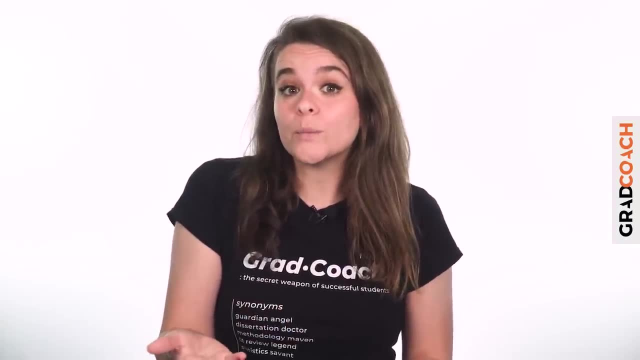 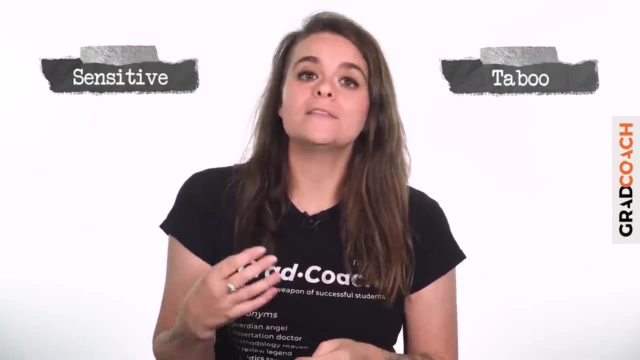 where it is difficult to identify and access a particular population, For example, people with a rare medical condition or members of an exclusive group. It can also be useful in cases where the research topic is sensitive or taboo and people are unlikely to open up. 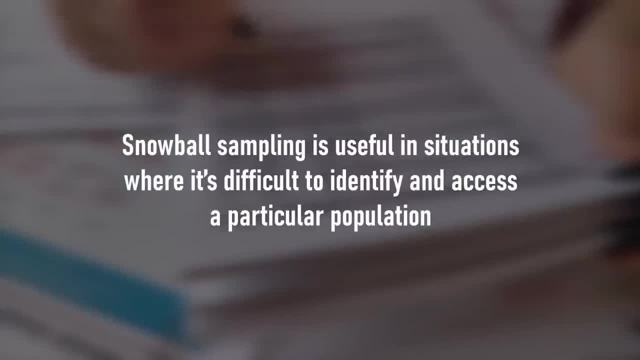 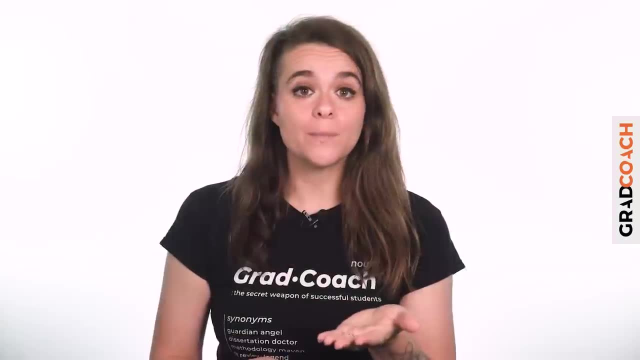 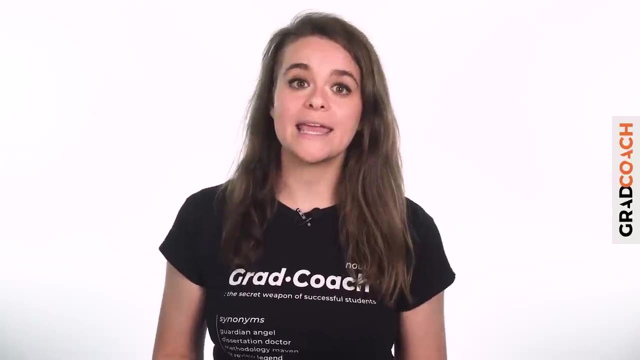 making it larger as it rolls along. Snowball sampling is often used in situations where it is difficult to identify and access a particular population, For example, people with a rare medical condition or members of an exclusive group. It can also be useful in cases 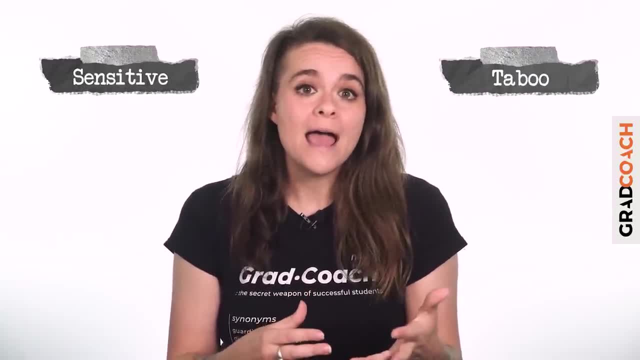 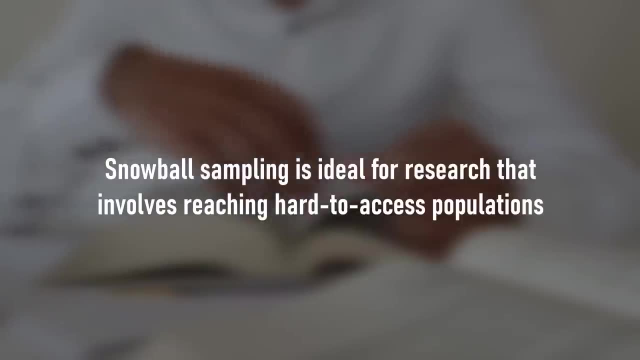 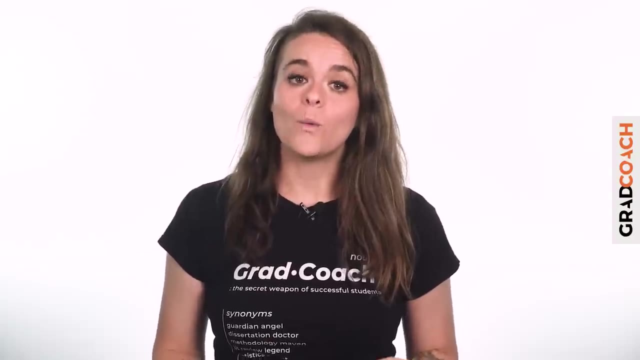 where the research topic is sensitive or taboo and people are unlikely to open up unless they're referred to by someone that they trust. Simply put, snowball sampling is ideal for research that involves reaching hard to access populations, But keep in mind that, once again, 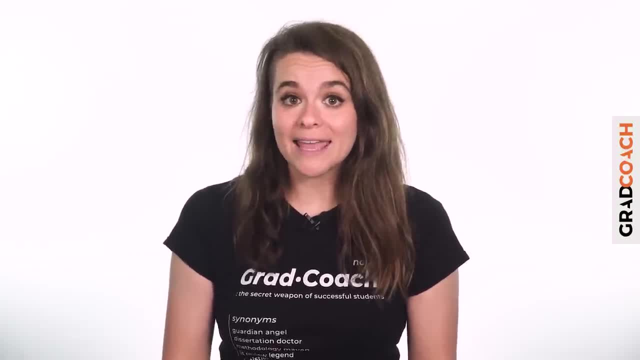 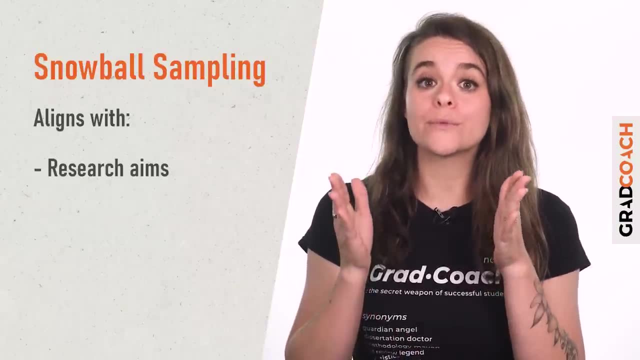 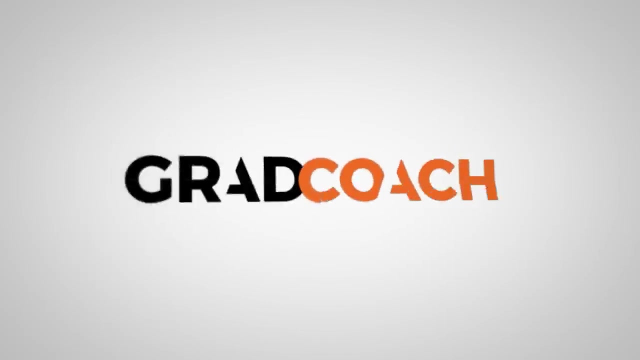 it's a sampling method that's highly prone to researcher bias and is unlikely to produce a representative sample, So make sure that it aligns with your research aims and research questions before you start rolling your snowball down the hill. Now that we've looked at a few popular sampling methods, 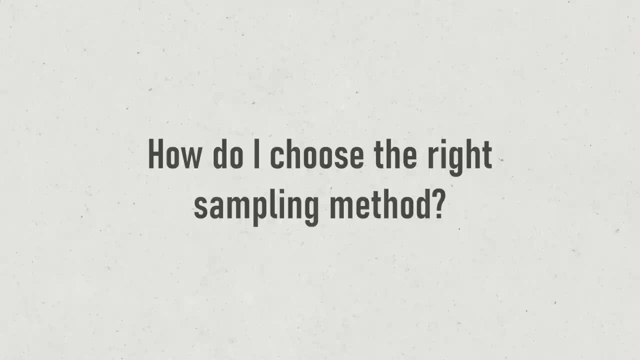 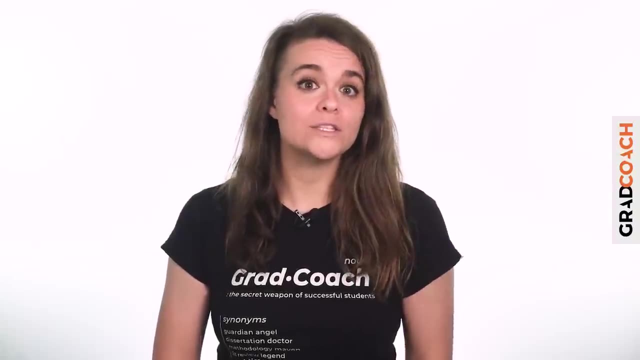 both probability and non-probability based. the obvious question is: how do I choose the right method of sampling for my study? This is a big question and we could do an entire video covering this, but I'll try to cover the essentials here. 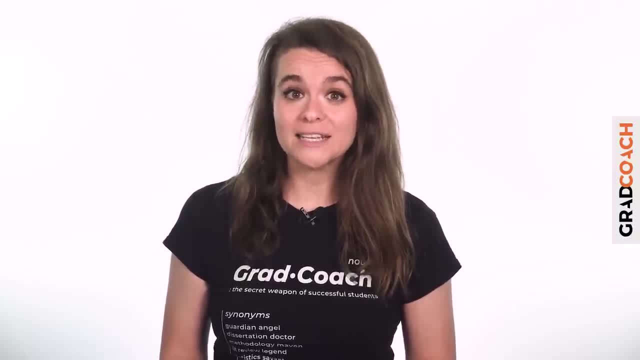 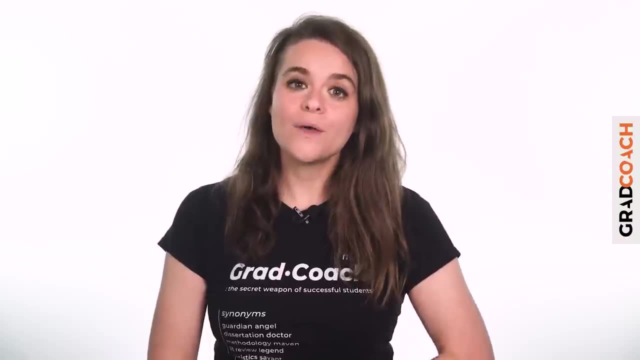 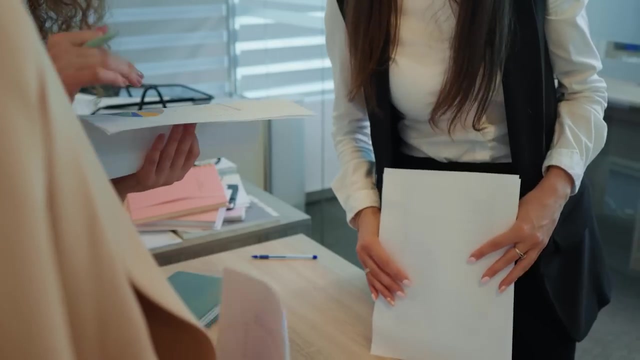 When selecting a sampling method for your research project, you'll need to consider two important factors: your research aims and your resources. As with all research design and methodology choices, your sampling approach needs to be guided by and aligned with your research aims, objectives and research questions. 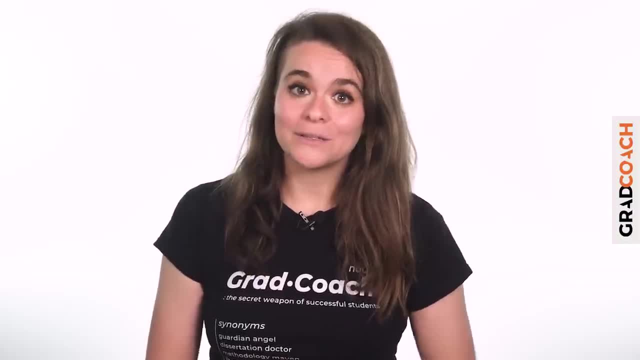 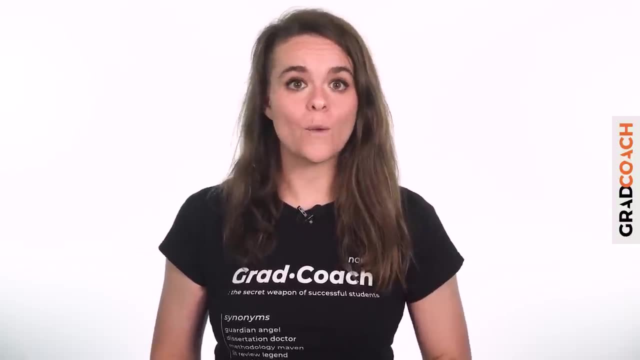 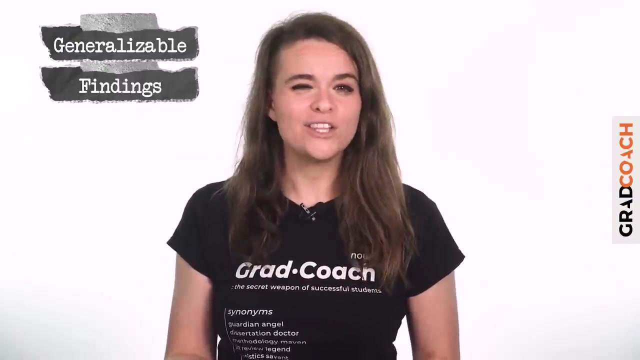 In other words, your golden thread. I know I'm starting to sound like a stuck record here, but this alignment is really important. Specifically, you need to consider whether your research aims are primarily concerned with producing generalizable findings, in which case you'll likely opt. 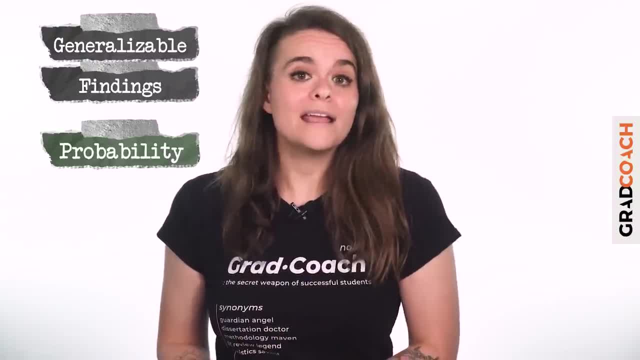 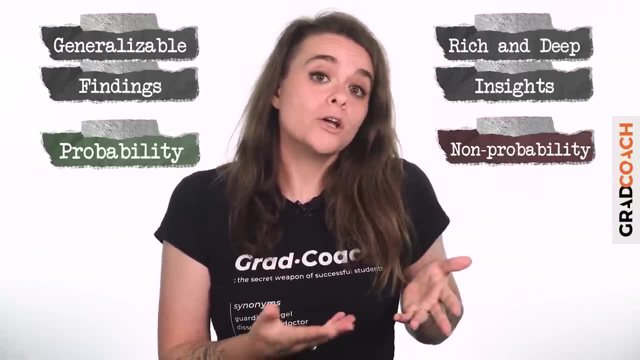 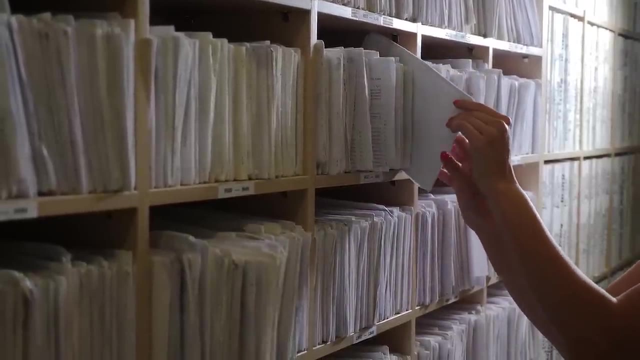 for a probability-based sampling method, or if they're more focused on developing rich, deep insights, in which case a non-probability based approach could be more practical. Typically, quantitative studies lean towards the former, while qualitative studies lean towards the latter. 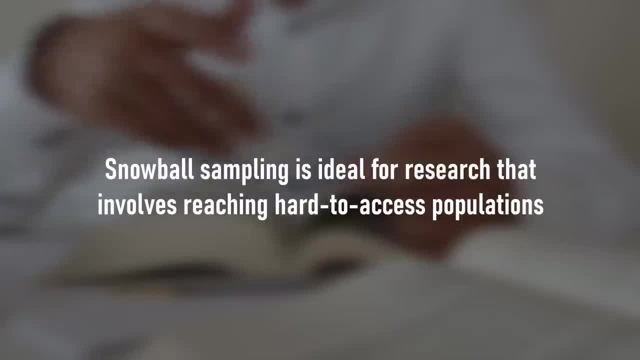 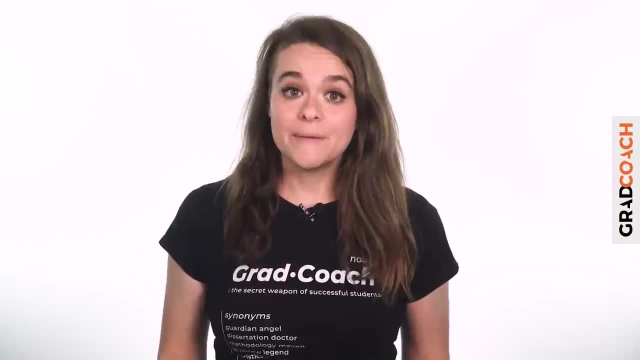 unless they are referred to by someone that they trust. Simply put, snowball sampling is ideal for research that involves reaching hard-to-access populations, but keep in mind that, once again, it is a sampling method that is highly prone to researcher bias. 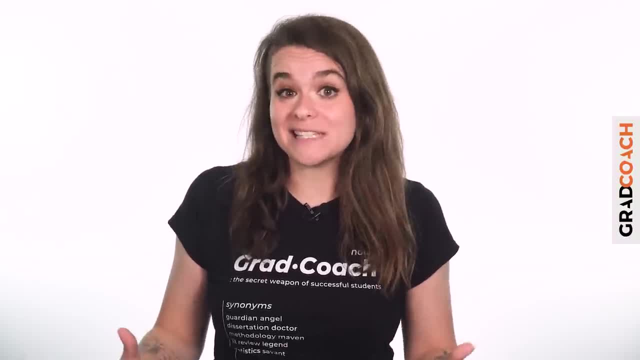 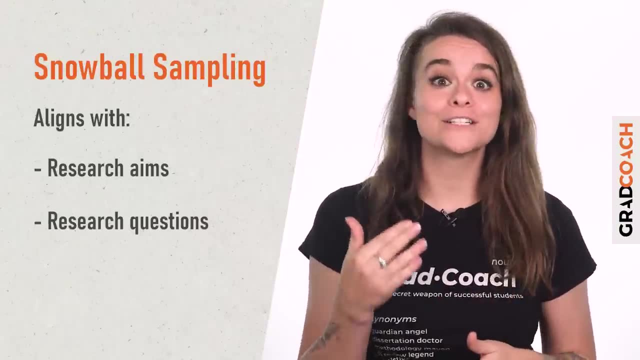 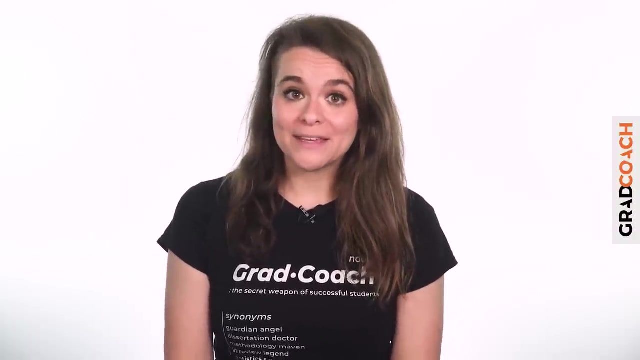 and is unlikely to produce a representative sample. So make sure that it aligns with your research aims and research questions before you start rolling your snowball down the hill. Now that we have looked at a few popular sampling methods, both probability and non-probability based, 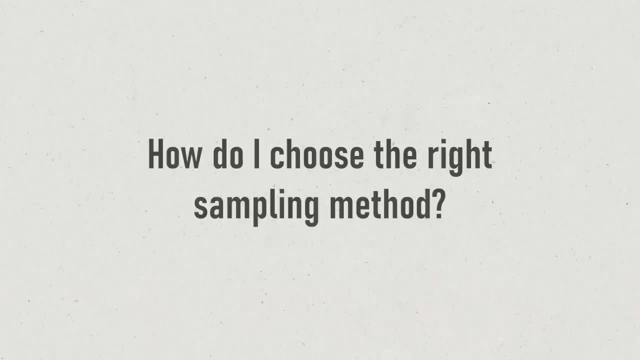 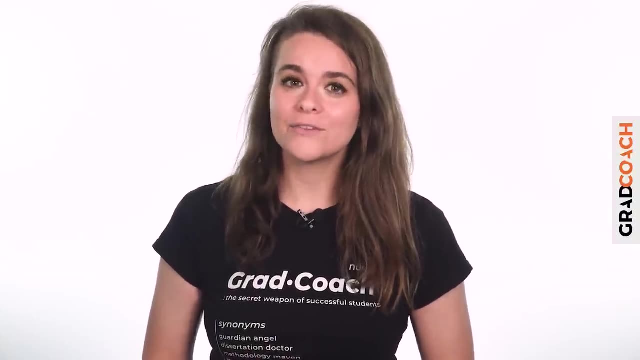 the obvious question is: how do I choose the right method of sampling for my study? This is a big question and we could do an entire video covering this, but I will try to cover the essentials here When selecting a sampling method for your research project. 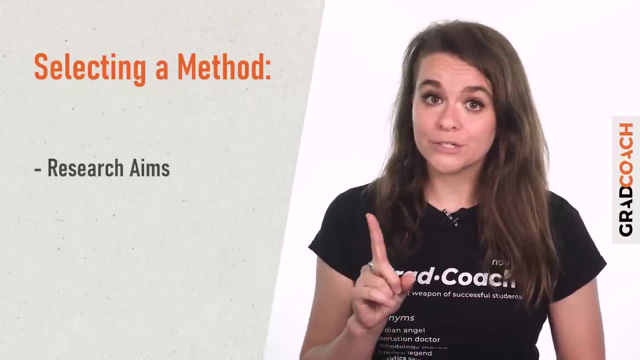 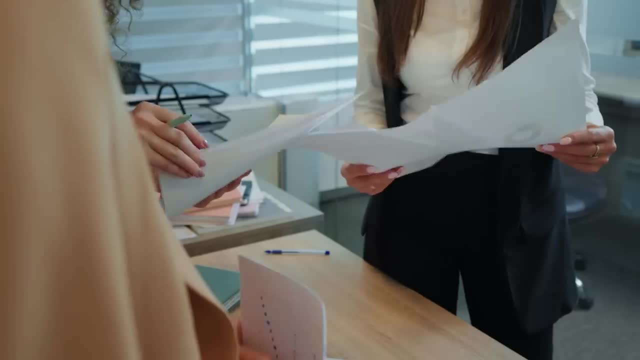 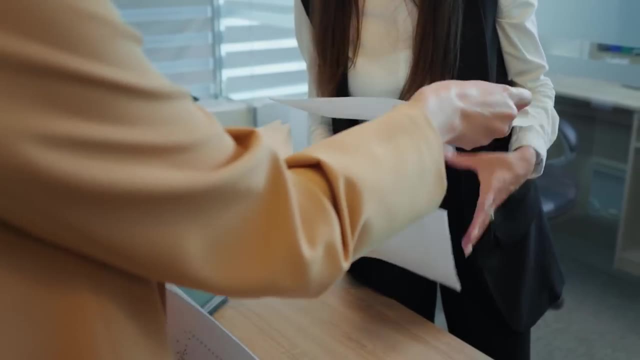 you will need to consider two important factors: your research aims and your resources. As with all research design and methodology choices, your sampling approach needs to be guided by and aligned with your research aims, objectives and research questions, In other words, your golden thread. 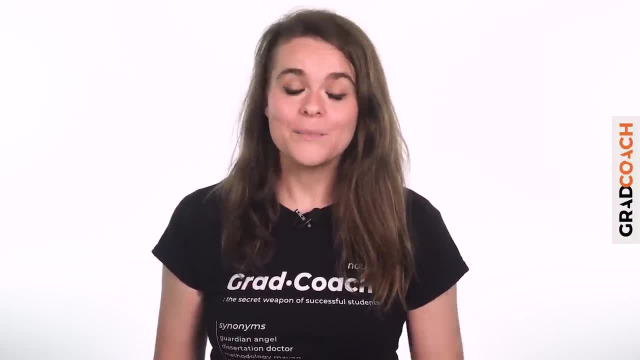 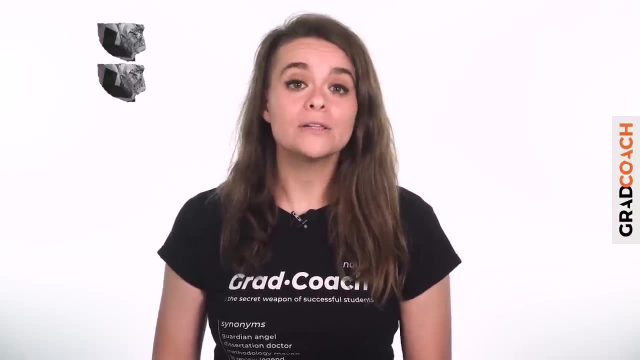 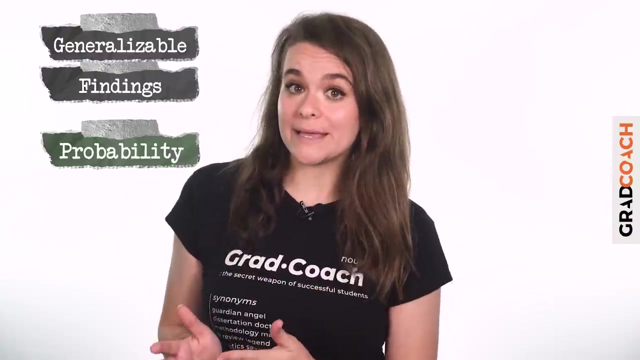 I know I am starting to sound like a stuck record here, but this alignment is really important. Specifically, you need to consider whether your research aims are primarily concerned with producing generalizable findings, in which case you will likely opt for a probability based sampling method. 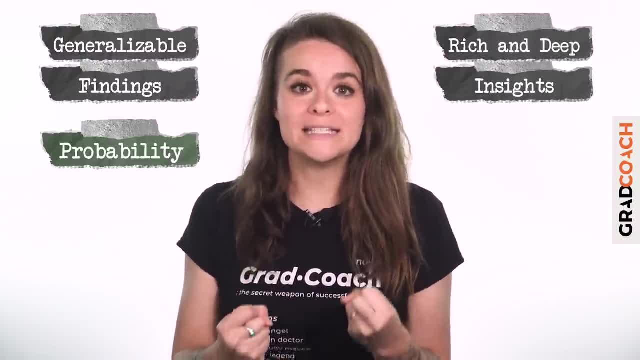 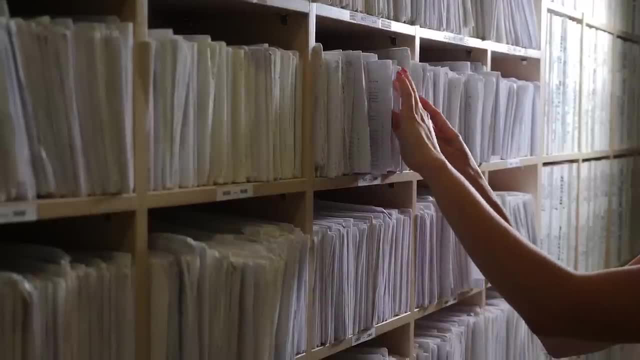 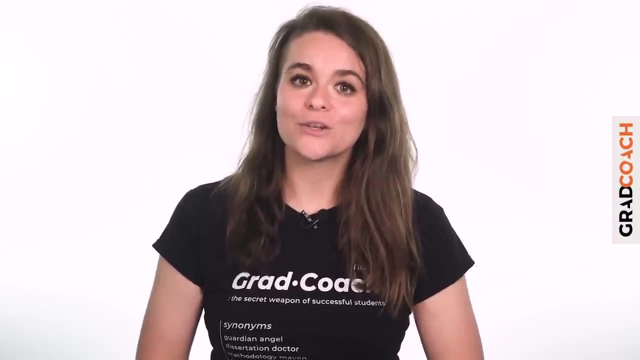 or if they are more focused on developing rich, deep insights, in which case a non-probability based approach could be more practical. Typically, quantitative studies lean towards the former, while qualitative studies lean towards the latter, so be sure to consider your broader methodology as well. 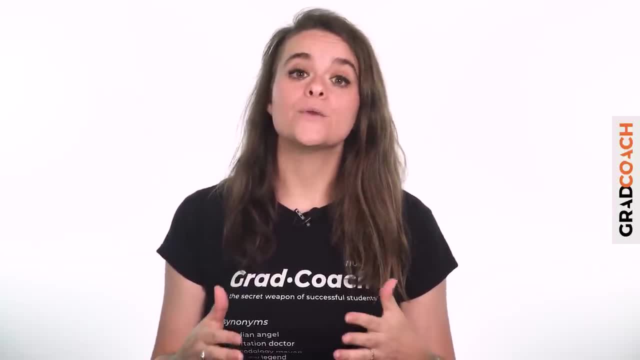 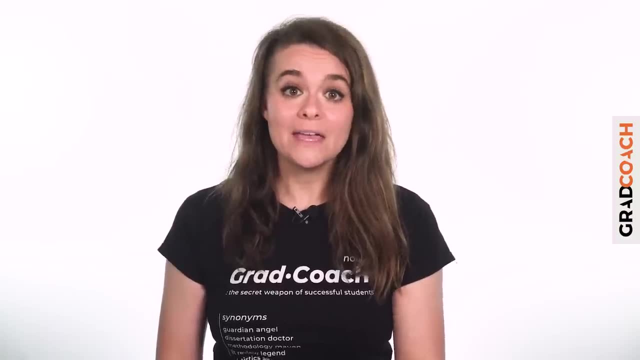 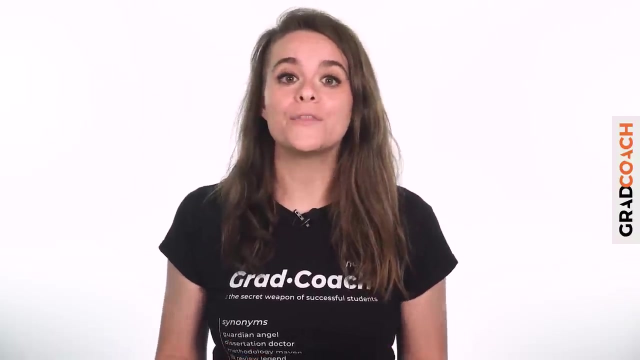 The second factor you need to consider is your resources and, more generally, the practical constraints at play. For example, if you have easy, free access to a large sample at your workplace or university, along with a healthy budget to help attract your participants. 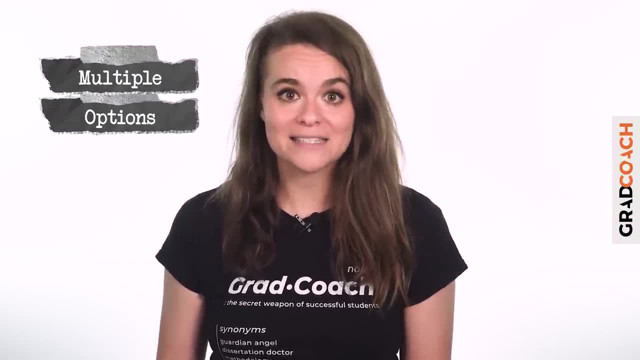 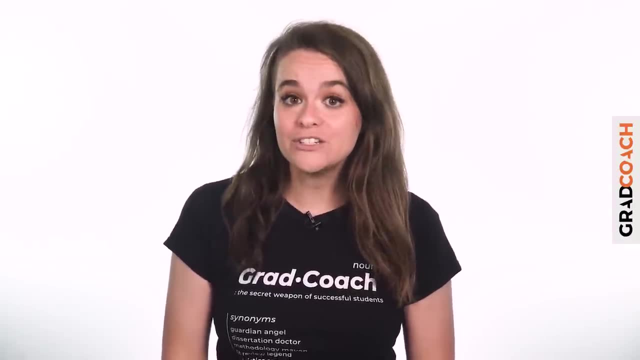 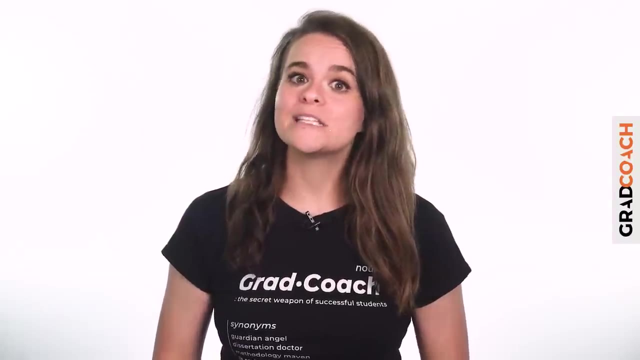 that will open up multiple options in terms of sampling methods. Conversely, if you are cash strapped, short on time and do not have unfettered access to your population of interest, you may be restricted to convenience or referral-based methods. Importantly, you need to be ready for trade-offs. 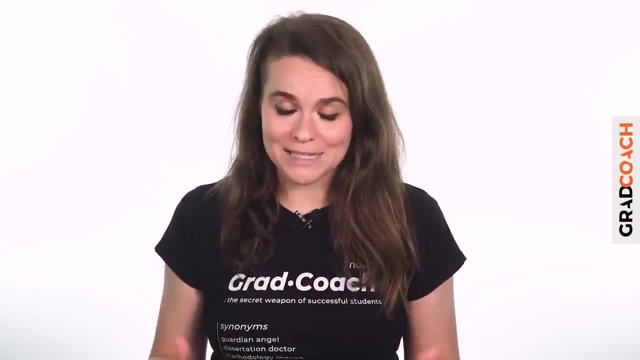 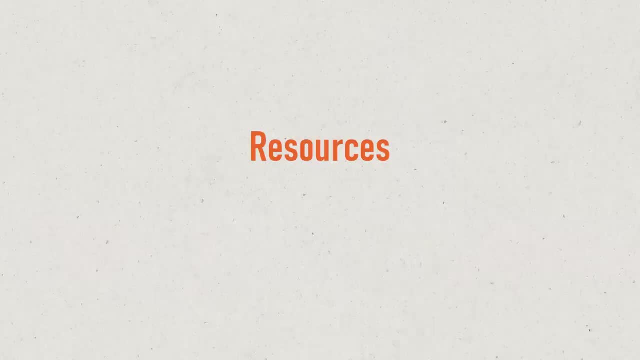 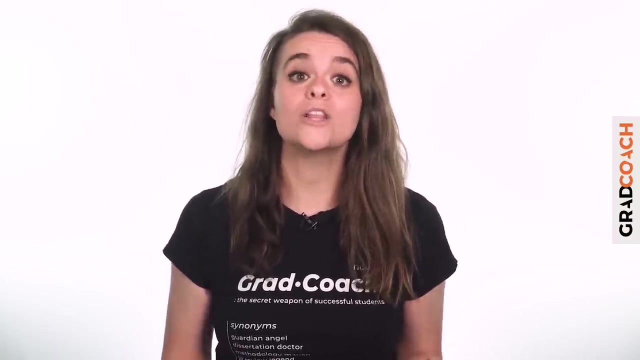 So be sure to consider your broader methodology as well. The second factor you need to consider is your resources and, more generally, the practical constraints at play. For example, if you have easy, free access to a large sample at your workplace or university. 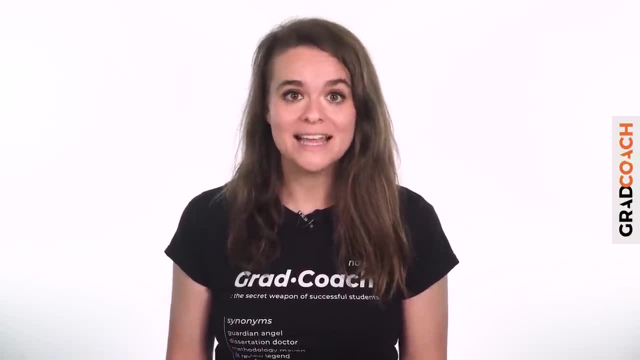 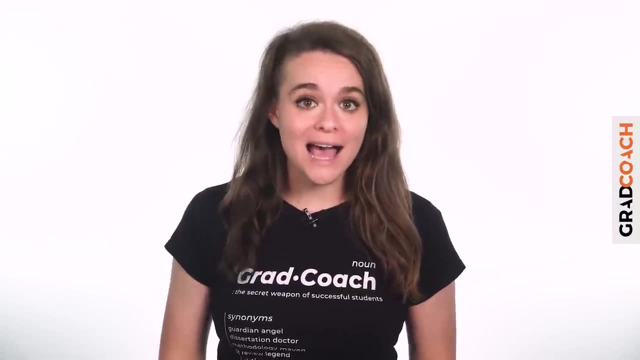 along with a healthy budget to help attract your participants. that will open up multiple options in terms of sampling methods. Conversely, if you're cash strapped short on time and don't have unfettered access to your population of interest, you may be restricted to convenience. 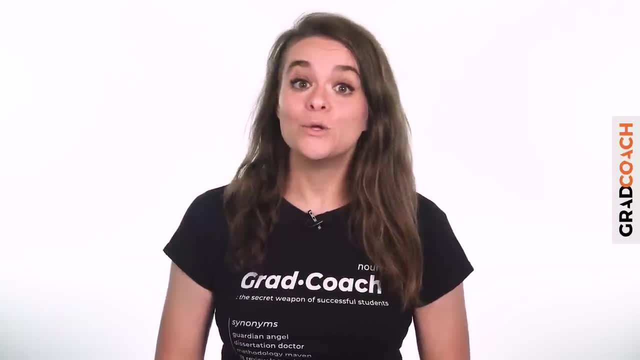 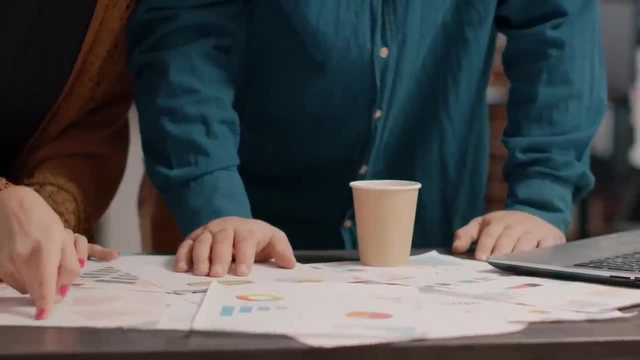 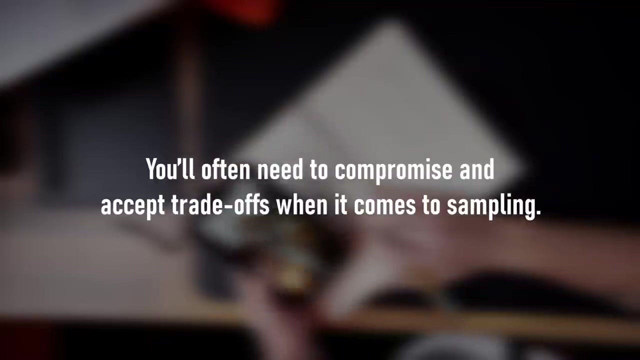 or referral-based methods. Importantly, you need to be ready for trade-offs. You won't always be able to utilize the perfect sampling method for your study, and that's okay. Much like all the other methodological choices you'll make as part of your study, you'll often need to compromise. 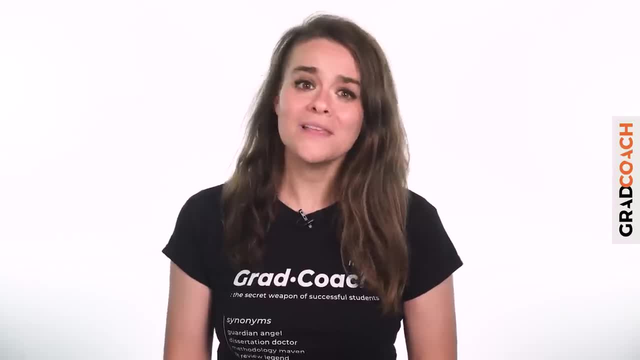 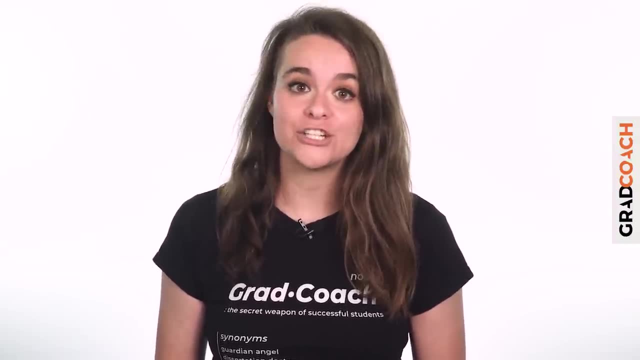 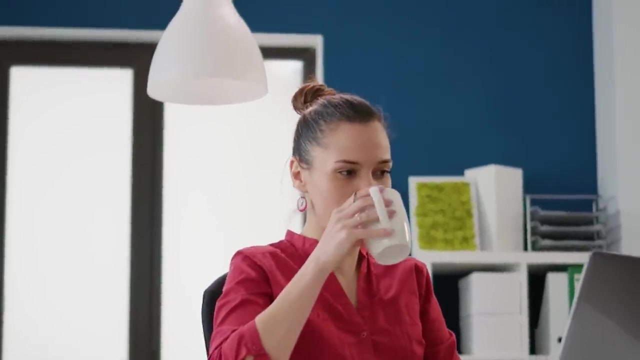 and accept trade-offs when it comes to sampling. Don't let this get you down, though. As long as your sampling choices are well explained and justified and the limitations of your approach are clearly articulated, you'll be on the right track. Every study has its limitations. 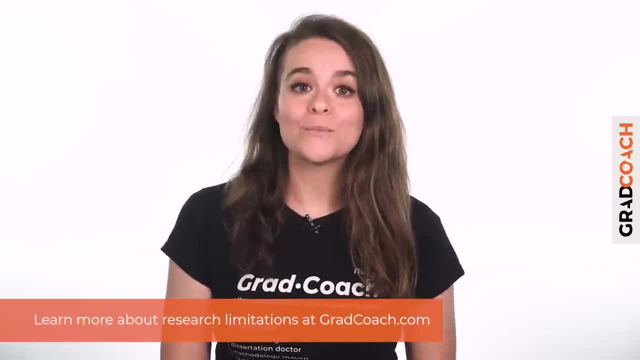 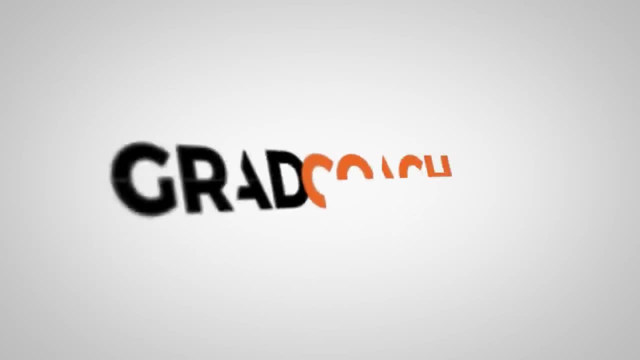 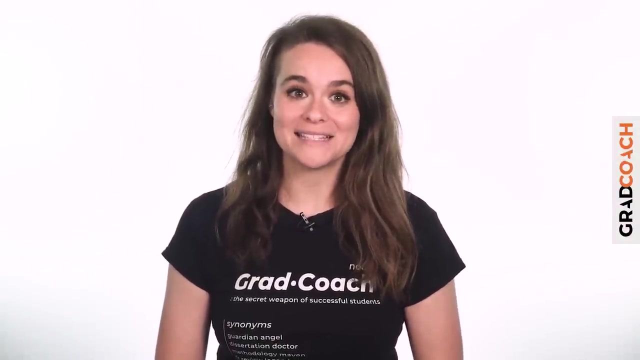 so don't try to hide yours. By the way, if you want to learn more about research limitations, we've got videos covering that too- Links in the description. All right, we've covered a lot of ground in this video. Let's quickly recap the key takeaways. 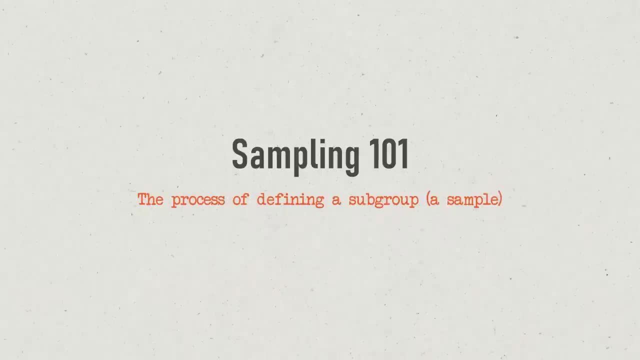 Sampling is the process of sampling. It's the process of defining a subgroup, a sample from the larger group of interest, the population. The two overarching approaches to sampling are probability sampling, random sampling and non-probability sampling- Popular probability-based sampling methods. 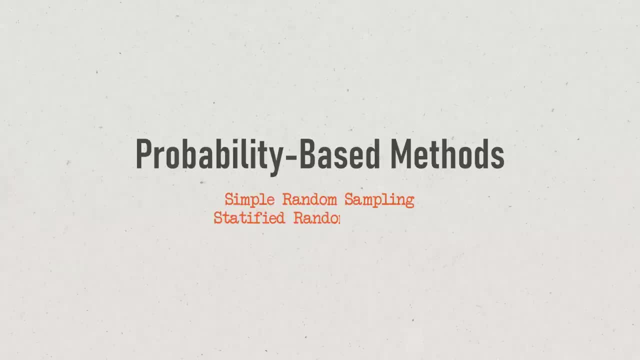 include simple random sampling, stratified random sampling and cluster sampling. Popular non-probability-based sampling methods include purposive sampling, convenient sampling and snowball sampling. When choosing a sampling method, you need to take into account your research aims. 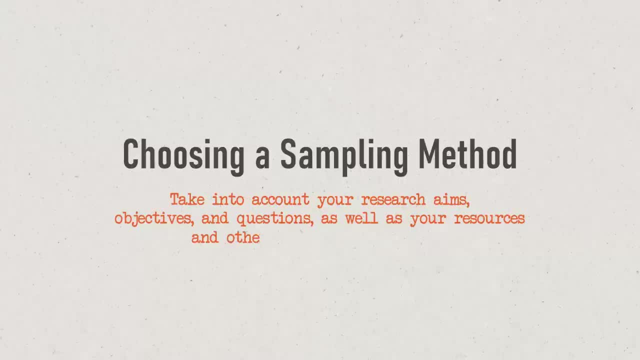 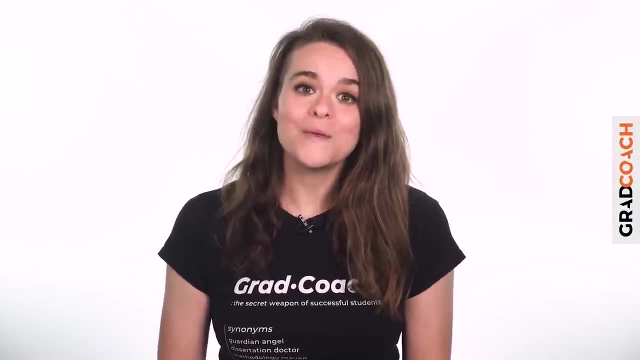 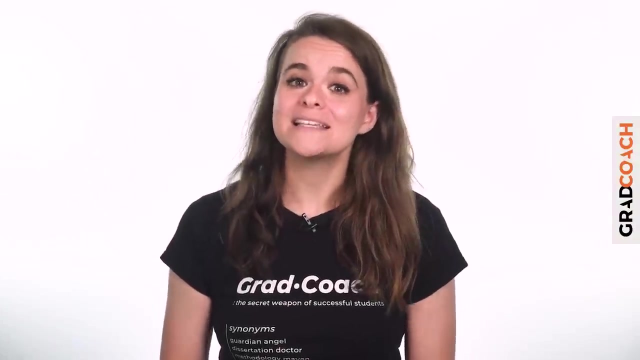 objectives and questions, as well as your resources and other practical constraints. Keep these points in mind as you plan your research and you'll be on the path to sampling success. If you got value from this video, please hit that like button to help more students. 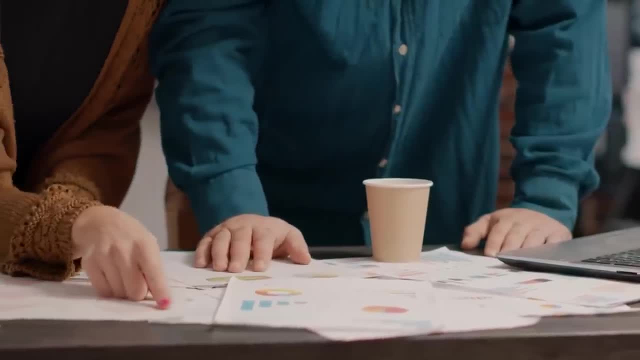 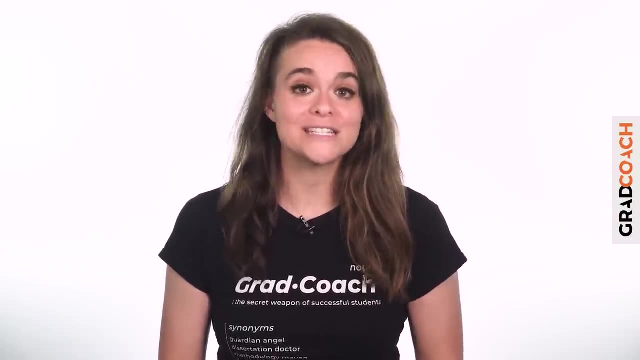 You will not always be able to utilize the perfect sampling method for your study, and that is okay. Much like all the other methodological choices you will make as part of your study, you will often need to compromise and accept trade-offs when it comes to sampling. 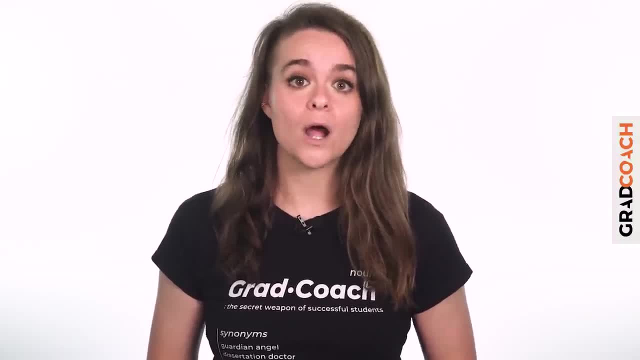 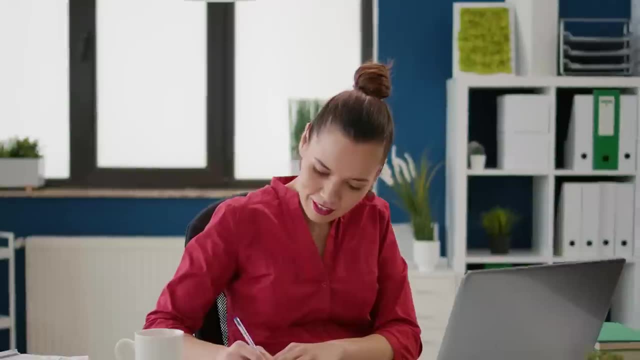 Do not let this get you down, though. As long as your sampling choices are well explained and justified and the limitations of your approach are clearly articulated, you will be on the right track. Every study has its limitations, so do not try to hide yours. 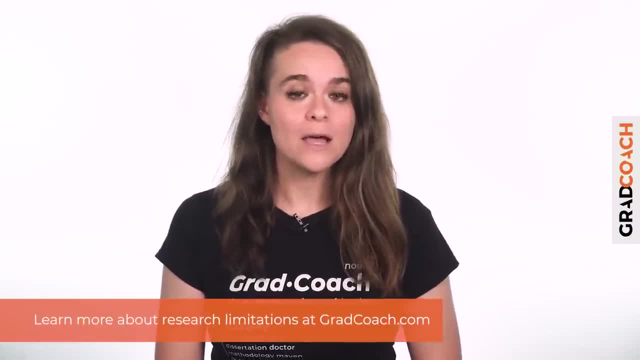 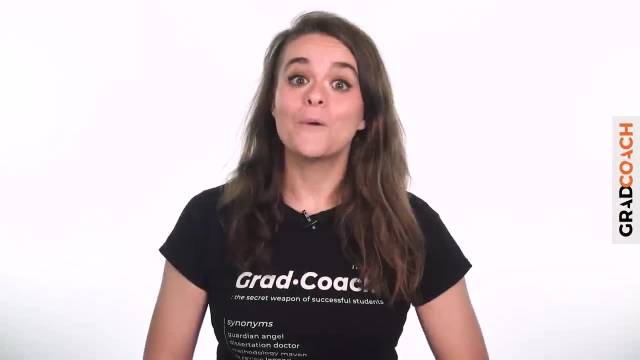 By the way, if you want to learn more about research limitations, we have got videos covering that too. Links in the description. Alright, we have covered a lot of ground in this video. Let us quickly recap the key takeaways: 1. Sampling is the purpose of your research. 2. Sampling is the purpose of your research. 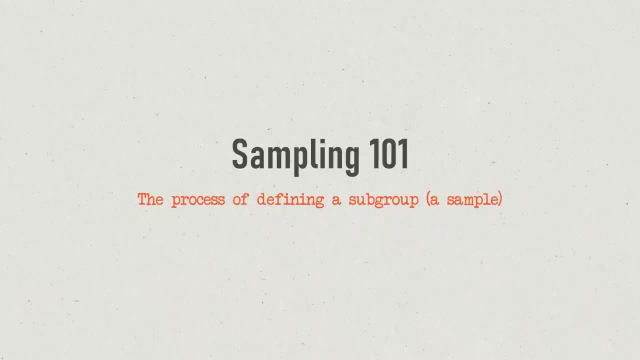 3. Sampling is the purpose of your research. 4. Sampling is the purpose of your research. 5. Sampling is the purpose of your research. 6. Sampling is the purpose of your research. 7. Sampling is the process of defining a subgroup, a sample. 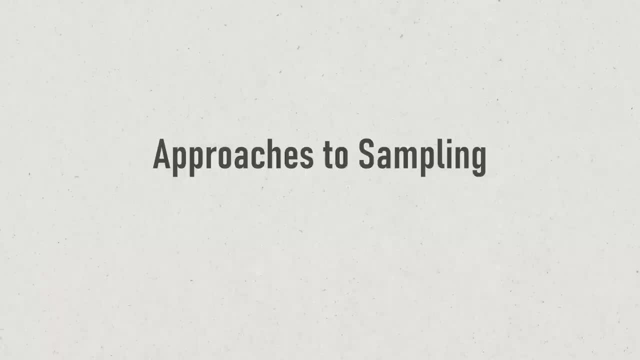 from the larger group of interest, the population. The two overarching approaches to sampling are probability sampling, random sampling and non-probability sampling. Popular probability-based sampling methods include simple random sampling, stratified random sampling and cluster sampling. Popular non-probability-based sampling methods include 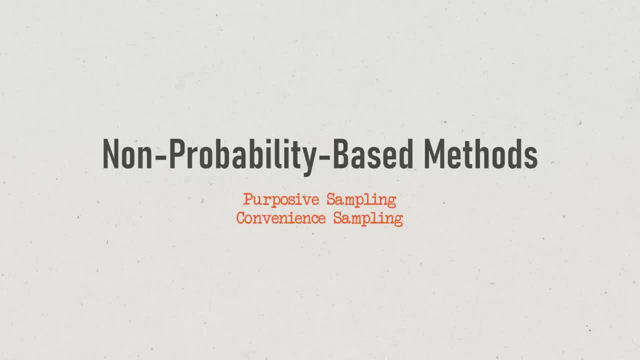 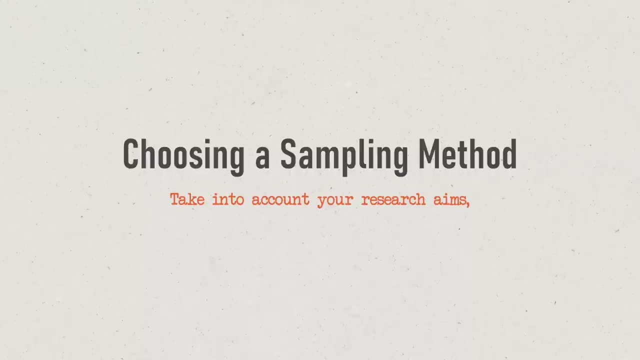 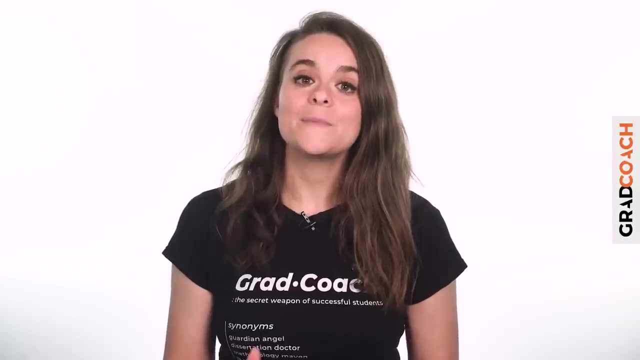 purposive sampling, convenient sampling and snowball sampling. When choosing a sampling method, you need to take into account your research aims, objectives and questions, as well as your resources and other practical constraints. Keep these points in mind as you plan your research and you will be on the path to sampling success. 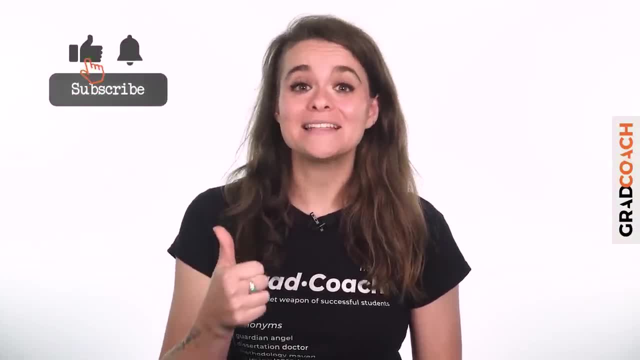 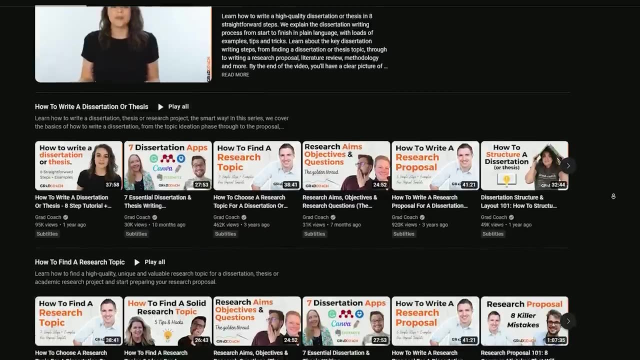 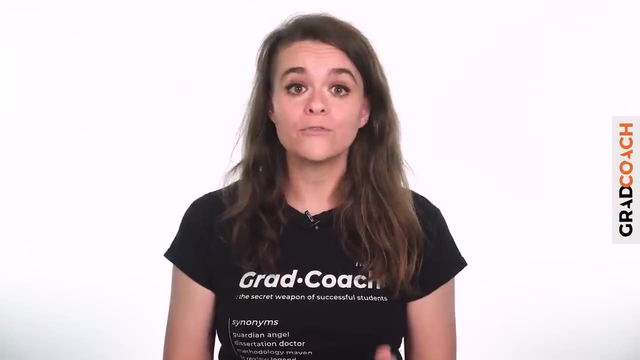 If you got value from this video, please hit that like button to help more students find this content. For more videos like this, check out the Grad Coach channel and subscribe for plain language, actionable research tips and advice every week. Also, if you are looking for one-on-one support with your dissertation, 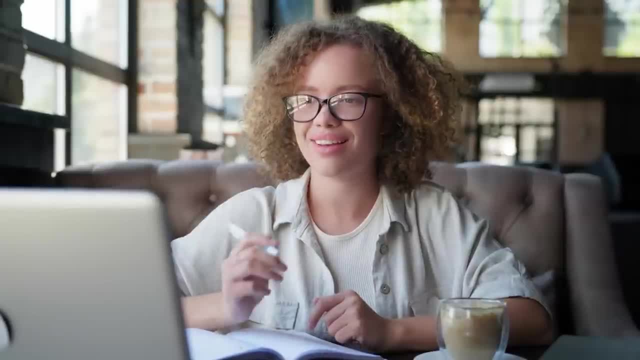 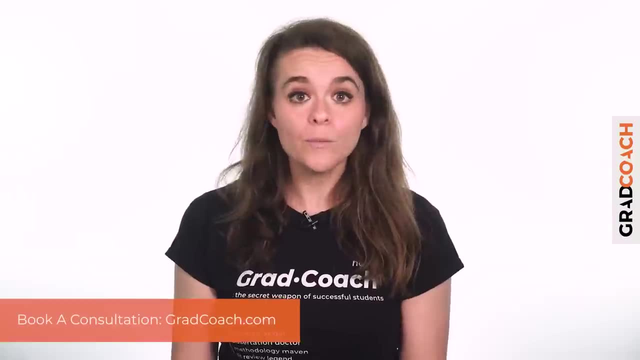 thesis or research project. be sure to check out our private coaching service, where we hold your hand throughout the research process, step by step. You can learn more about that and book a free initial consultation at gradcoachcom. 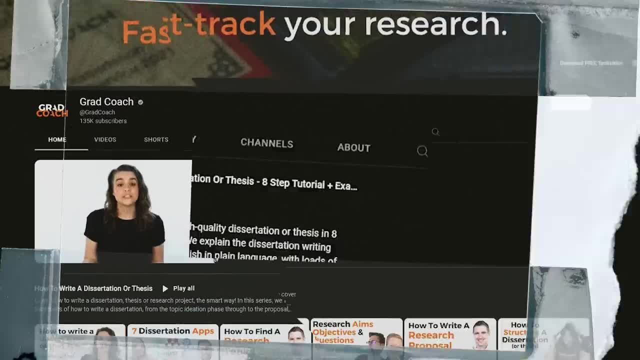 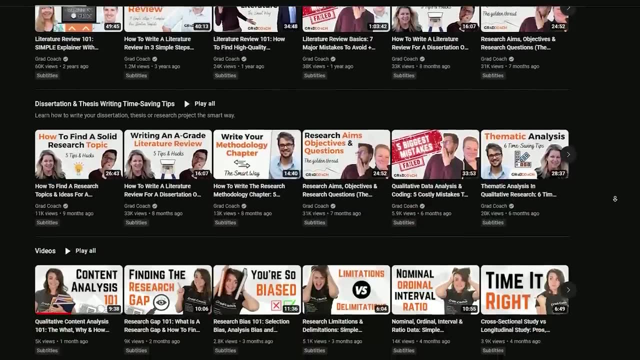 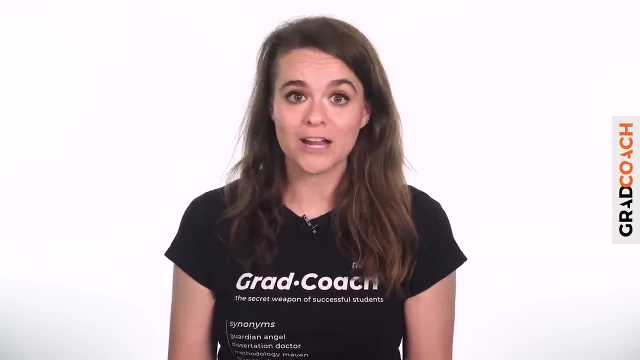 find this content. For more videos like this, check out the Grad Coach channel and subscribe for plain language, actionable research tips and advice every week. Also, if you're looking for one-on-one support with your dissertation, thesis or research project, 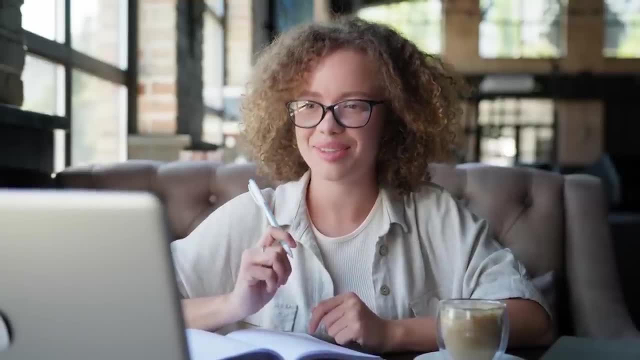 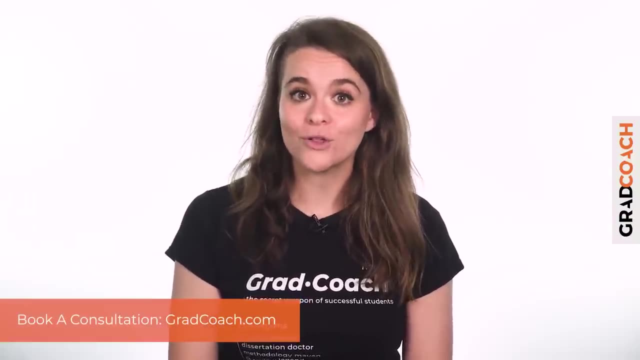 be sure to check out our private coaching service, where we hold your hand throughout the research process, step by step. You can learn more about that and book a free initial consultation at gradcoachcom. 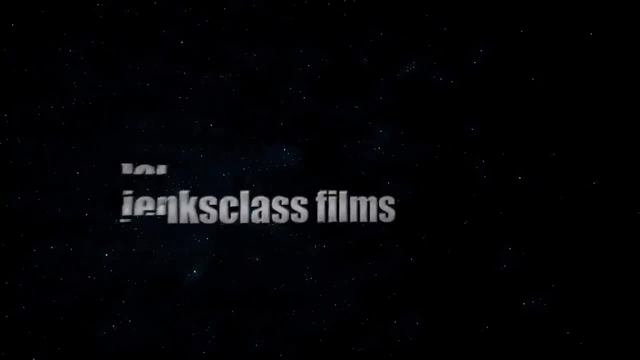 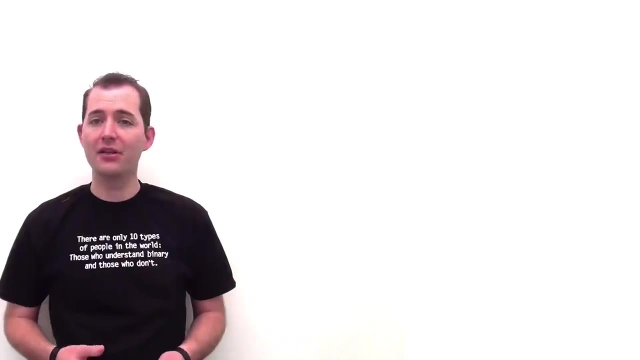 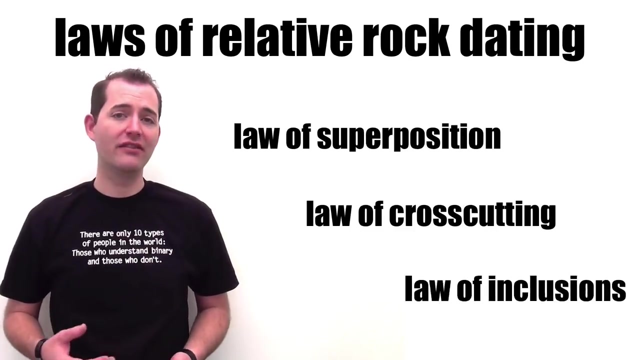 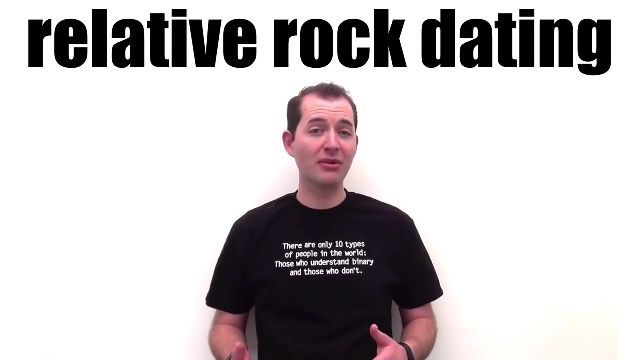 There are three basic laws of relative rock dating. They are the law of superposition, the law of crosscutting and the law of inclusions. First, let's define what we mean by relative rock dating. Relative rock dating is where we determine the relative or comparative age. 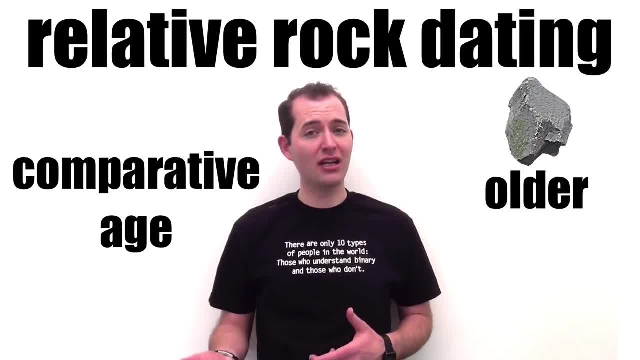 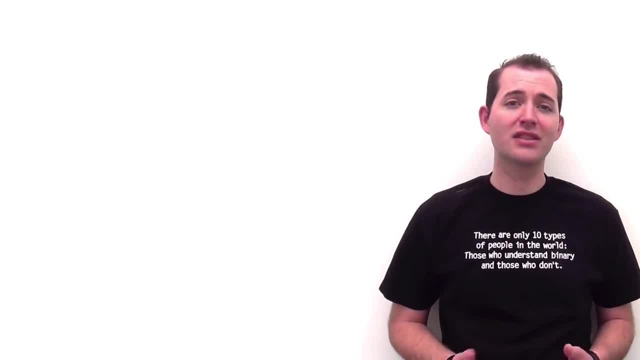 of rocks to each other. This means that we know which is older and which is younger, but we don't know exactly how old they are. Determining an exact age of a rock is what's known as absolute or radiometric rock dating. We use relative rock dating laws to determine. 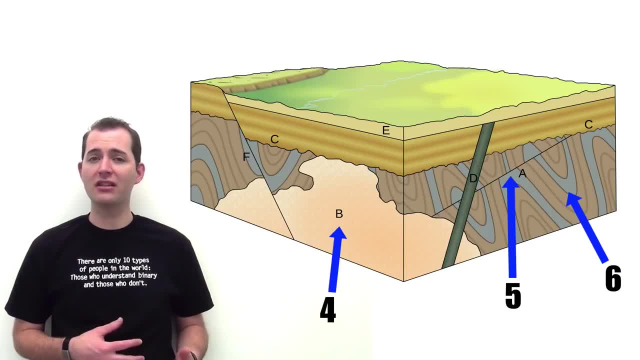 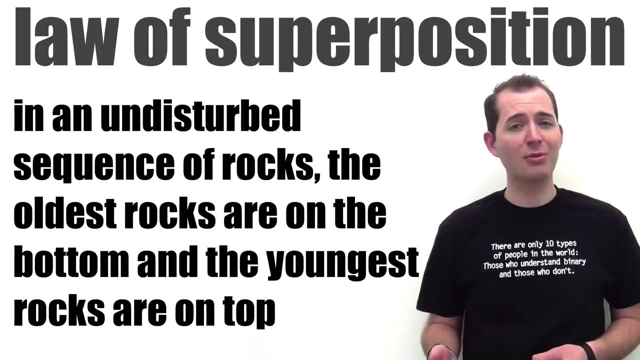 the relative ages of rock layers or features to each other. Again, we're only able to determine what is older and what is younger. Let's look at each of these three laws. The first is the law of superposition. The law of superposition states that in an undisturbed sequence of 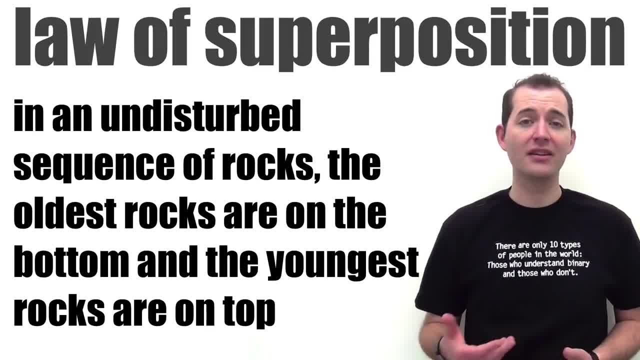 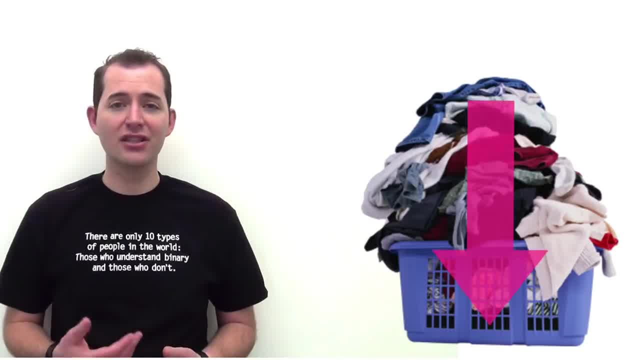 rocks. the oldest rocks are on the bottom and the youngest rocks are on top. We can compare this to an analogy of a laundry basket. Each day, as you add dirty clothes to that laundry hamper, the layers stack one on top of the other, And as long as this stack is,